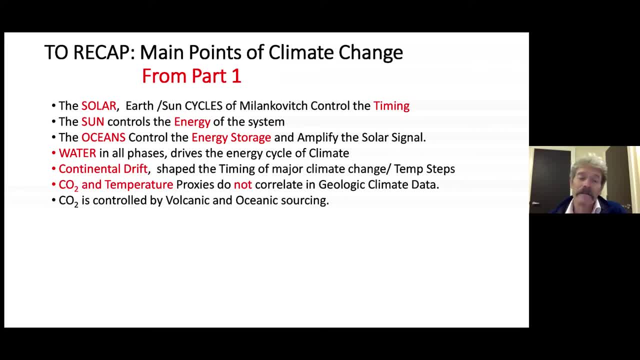 acceleration of CO2 and temperature. We concluded from all of this detail: fossil evidence and data on CO2 and temperature do not correlate. CO2 is controlled by volcanic and oceanic sourcing, and temperature is being controlled by the sun, the oceans and the continents drifting. 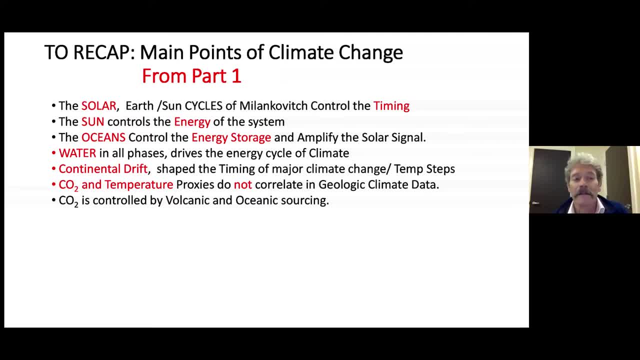 creating open or closed continental areas, oceanic areas- excuse me, The default condition that we are in now is cold, dry, dusty and glacial. What has happened in the past where we had very warm periods, like the Eocene, where it was warm, wet and non-glacial? No, 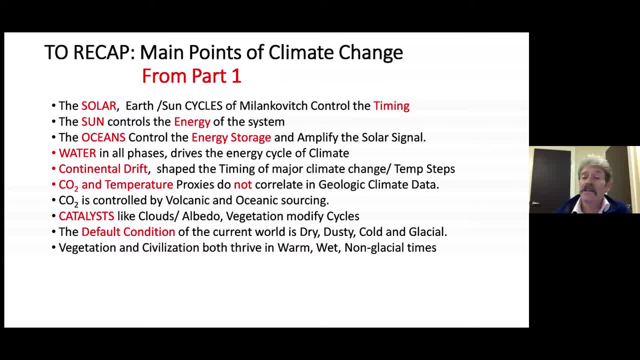 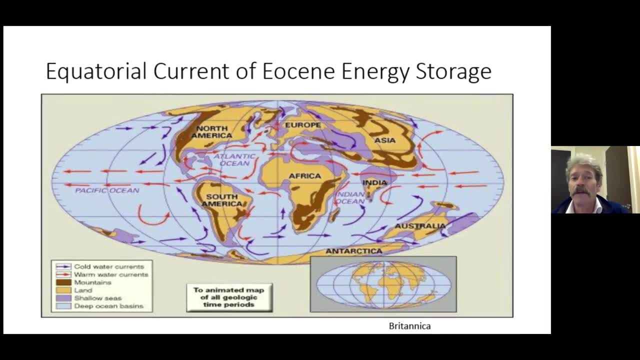 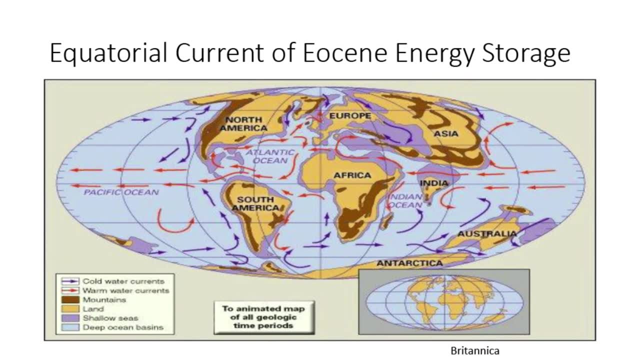 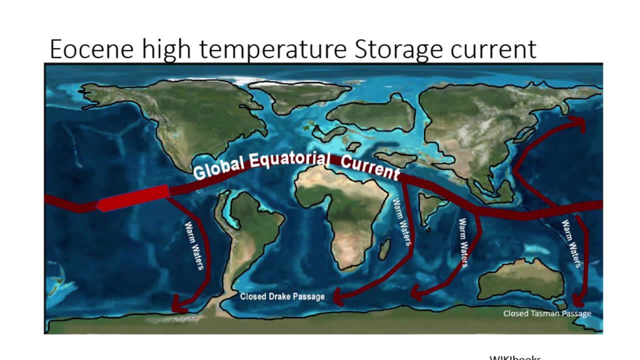 glaciers existed. Vegetation and civilization prospered during those warmer wetter times. This is a picture that we used last time to illustrate the circumpolar and the circum equatorial current systems that existed during the Eocene. This is a simplified version thereof. 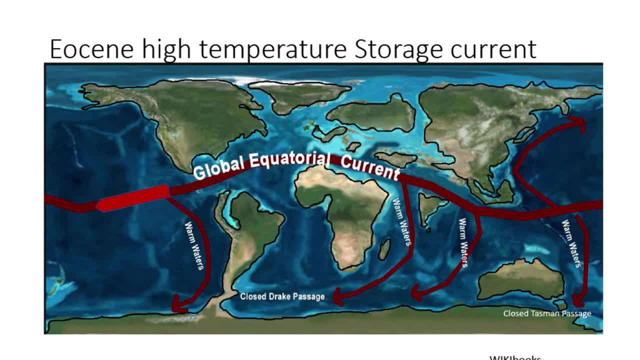 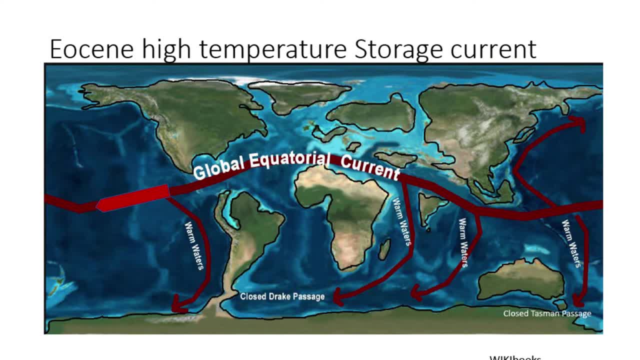 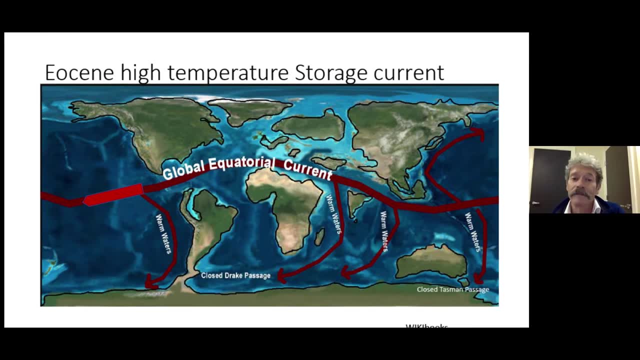 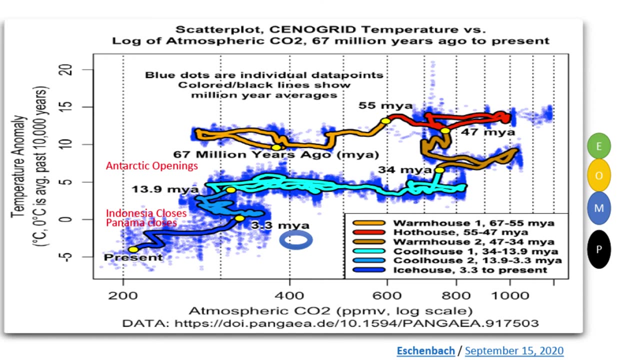 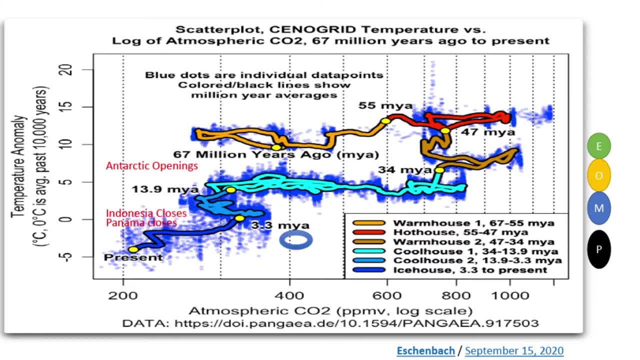 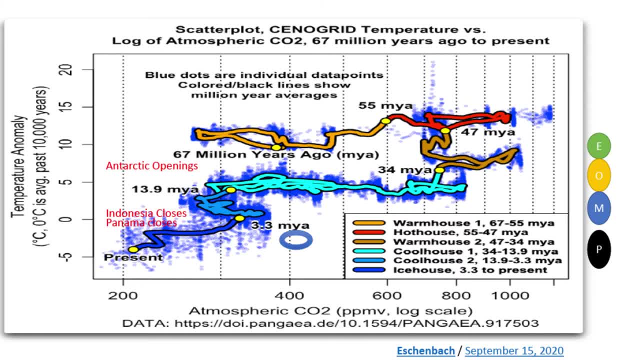 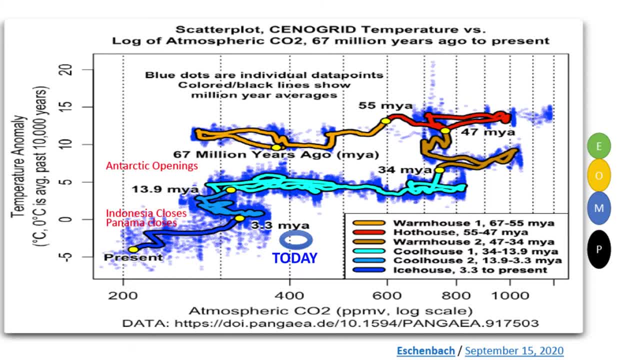 where we are today, from 67 million years ago. This graph is of the past- fossil temperature and CO2, and it is in strong agreement with steps, not necessarily any kind of continuum between those two end members. So the temperature corresponding to the major openings and closings is the important take home. 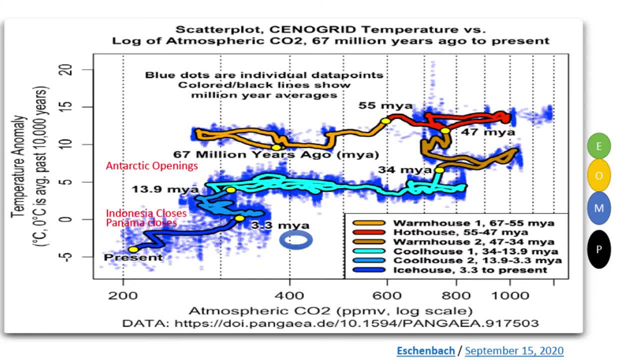 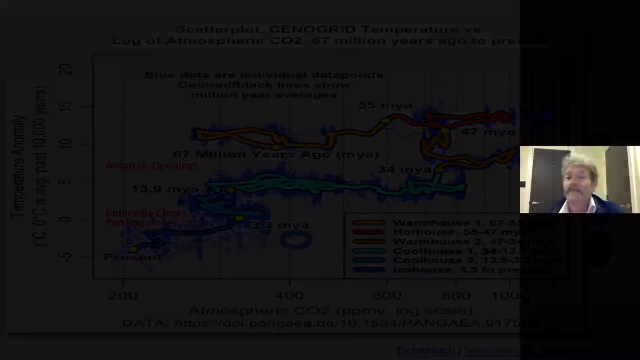 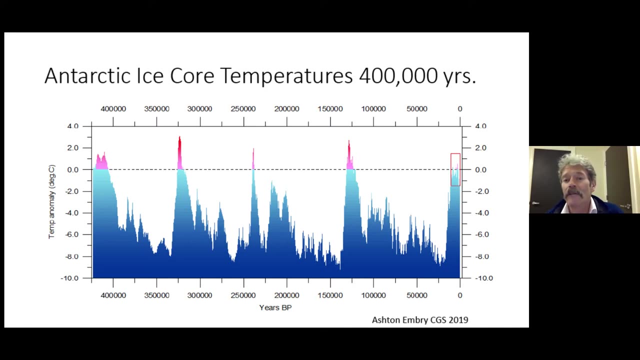 message and solar energy and ocean current storage of that energy governs the temperature. The greenhouse gas theory and CO2 are completely absent from this view of history. The Antarctic Core and temperature data in this illustration are made from oxygen isotope work. 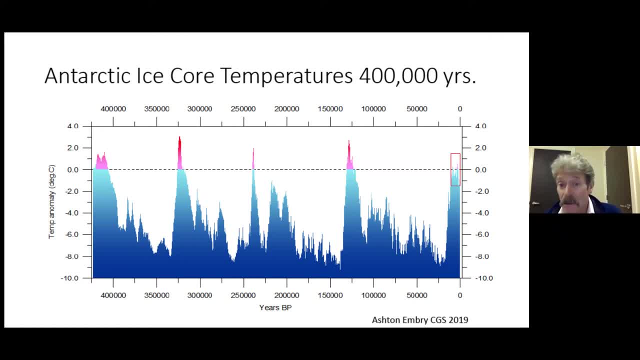 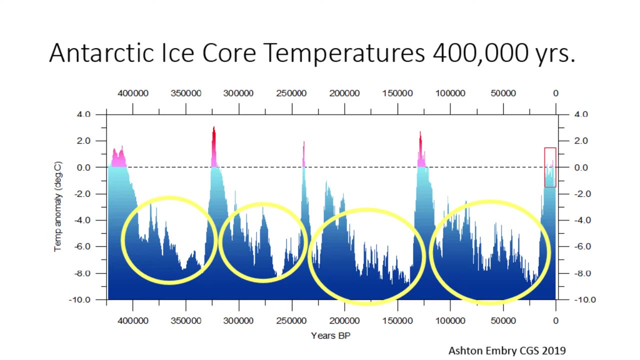 and show the thermal history of the past 400,000 years, As reviewed in part one. the warm peaks are times of earth sun system coincidence where warming could take place. These, the lows, are where 100,000 year long periods of cold took place because of the Milankovitch cycle. 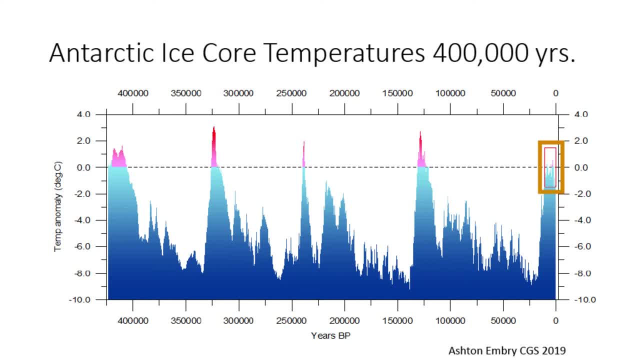 The last period of time- the Holocene- here, 11,000 years of earth history. the last 11,000 years of earth history is where we want to focus now. We're in that last little peak and we should prepare for something to be cooling after that. 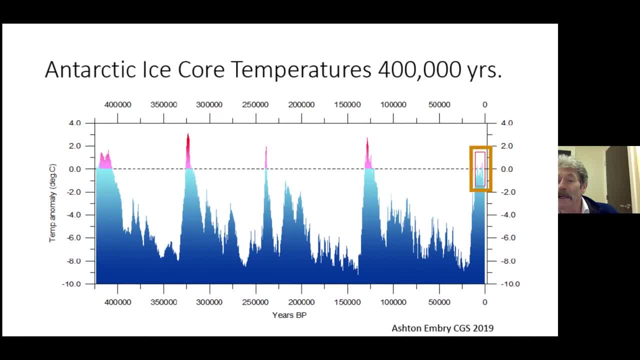 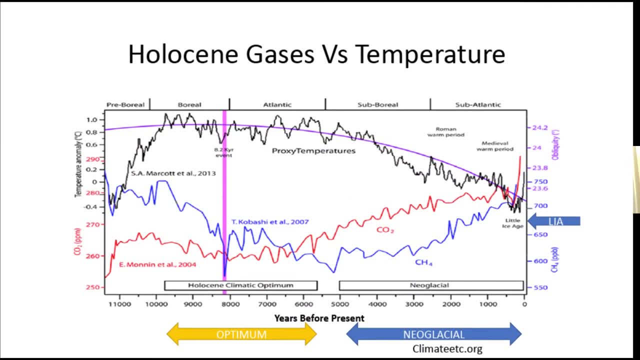 In this red box we'll do a lot of expanding and explaining of what's happening in the current period of time. This is a blow up of that 11,000 year period. The arc of proxy temperatures in the Holocene period is magnified here in the black jagged line. 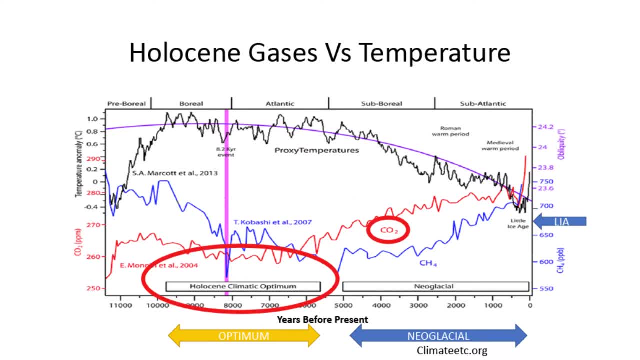 Note that during the warmest part, the climate optimum, the CO2 is lowest. not at all, as theory would predict. It's very low CO2, high temperature. The purple arc is the tilt of the earth on its axis. It's obliquity. 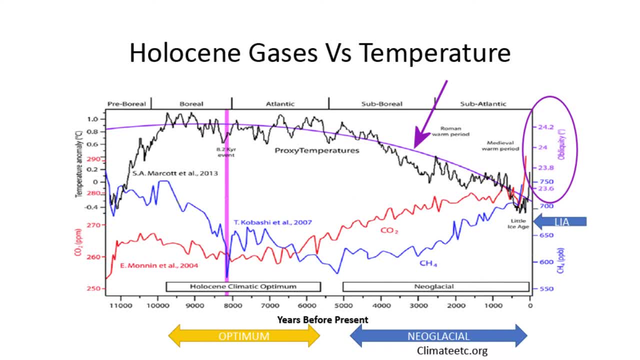 The temperatures were highest when the axial tilt of the earth and the sun was 24.3 degrees at the top, And now we are 23.5 degrees. Carbon dioxide and methane, both plotted here, do not track the temperature and actually are anti-correlative with temperature. 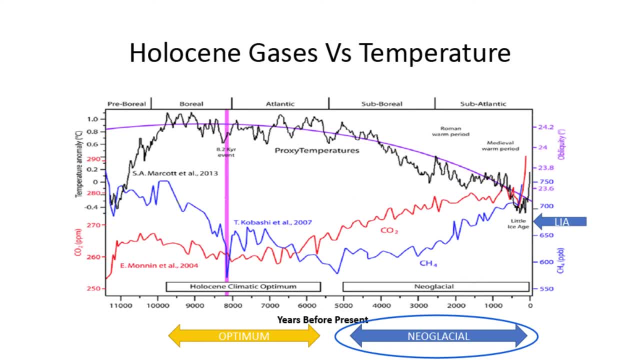 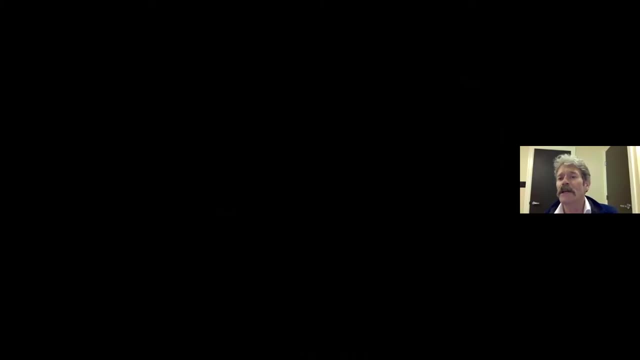 during the last 11,000 years. We are now in the period called the neoglacial part of the cooling Holocene that we have just come through, And the coldest part was the little ice age. here, The Holocene reconstruction of solar activity. 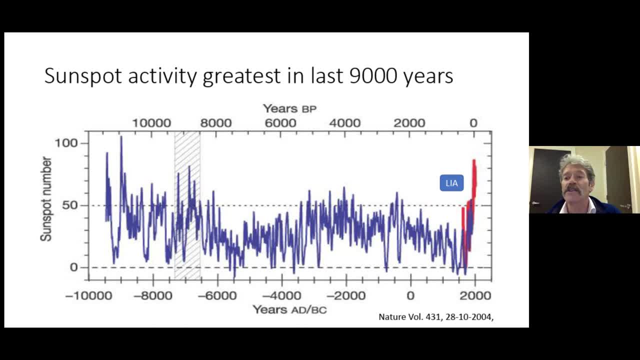 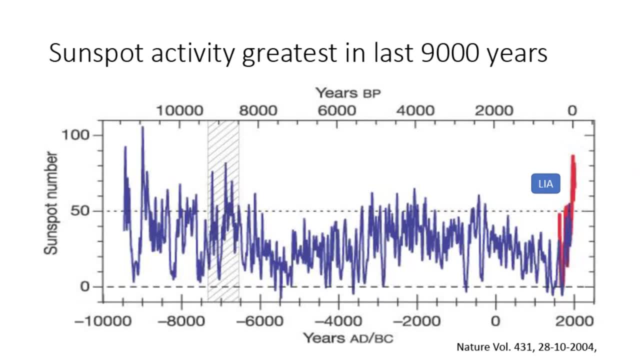 based on beryllium-10 records and carbon-14 records shows that the solar activity has recently recovered to above normal after dipping during the little ice age shown here. We are returning to a higher point. we have been in much higher solar activity periods. 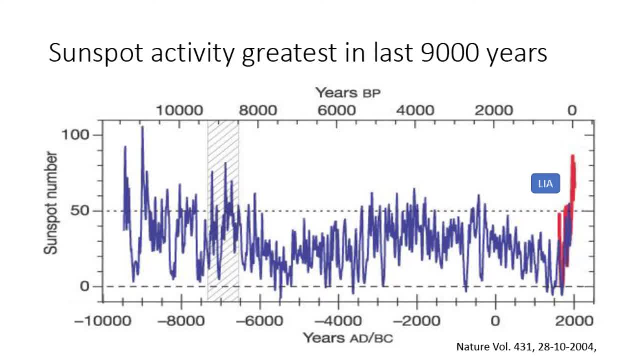 The early Holocene maxima warm period shows very similar high solar activity. The only driver that can create earth system energy is the sun. These solar indicators of fossil solar activity show significant variability. The only way to retain and store the energy from the sun. 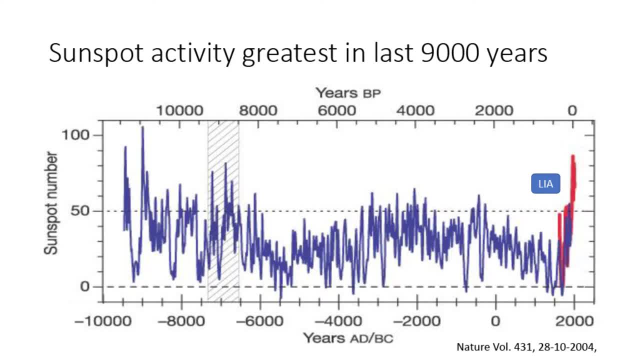 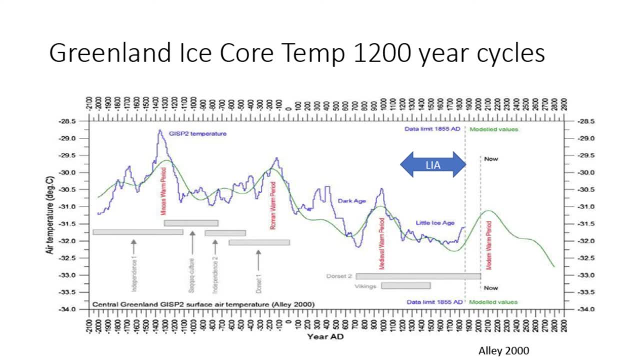 is to drive it through the water cycle. This is a blow-up, once again, only this time- of only the last 4,000 years of human history. this time- And we're dealing with Northern Hemisphere, Greenland, ice core- We're seeming to get a pattern, a cycle cyclicity to this. 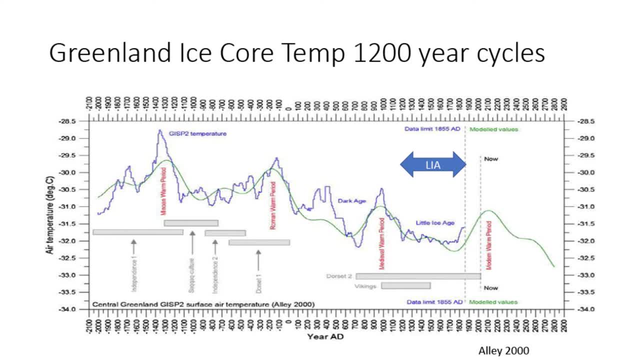 The green line is showing you that And the blue line is the temperatures as per the ice core, We appear to have a rhythmic and steady decline, a declining temperature. So we're declining through the whole period And we are now, as I mentioned, in the neoglacial. 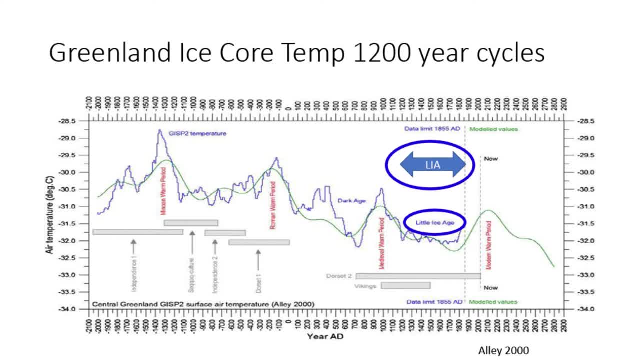 So we're moving into this and we have the little ice age period here. Period covered is very historic and shows that dynasties succeeded during the warm periods of human history: the Minoan, the Roman, the medieval, the modern periods. 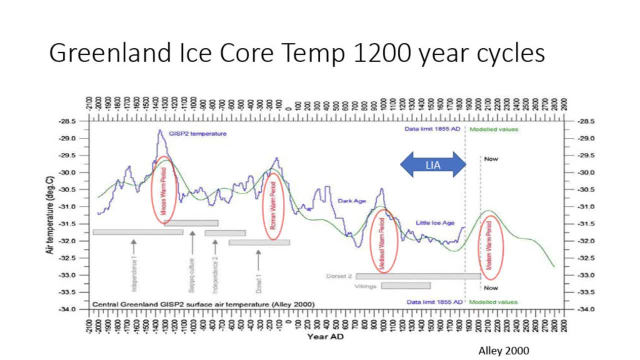 But there are cold, dark and difficult times in between these good times: the dark ages, the little ice age, et cetera. We have just recovered from the last low of the little ice age, which generated four to 600 years of glacial advances. 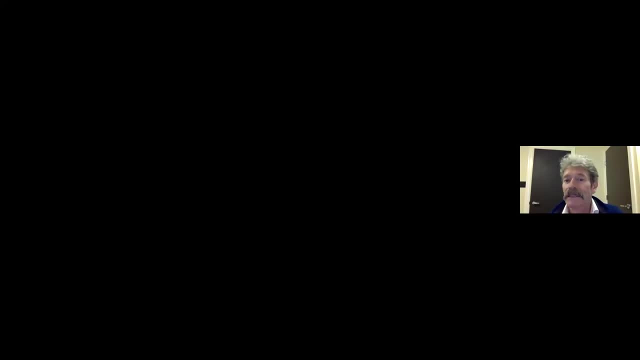 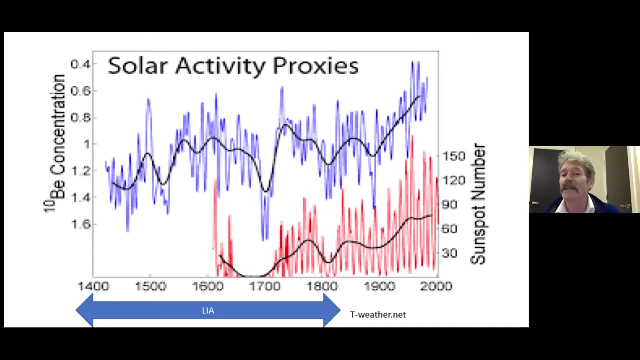 The trend of temperatures is down for the whole period. This is a blow-up of the last few years of this solar activity based on beryllium 10 anomalies lowest during the little ice age and growing And growing toward the modern climate warm period. 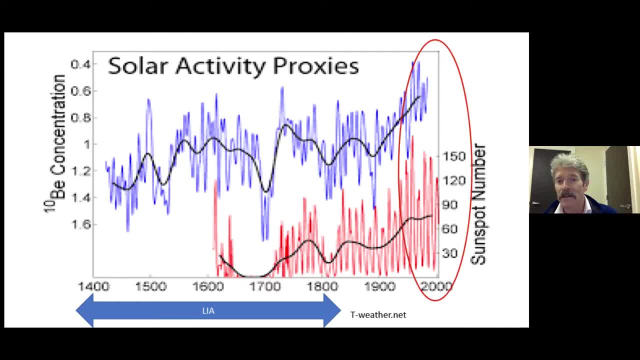 The sun is very active now in this area. It was very dormant through the little ice age and has very few sunspots compared to the cycles of today. Each solar cycle in red is 11 to 12 years between peak and trough The lower cycles. 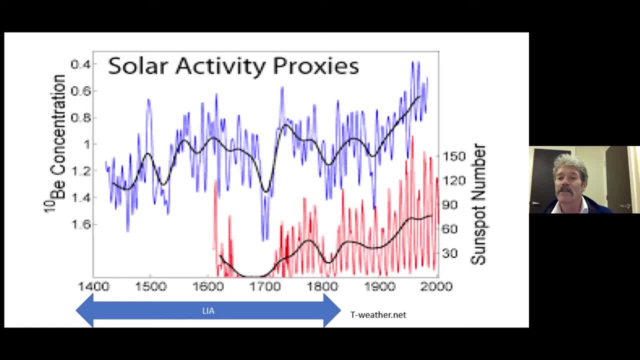 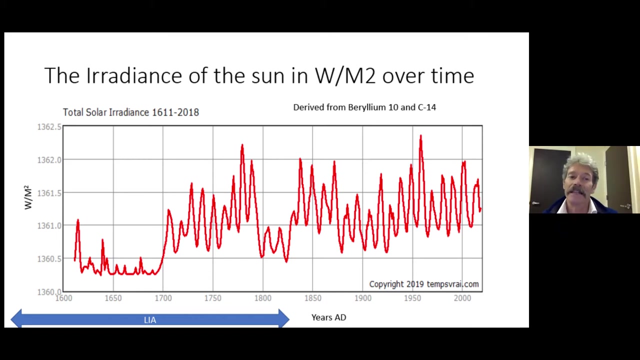 when the solar intensity and sunspots drop near zero, are those areas of cold And the temperature falls. what we have are periods of ice age, In this particular case, accumulation of glacial ice. Here's another view of that: solar activity data. 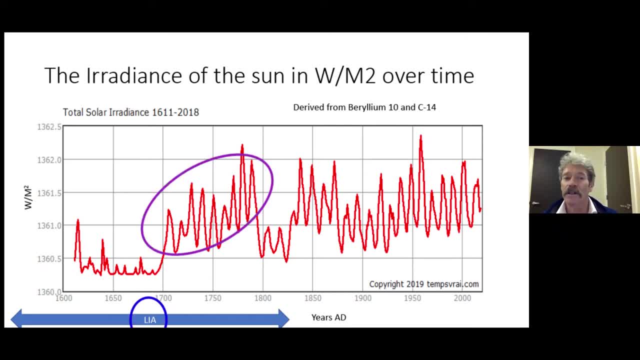 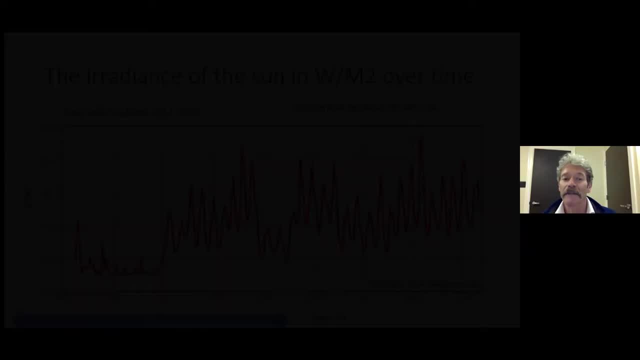 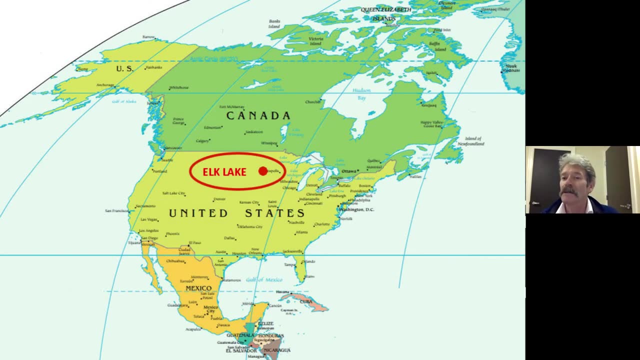 the little ice age period here, extending right through to this portion, with a small uh aberration here of energy, and then continuing to climb to today. Let's look at some lake core Now. this would be coring from a lake in Minnesota. 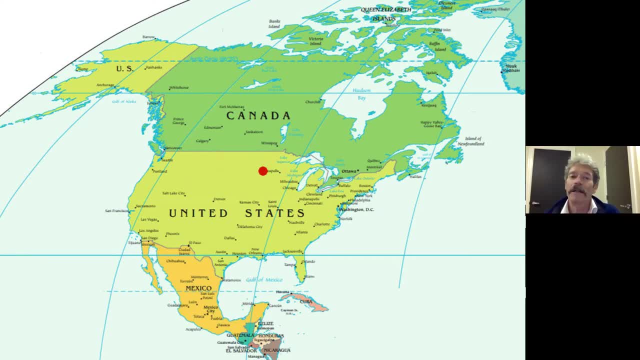 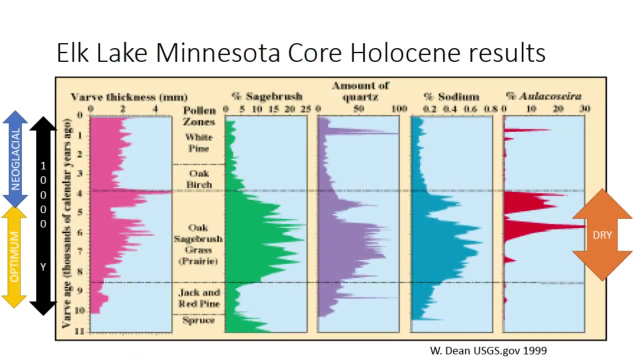 called Elk Lake. It's a place at the meeting point of three major climatic zones in North America: The Pacific, the Arctic and the Gulf of Mexico. They all influence this area. They all influence this area In these cores. we see the thickness here represented as years of age. 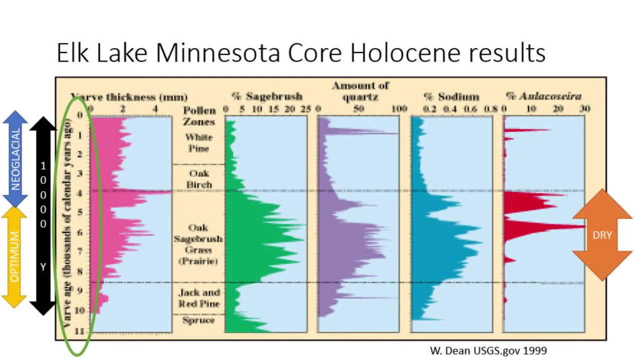 of the core 11,000, the beginning of the Holocene up to today, modern. We look at the types of materials that are within those cores, from pollen of trees, from sagebrush, et cetera, which were found in those areas. 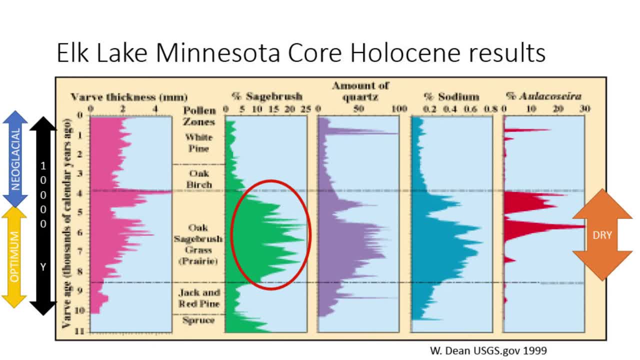 Sagebrush is blooming here, Quartz- this would be sand deposited- is here and a sodium concentrations here. This is a dry period of time. This is a little bit different. Why such a dry period? This is also a part of that optimum period. 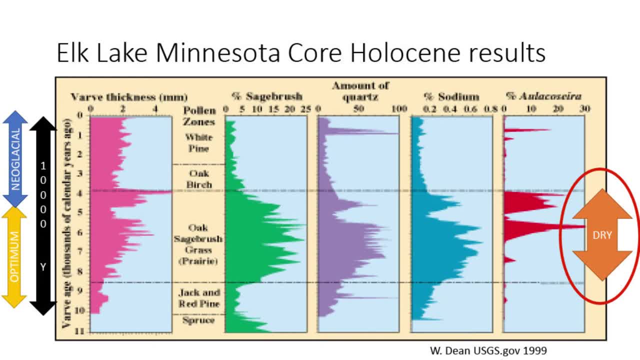 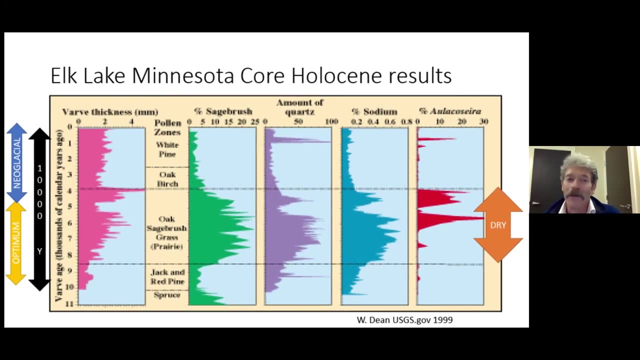 We are in the neoglacial. We've come out of it and moved into a different period, So optimum conditions aren't the same everywhere, All places. what you might view as optimum in this situation, when you're in dry and dusty, might not be what you really want. 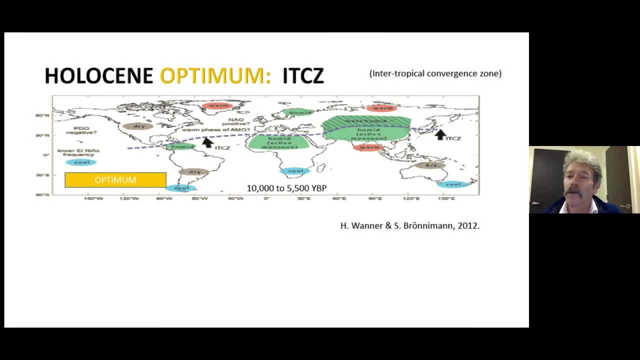 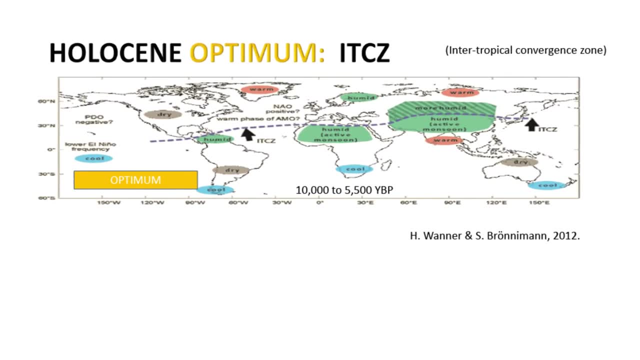 But here's a summary. This is what the globe looked like in the Holocene optimum, 10,000 to 5,500 years ago, where the climates were very different than they are today. There was drying of Elk Lake in Central North America. 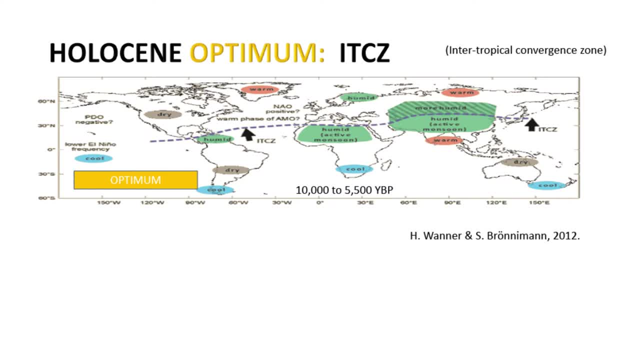 There were humid monsoons that dominated what we now think of as large deserts in Africa and in Southeast Asia. The position of this line, the ITCZ, the inter-tropical conversion zone, is shown on the map and it shifts to the north. 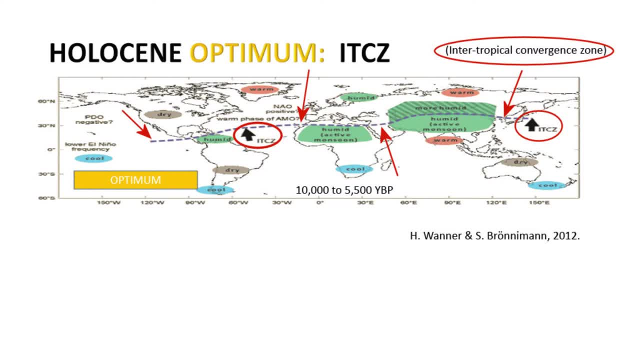 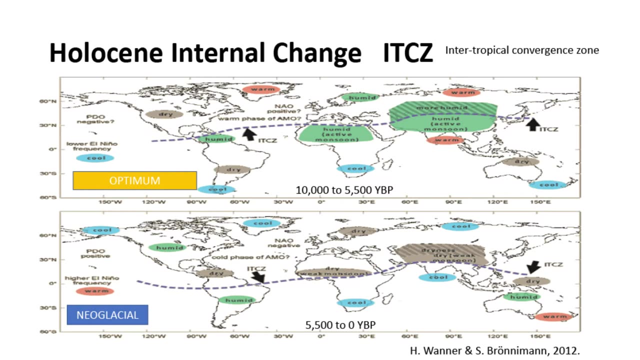 And we'll see it later on. to the south, This is the zone of convergence of upper level winds and lower level tropical winds on the earth. This is what it looked like in the neoglacier does in the neoglacial, where we are now. 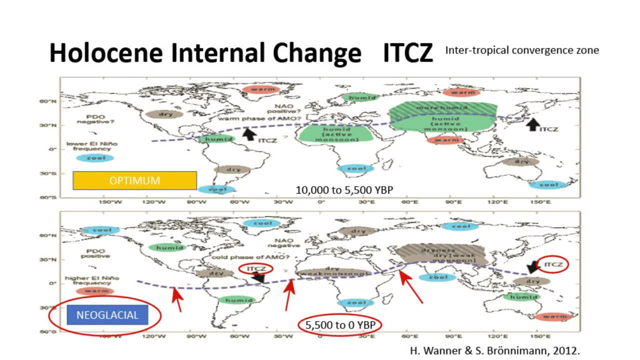 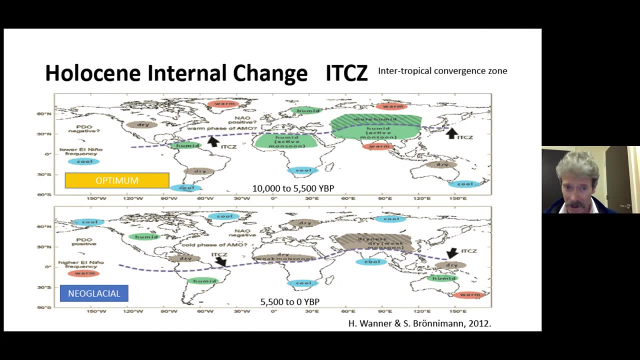 The ITCZ has moved south. Dry has been replaced by humid in Central North America. These are the kinds of changes that takes place over 11,000 years of climate variation within what we see as the warm period that we're in right now. 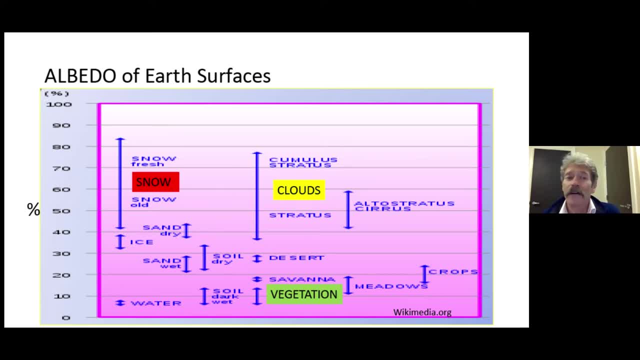 On this slide we're showing something called albedo. Albedo is a reflectivity off of the surfaces and the materials on the earth's surface. What we're seeing here are forests and vegetation that have low albedo- And water does too, but water is the lowest. 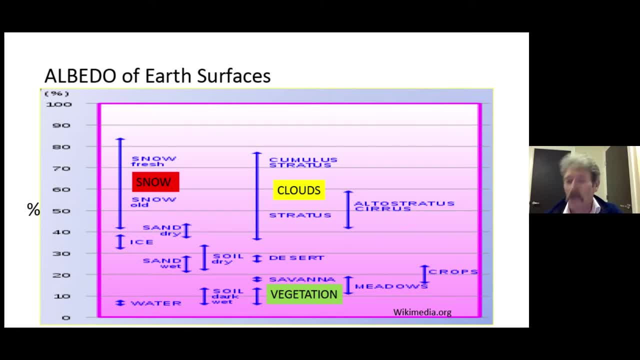 It's very important that we concentrate on that Highest absorption of water, of energy within the water. The most notable thing in this diagram is the water, And what we need to do is think of it as the greatest absorber of solar radiation energy. 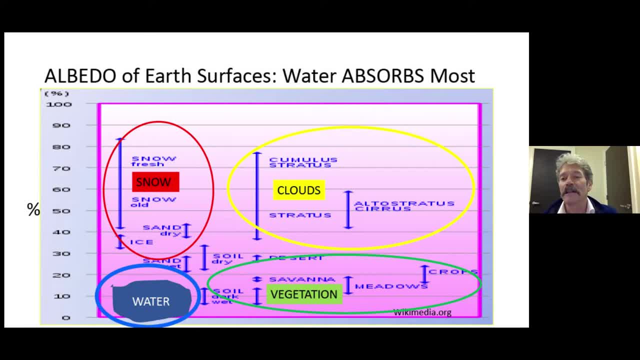 especially of the high energy bands of radiation in the ultraviolet, The shortest wavelengths of solar radiation. This is the major reason why solar and water systems drive climate. It's the absorption by something that covers more than 70% of the earth's surface. 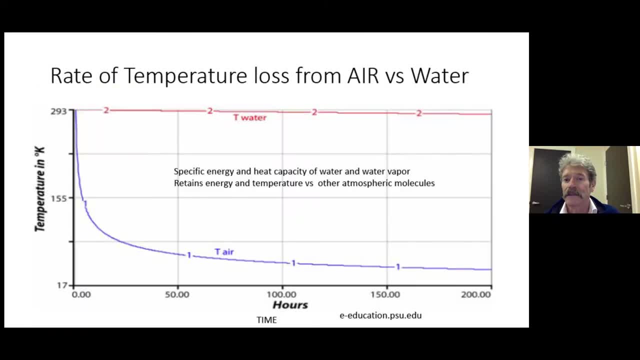 The water that makes all the difference. Why is it so different Water versus air? This would be the cooling rate that you would experience from those two equal amounts, And this is the lower energy. waves is what we're talking about in terms of the inability of air and atmosphere to make. 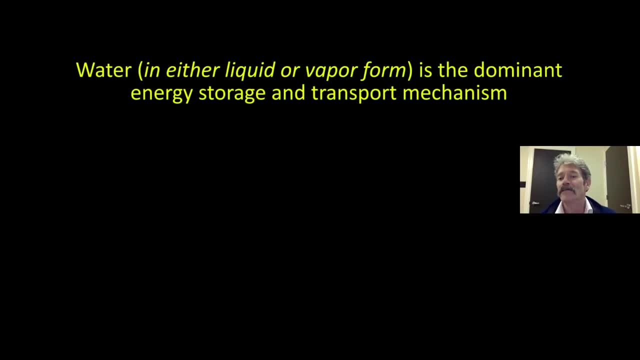 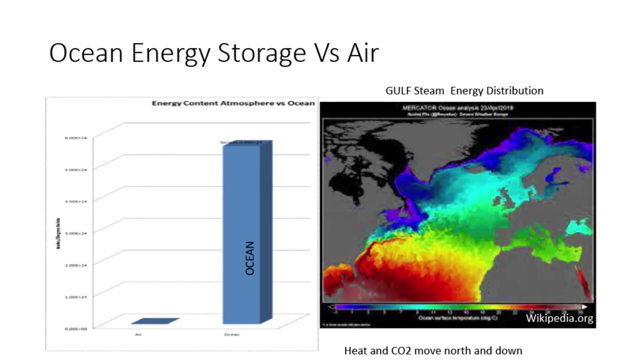 the whole difference. Energy in the form of water and water vapor are what we really want to stress now. Energy storage systems are so strikingly different between air and the ocean that it's hardly even possible to illustrate them at all, But what we do know is the Gulf Stream distribution. 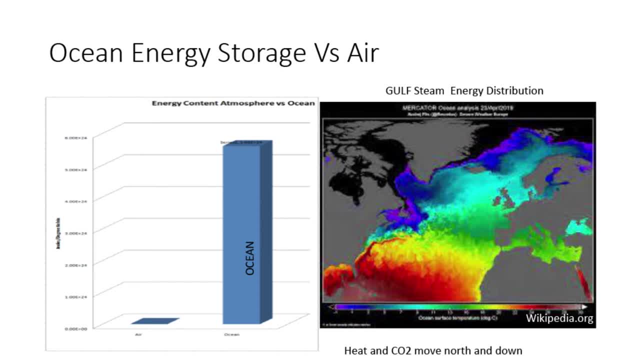 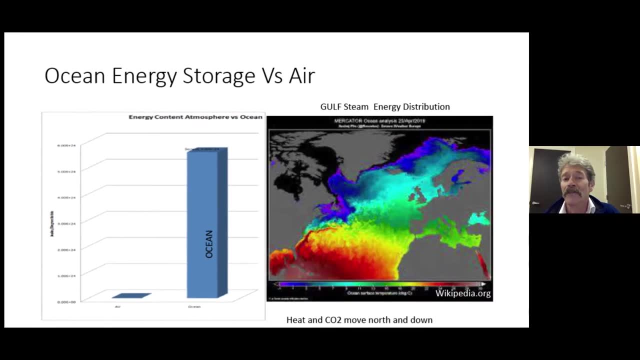 system shown here on the right is the reason why Europe remains so warm, even though it is at a latitude of northern Canada or northern Russia. It's basking in the glow of the retained energy of the ocean system, the Gulf Stream, In a polar vortex dominated. 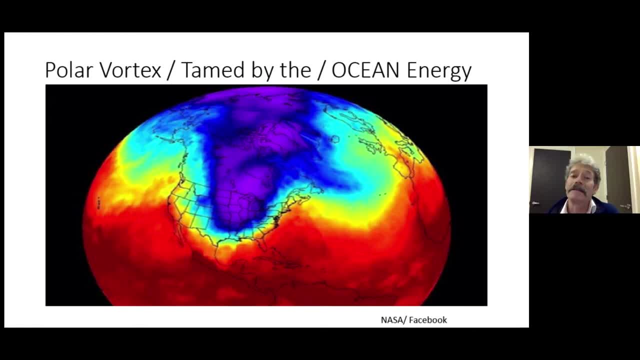 North American winter we look like this. This is the cold polar vortex: extremely cold, negative 30 to negative 50 in this area, And the temperature is very obviously being shielded and modified by the oceans which surround us. So the role of the ocean and heat storage and climate. 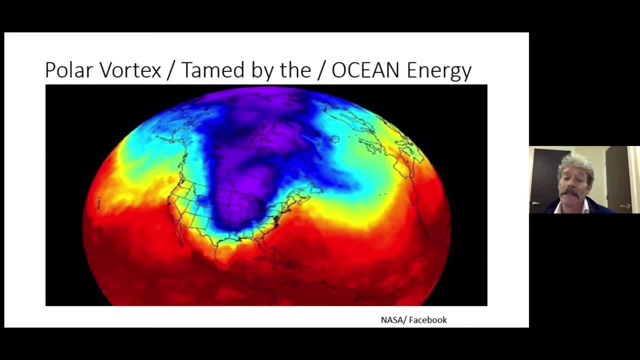 is just now, however, starting to be properly documented. Climate models have still not properly realized the storage and redistribution of energy from this climate weather driver. Very few can claim to understand and document the real changes due to the oceans at all their depth levels. The planet of the past had many large, continuous heat accumulating. 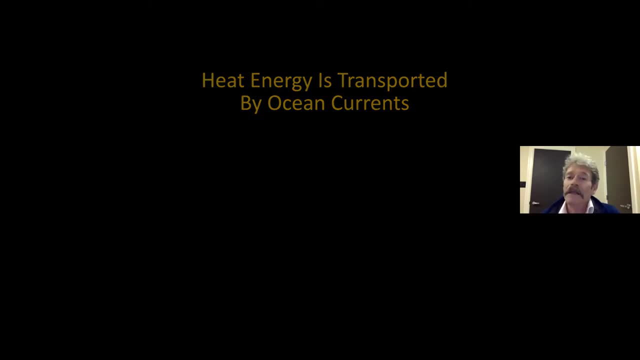 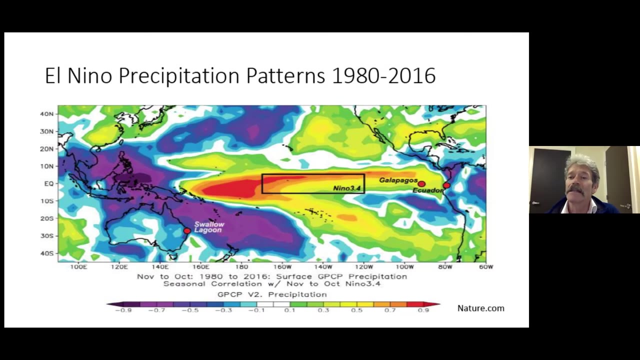 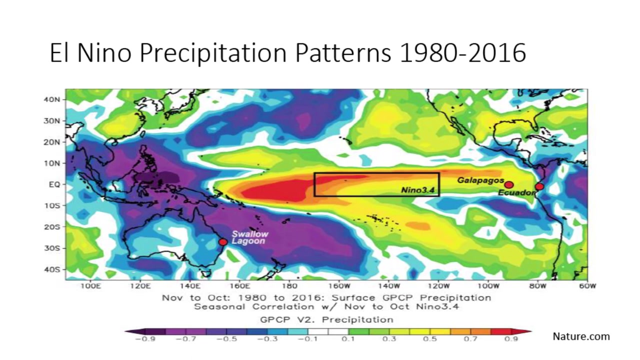 ocean currents, as we remember from part one. Today we have some of these large climate creators still around. The most significant is the oscillating El Niño-La Niña system of the tropical Pacific Ocean. They call it the ENSEO. The map shows the most recent precipitation results from El Niño here. 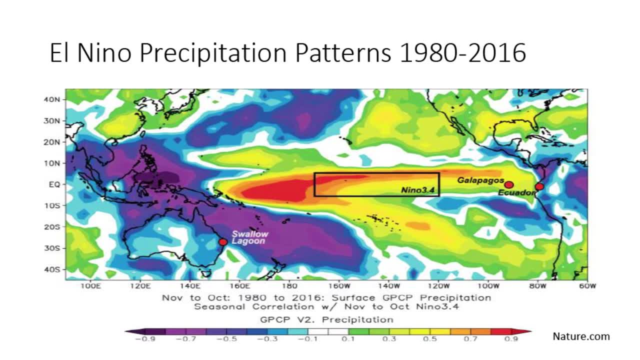 in the El Niño 3.4 region. The Pacific has entered a drier, cooler, La Niña phase now in 2021.. If you like this video, put a like or leave a comment and give us a comment below. If you need help with a video call or comment below, please feel free to contact us via the email. 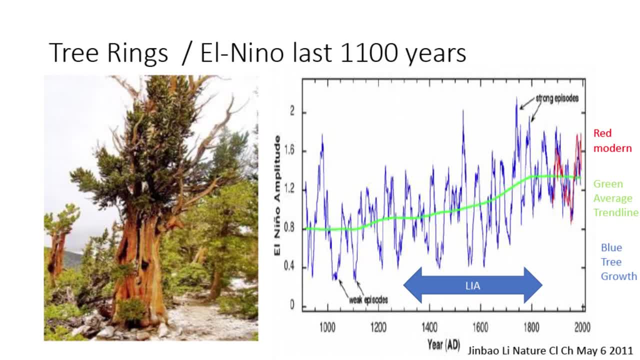 services that we have at the moment. We're also ready to cover a huge amount of engineering and AI within our team at El Niño. For this segment, we're going to kick off our new mission in the own small possible way, and that is to keep you informed, and informed of our next game. 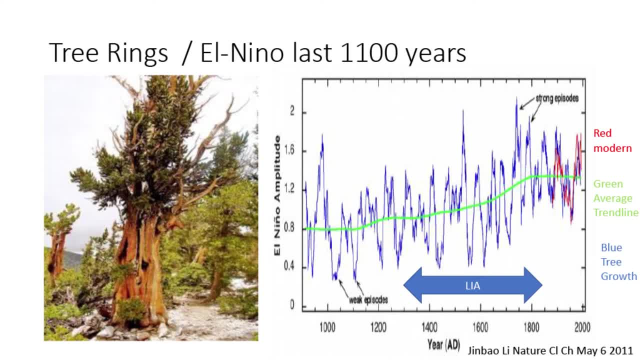 If you would like to be informed about any of the events that we have this year, please do so via our web site at wwwelniñoca. Thank you so much for tuning back in with us today. We'll see you again next time. 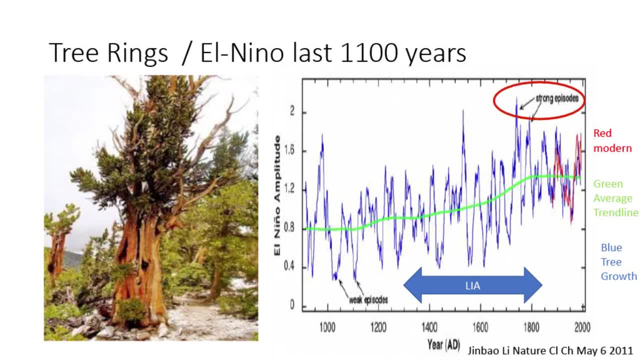 Have a great weekend. Stay safe and healthy. Take care. Stay, keeping yourself safe. people Will see you next week on the show Ice Age here. And these strong episodes are followed by weak ones. El Niño, La Niña A. 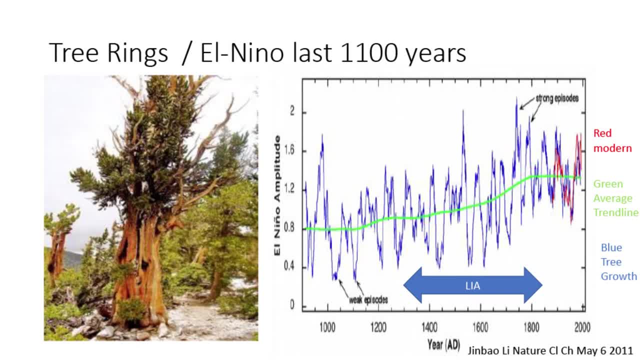 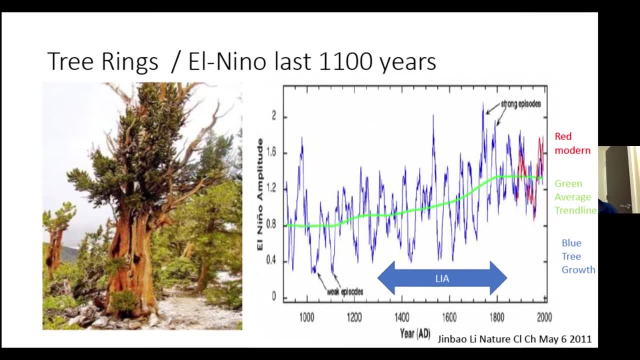 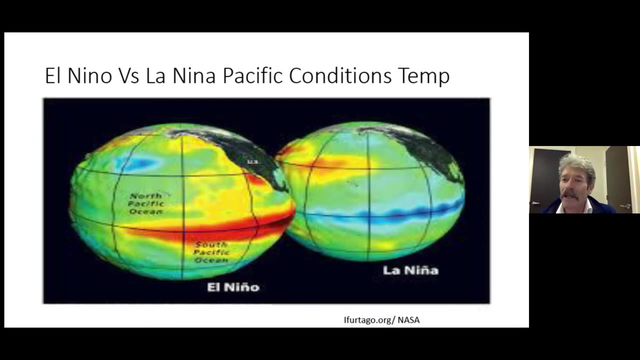 trend line is shown in green, The modern observations are shown in red And these are all of the tree growth recording components of the sporadic, oscillating El Niño. These distorted beach ball-like pictures show the contrasting years between what is a strong El Niño here in. 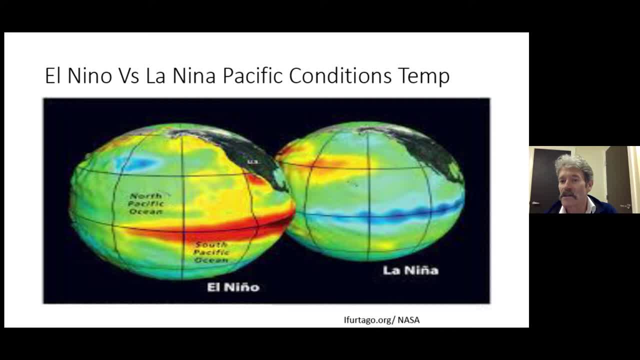 the South Pacific and a La Niña in the South Pacific. These pulse back and forth on two to seven-year cycles, and the areas around them are significantly affected by large swings between the wet and the dry times. Some researchers tie these pulses to solar cycles which have more of. 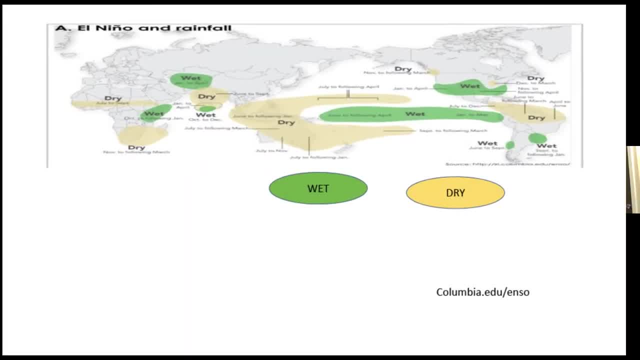 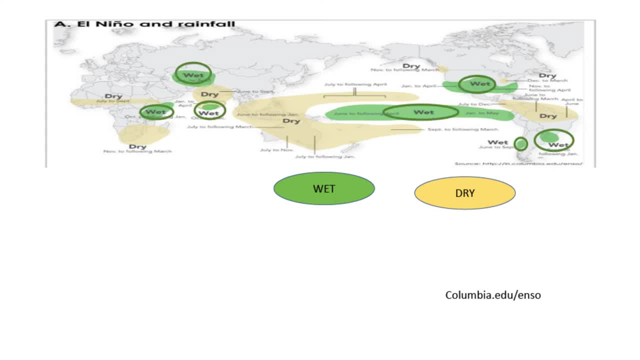 a 10 to 12-year frequency. Here's El Niño and rainfall and what happens? wet and dry. Here's that wet component of El Niño in the Pacific. Here are the dry areas of Australia and South America beside it. 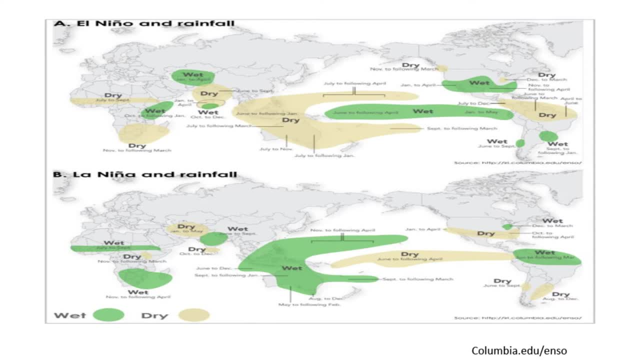 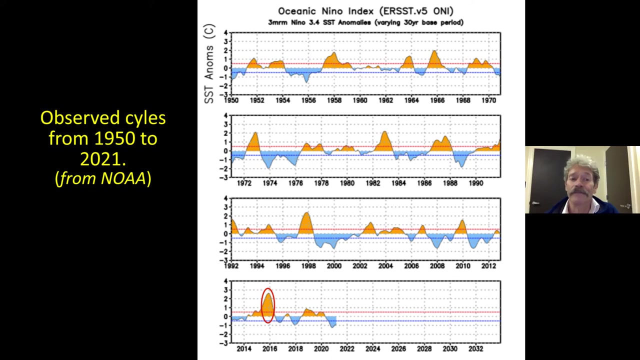 Then you put in La Niña and its rainfall and you get what is almost a perfect mirror image within the areas of the tropics. So what was wet, It's dry. What was dry is wet. This is the 2016 El Niño. 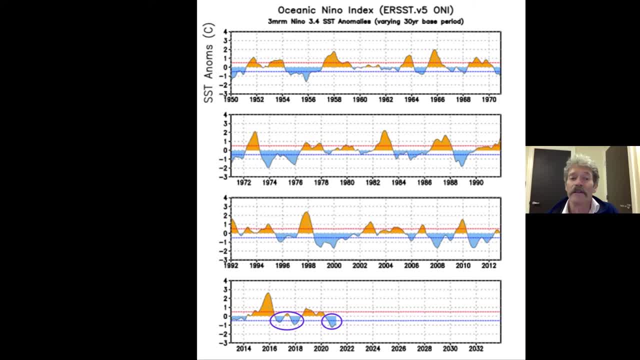 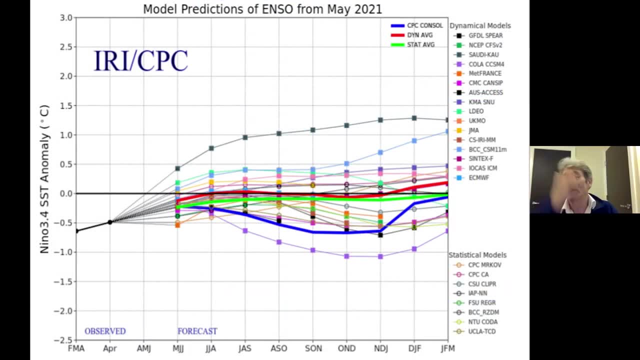 These are the cooler periods that followed it. We're now into the 2021 El Niño, sorry, La Niña. If models are made- and they are- of this surface sea temperature prediction, what happens here? We've got a complete 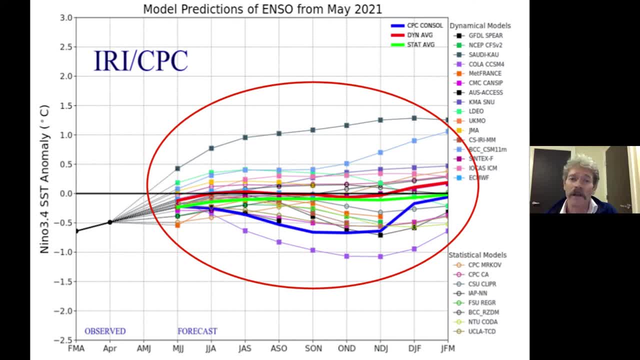 complete scatter, and these are the models that have been built to try to anticipate what El Niño is going to be like in the future. This is April of 2021.. The studies of the ocean current systems need a significant amount of work, as the ocean systems are said to control 90% of the heat flow imbalances of the atmospheric models. 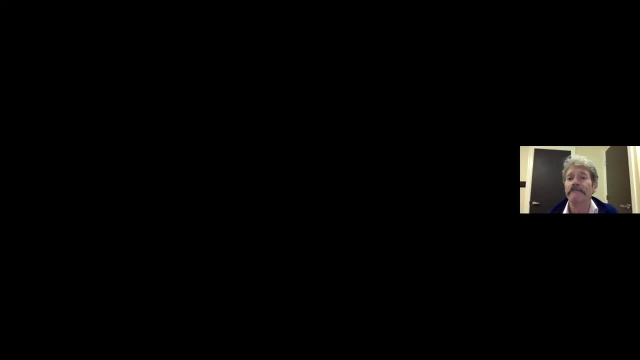 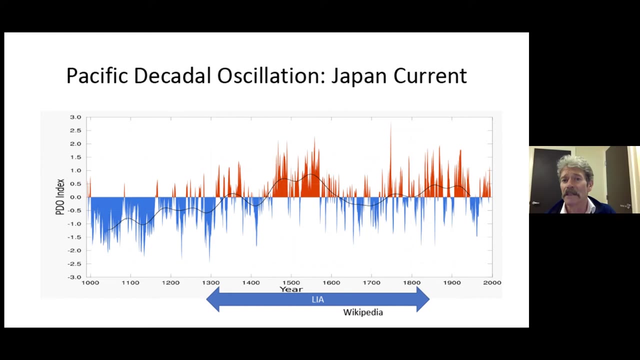 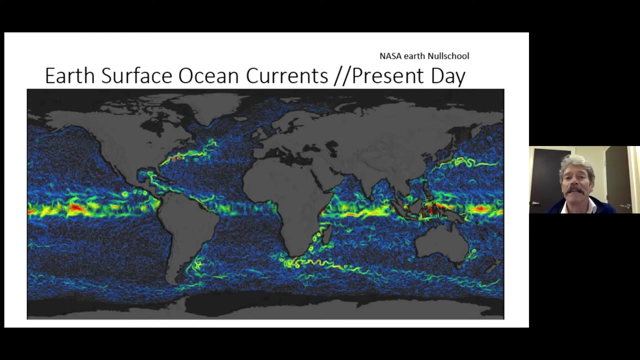 Here we have a scatter. north of El Niño There is something which is called the Pacific Decadal Oscillation, more along the lines of a decade long, like the solar cycles. The Japanese current makes up a big part of that. This is a picture made by NASA in their Null School on the internet. 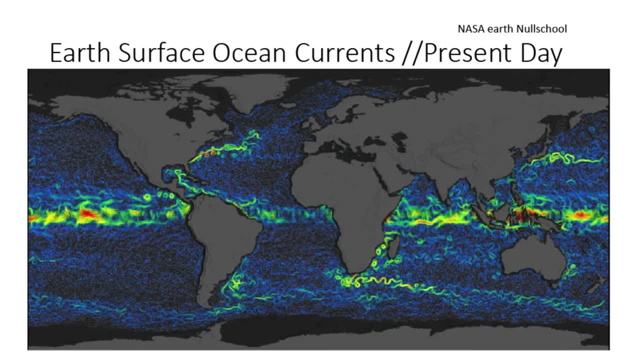 What it shows is the currents, The ENCO, ENCO, ENCO- This is the comfortable This would be El Niño. It shows the Gulf Stream Here, It shows the Japanese current here and the rest of the tropical and subtropical Southern currents that exist within the world. 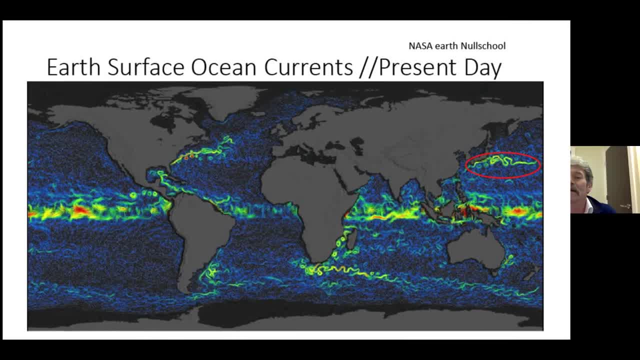 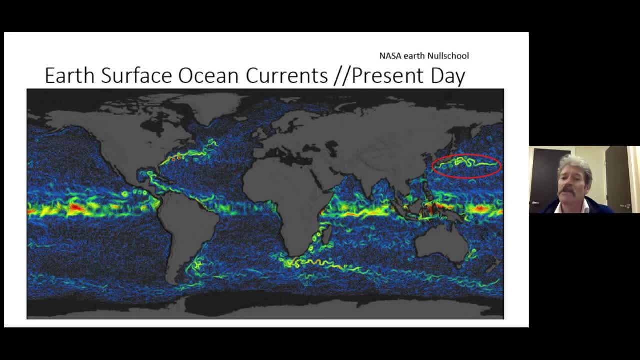 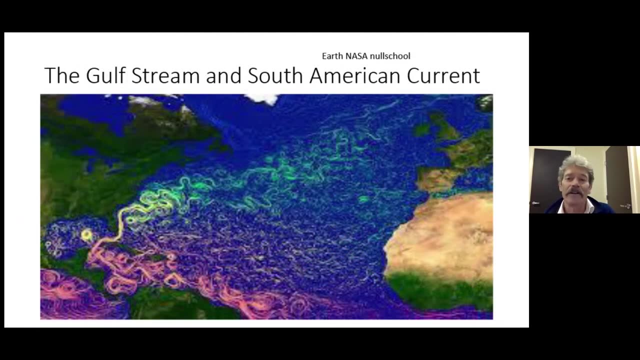 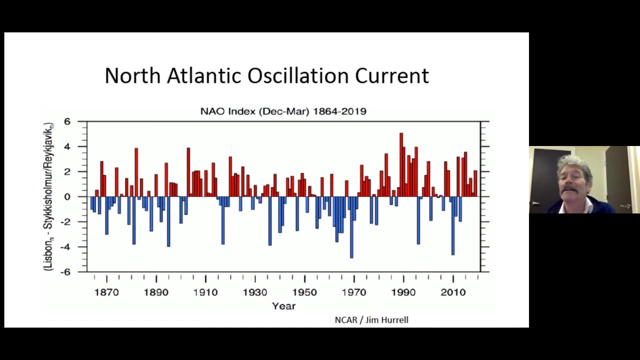 Europe needs the Gulf Stream, Japan. the influence of the Japanese current, The ENCO, is big and very important. ENCO, ENCO engines of our current neoglacial period. Would Europe be like northern Canada or Russia without the Gulf Stream? This is the oscillation of that North Atlantic current and how it varies from. 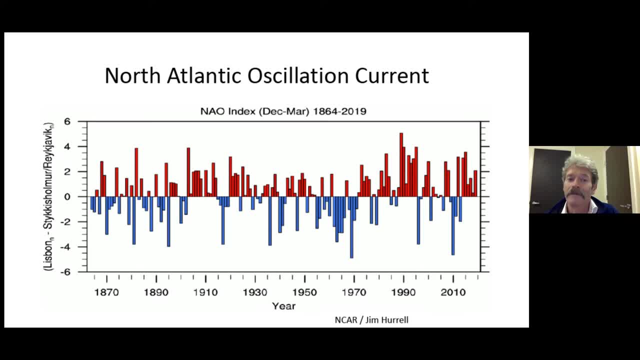 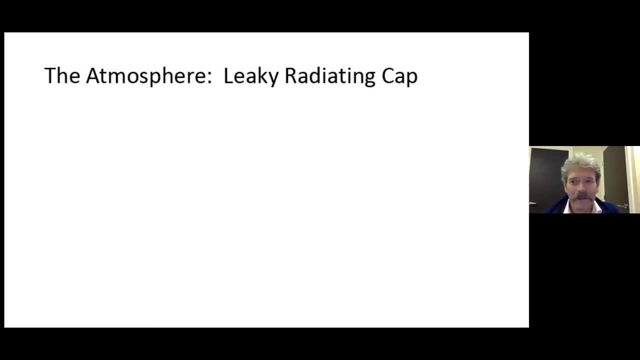 warmer to colder and completely controls the European weather systems and sometimes even fish yields The atmosphere. I'm going to call it a leaky radiating cap. I'll get to that in a little while. why I've termed it that way? It's a complex, layered composition, of course very important to 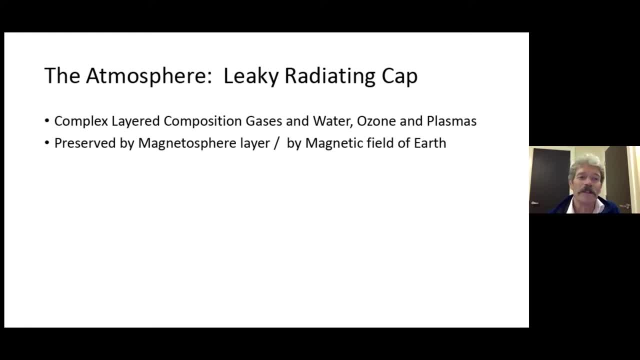 us of gases and water and ozone and plasmas. It's preserved by the magnetosphere, a layer up higher, which are protected by the zone that the magnetic field of the Earth protects us from the solar radiation. in The lower troposphere is dominated by water vapor and ocean energy. as we've discussed, The water vapor varies. 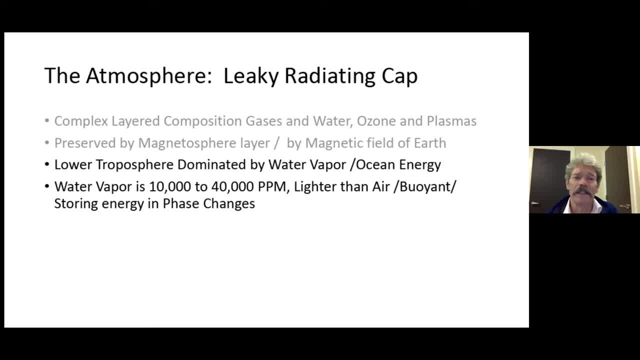 from 10,000 to 40,000 parts per million and is much lighter and buoyant in air, air being dominantly oxygen and nitrogen. Storing energy in its phases is what water can do and very successfully modifies the world's oceans- sorry, the world's weather and climate as a result. Thermal inversions above the tropopause. 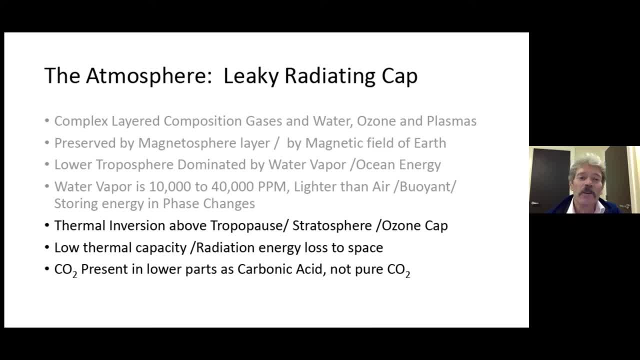 and the stratosphere and the ozone cap area are something that we'll probably have to deal with in later, but we will talk about briefly here. The atmosphere has a low thermal capacity. It operates by energy loss, dominantly loss to space. So that's the leaky cap part of it. The CO2 present in the lower parts is not present in the form that we have been told or how we have. 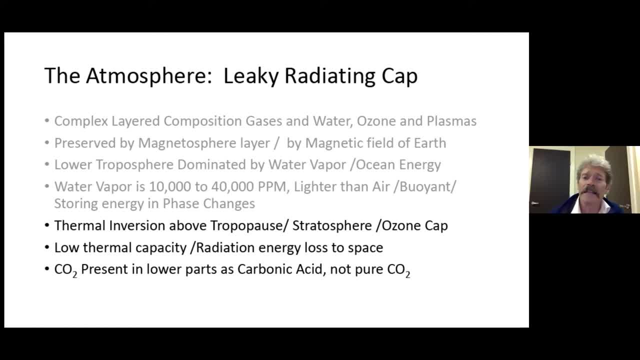 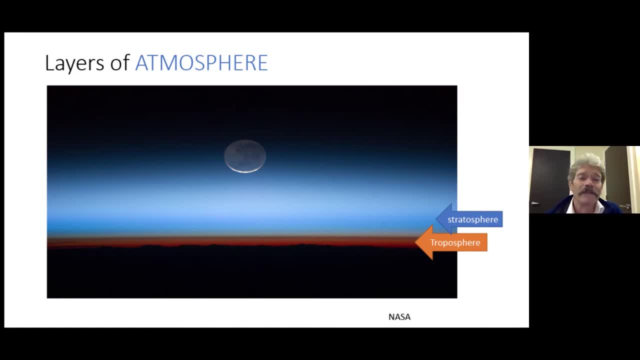 alluded to it before. It's not pure CO2.. and we'll get into that with our discussions of carbonic acid. The layers of this atmosphere are shown here by a space shuttle shot. The troposphere is that oranger zone down closer to the surface. 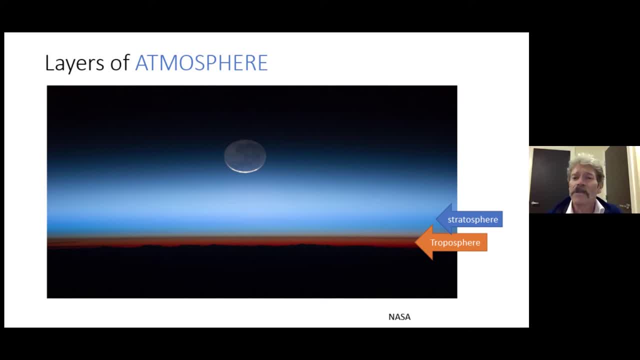 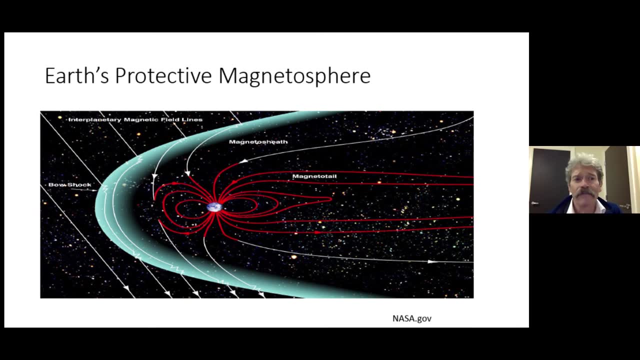 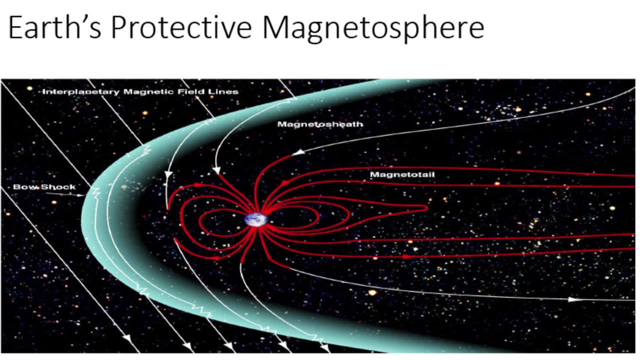 and, of course, is the area that we're most concerned with. The stratosphere is above it. The ozone layer is within that stratosphere. Here's that magnetosphere, the Earth's protective shell, Because we have a magnetic field in the Earth, the lines of magnetic force control. 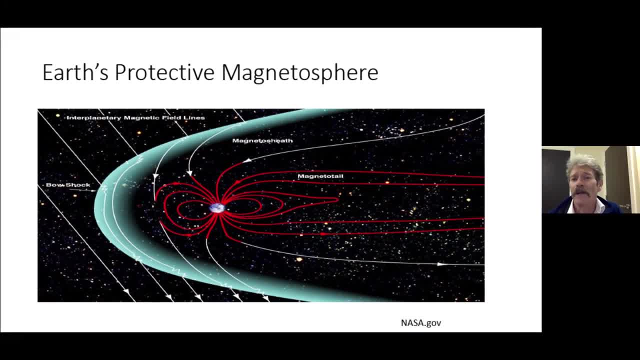 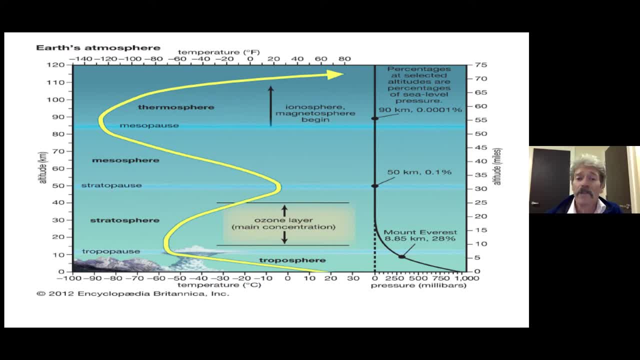 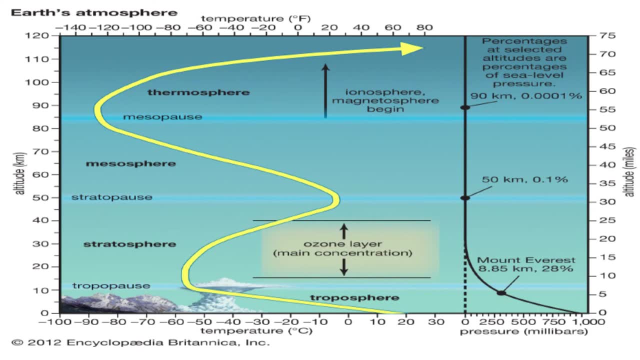 this shock wave, this bow wave, which would otherwise be highly destructive to our atmosphere. Here are those layers Below that protective magnetic envelope, our atmosphere has formed and retained a layered structure. The yellow line shows the temperature profile of the atmosphere. The yellow line shows the temperature profile of the atmosphere. 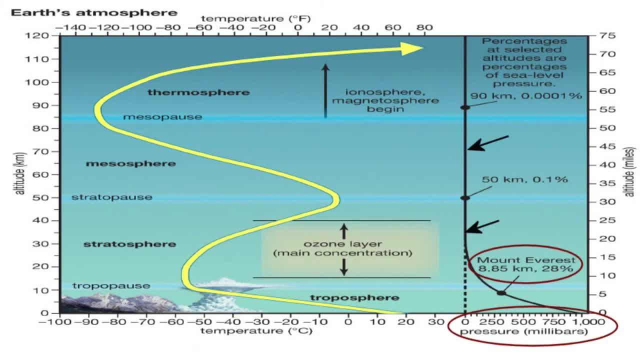 The atmospheric pressure line is the black one on the right and it shows a rapid loss of pressure as we rise above Mount Everest, shown there. Our life zone is the troposphere and it's governed and dominated by water in all of its forms: ice water and gas. This zone lies below the tropopause. 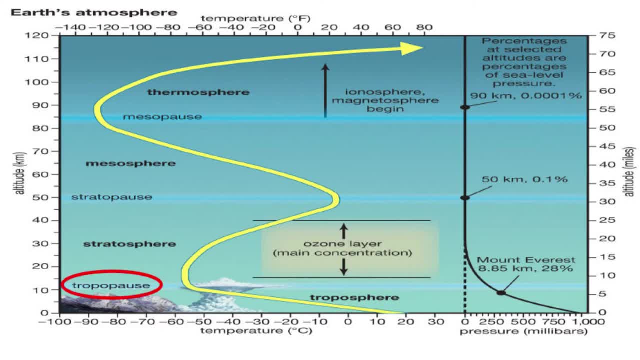 which is a strong thermal inversion, shown here Near the tops of that deck of clouds down there. This thermal inversion is also the point at which ultraviolet light creates an ozone layer which heats. So this is a zone of heating again in the 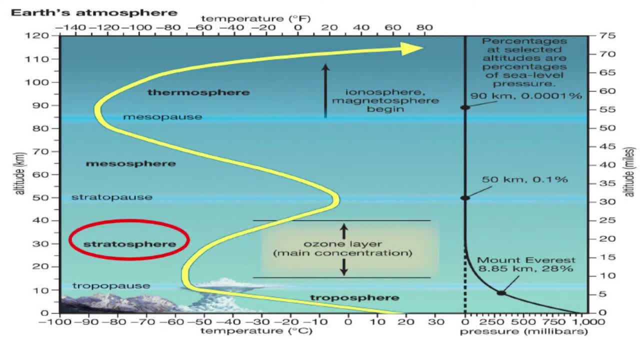 ozone layer. The stratospheric zone is the highest and is the beginning of the tenuous ozone layer and that is an inversion which, of course, caps that thermal loss which we were experiencing in the troposphere. Troposphere has an adiabatic cooling rate. 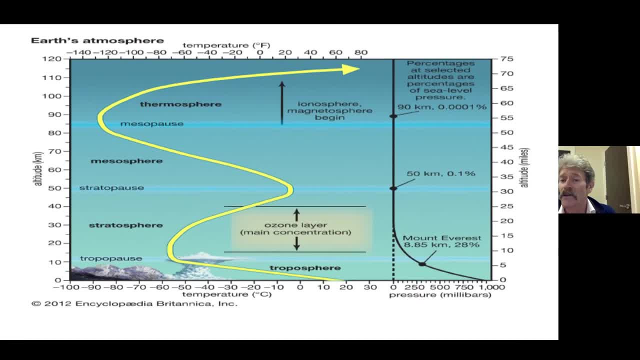 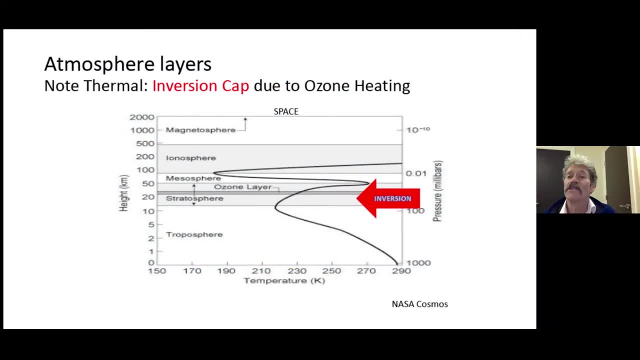 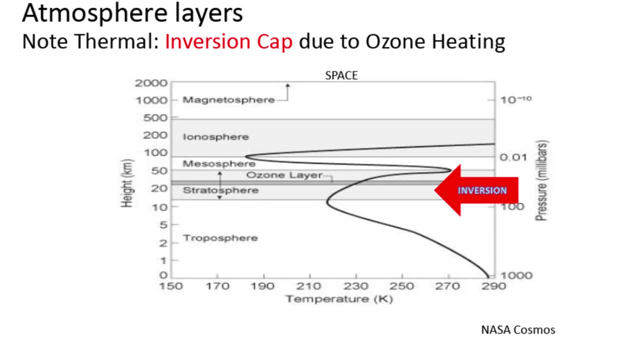 which is very extreme, and then things reverse. Our focus will be on these lower zones. This is another view of that critical inversion zone: capping the thermal heat loss of the troposphere at the tropopause. Above that we see the magnetosphere. 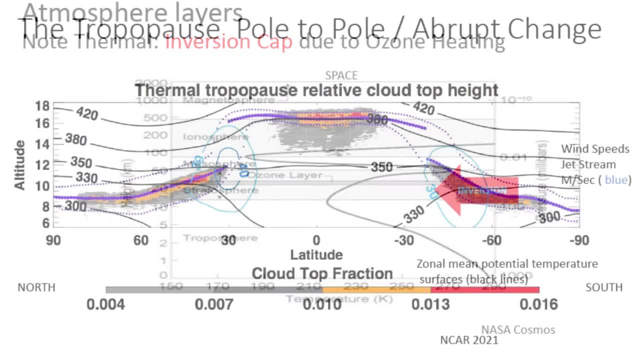 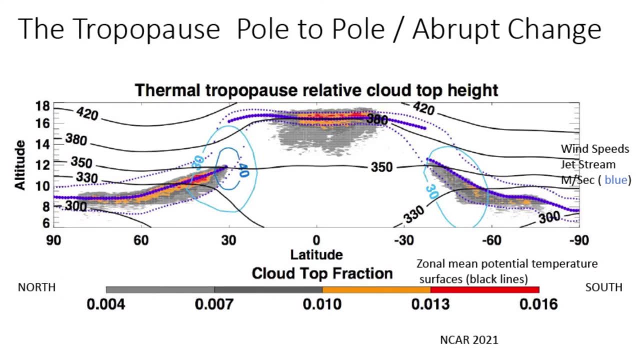 and above it is the cold vacuum of space. This is a view north-south, north to south, and it's cross-sectioned through that lower portion, our troposphere, and shows a very unusual feature Here at the poles. it's low and this is the cloud. 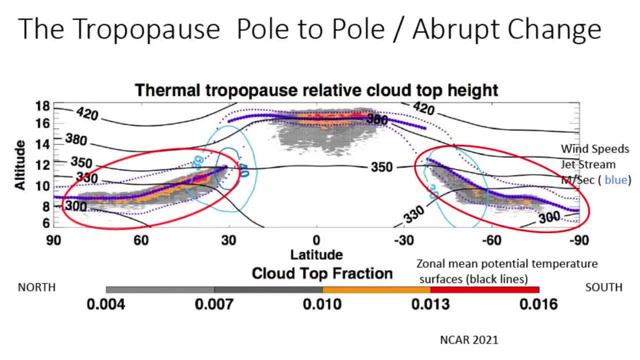 deck and the tropopause here in purple. and this is the tropopause over the equator, at zero latitude. There are jet streams. This is the tropopause over the equator, at zero latitude: There are jet streams. There are jet streams. 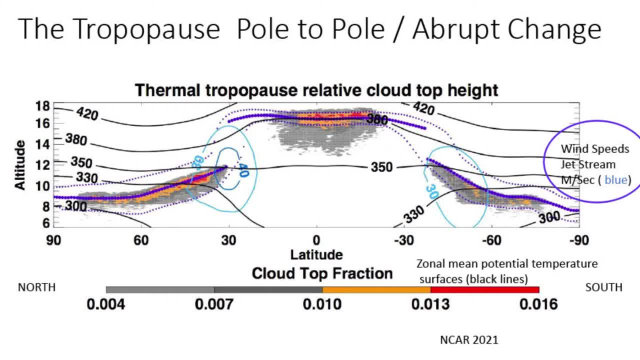 Here's the meniscus we've had over the past year. She was peeled up toещ. Here's a good image of the tropopause. every Okay leads to three seconds. up to eight kilometers at the poles, to get up to it 17 or 18 kilometers or more at the equator. Intense jet streams, as I mentioned, are sitting in those blue areas. They inhabit the portions near the step of the bulge and these winds are due to the inter whistle migril. Now there is no. It could just go per e80 and say: 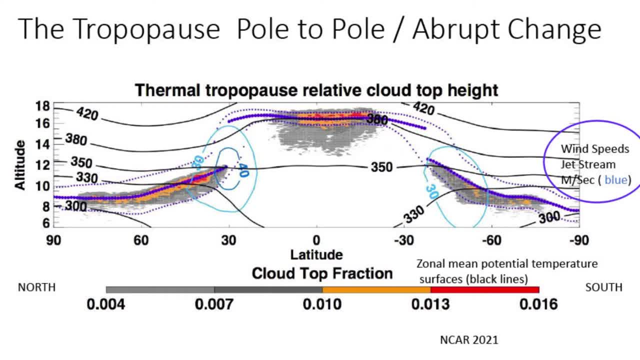 And I know in the past 30,, you know 30, but we have never said pull to than sa i face of the thermal zones and the Coriolis forces from the rotation of the earth. These wind systems partially isolate the polar regions from the equatorial regions and the complete thermal regime. 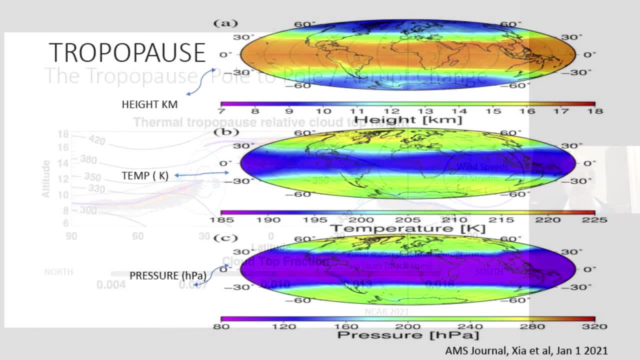 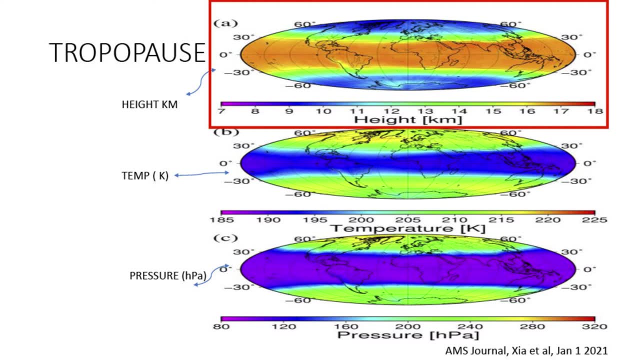 will be a little clearer later on. This is a picture taking the world in three different views. This is the height of the tropopause in kilometers. This is the temperature of that tropopause and this is the pressure of the air pressure in it, This sudden break in temperature. 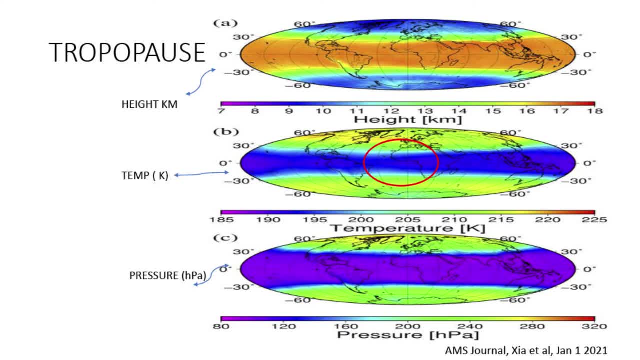 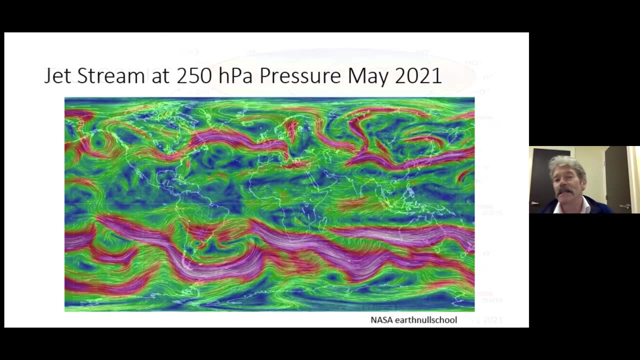 profiles is where we are seeing that large step At the equinox is where we're viewing this: not extreme winter or summer, but extreme winter-summer seasonal tilts of the axis of the earth Move these zones north or south. This is a view showing upper level winds of the earth. 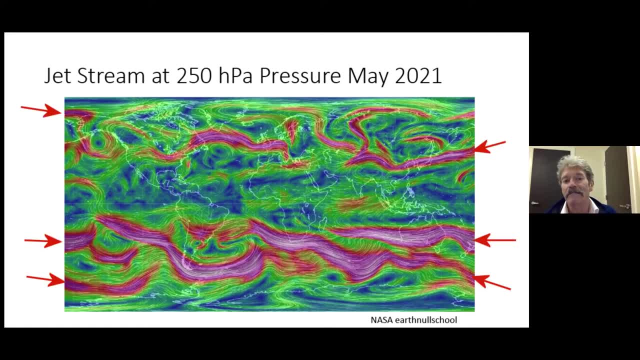 very high velocity winds in these areas: 200 to 300 kilometers per hour. This is the barrier now, in May of 2021, against the warming versus the cooling, So it is isolating those parts of the atmosphere. These are the portions that 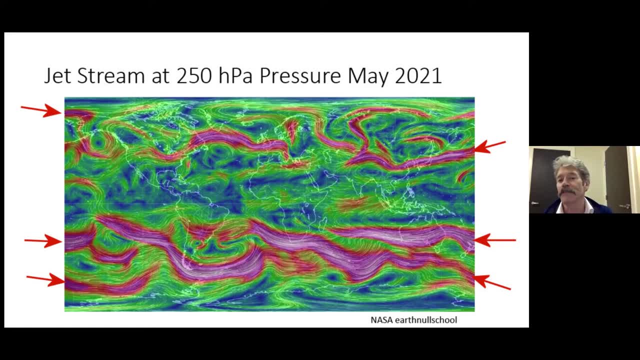 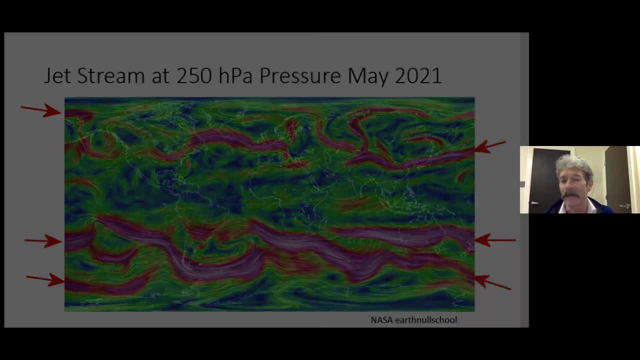 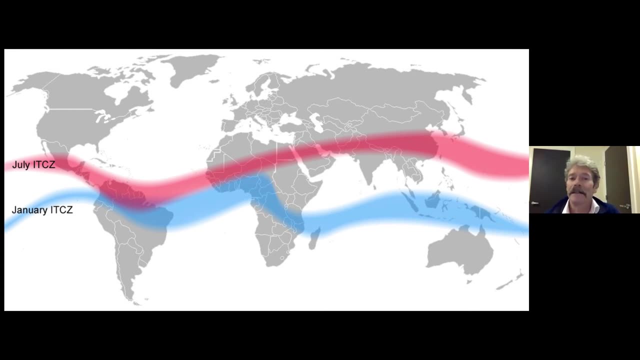 of course sit where the blue areas were in the last diagram. It's of a low pressure zone higher up in the atmosphere where these jet streams exist and dominate. So we get back to that ITCZ, the variation it did. in today's world It moves but it's quite. 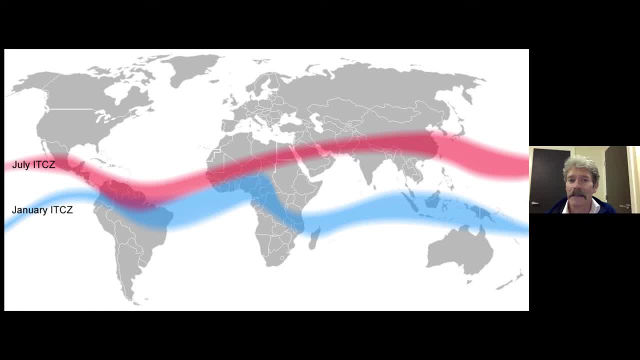 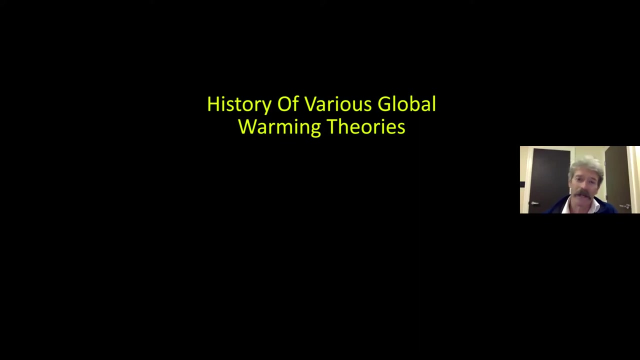 asymmetric. It's not equal around the equator as we might think. It moves from July here in the north northern hemisphere summer to northern hemisphere winter. here Sometimes it's coincident, other times quite separate. under the current conditions, This is an attempt to talk in a very capsuled way about the history of global warming theory. 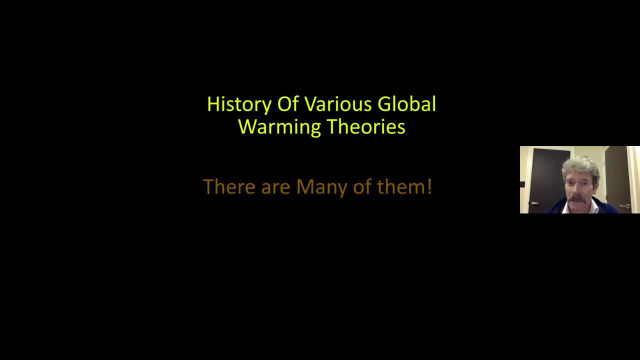 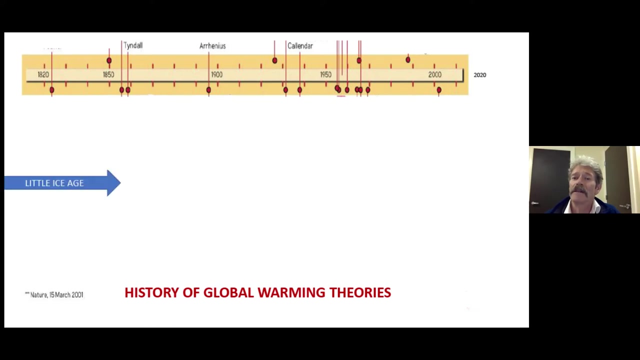 We still have to think about it as a theory, like a lot of other theories, and still needing a lot of proofs and a lot of further development. This slide represents the timeline of global warming theory, the greenhouse theory, from earliest times, during the emergence from the little ice. 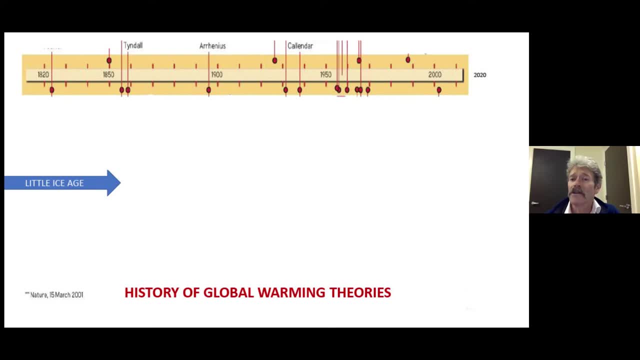 age. back over here The proponents during this very early period, most notably this particular fellow here. Arrhenius, published on something during a global cooling period. He was emerging in Sweden from the little ice age. He published in 1896 and proposed the theory of greenhouse. 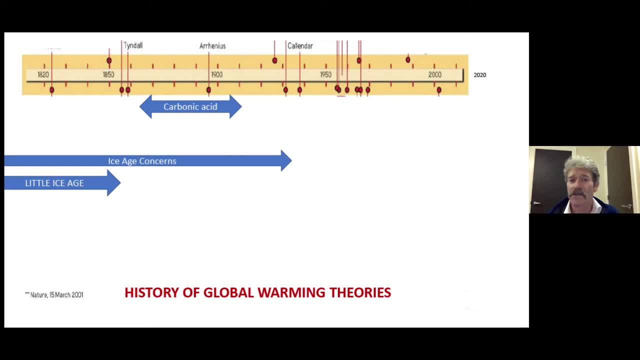 gas. He hoped that it would preserve the temperature of the earth and make it warmer. Carbonic acid is what he used in his analysis and he was right. His conjecture, his early conjecture, was about carbonic acid to extract the earth from this cold period. The theory was in touch. 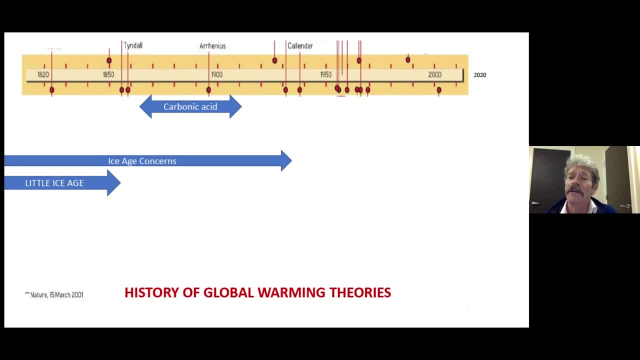 with the real form of carbonic acid. The theory was in touch with the real form of carbonic acid, of CO2, in the atmosphere where it combines with water vapor. This is a biological atmospheric theory. Subsequent efforts to look at the theory stumbled on saturation of greenhouse gases and 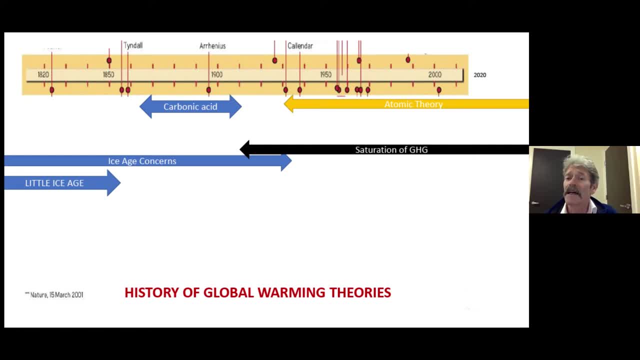 the effects then of the atomic theory, to analyze it and how irradiation affected these vibrating greenhouse gases Of significant note. it took until 1933 to discover how plants actually receive and process water and CO2 by the use of this catalyst, carbonic anhydrase. Without it, 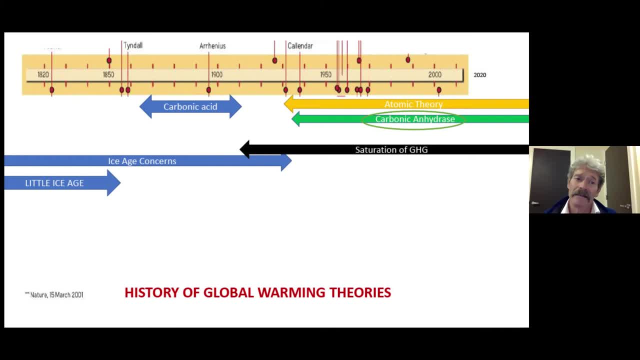 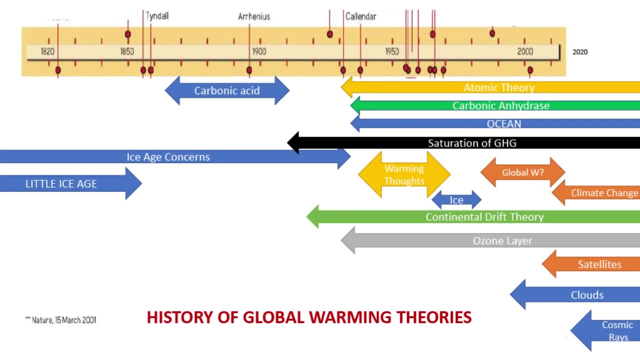 we would not be able to break down the carbonic acid in the system to generate the products necessary for photosynthesis. Other discoveries, such as continental drift, have allowed us to modify how we look at climate and the drivers, as we did in part one. Only very recently have 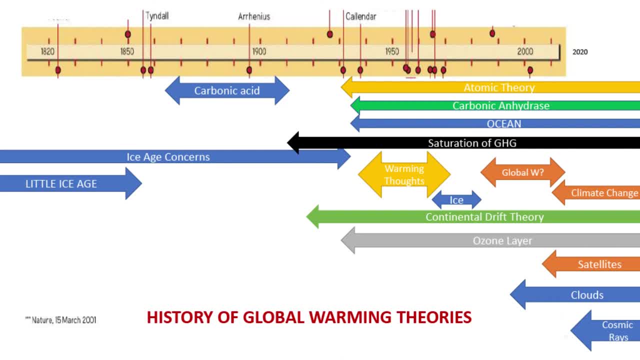 the major drivers of climate change and climate change in the world have been the carbonic acid. We've also got to include the ocean involvement. We've got to include the ozone layer And, lastly, the contribution of clouds and cosmic radiation. These might have to be part of a third talk. 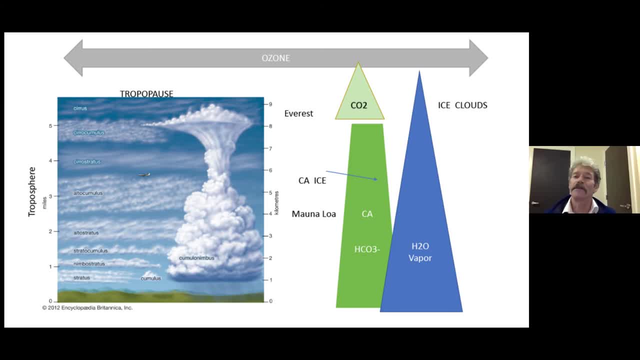 So this might be a way of looking at the abundance and temperature regulating components of the gases in the atmosphere, the two major ones: water vapor, which is dominant and lighter than the other gases. It falls off with elevation. however, It is topped out at the freezing point in the high clouds. 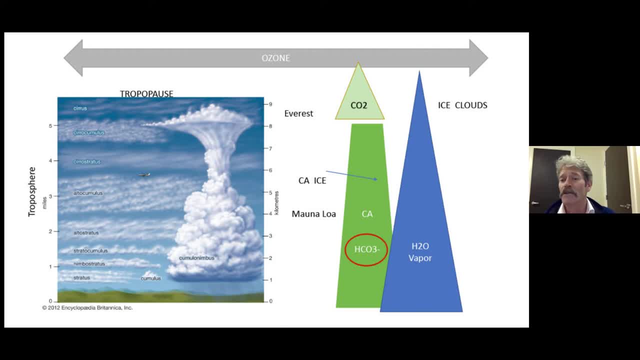 like the cirrus clouds shown here In the lower troposphere. CO2 is tied up as carbonic acid and water in the water vapor and it rises with it, separating in the upper atmosphere at the freezing point. The dynamics of real atmosphere and CO2 needs to be better understood. 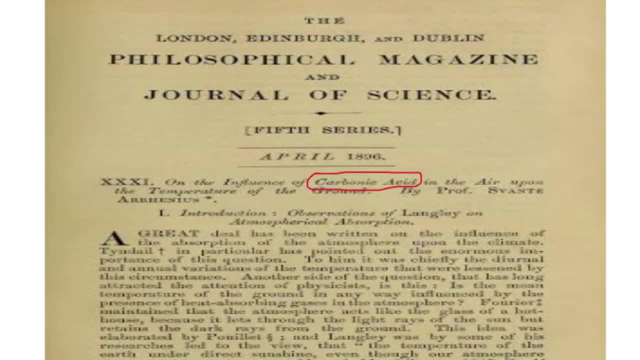 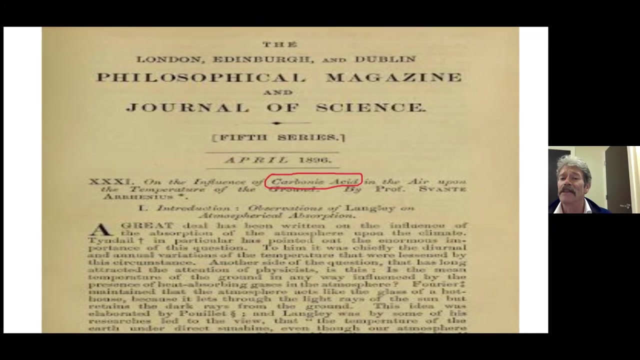 Let's have a closer look. This was the original paper of Arrhenius Greenhouse Gas Theory. It involved carbonic acid- not CO2, but for good reasons. In this paper he knew about biochemistry of CO2 and water. He used these to actually support his theory. He was living in Sweden. 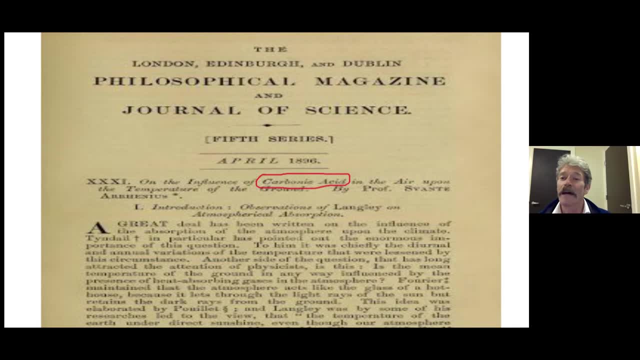 and it was pretty cold. We have strayed further from the path of real data and science that Arrhenius might have been trying to bring. I'm going to stop here, talk to you in a few minutes. See you then, Bye-bye. 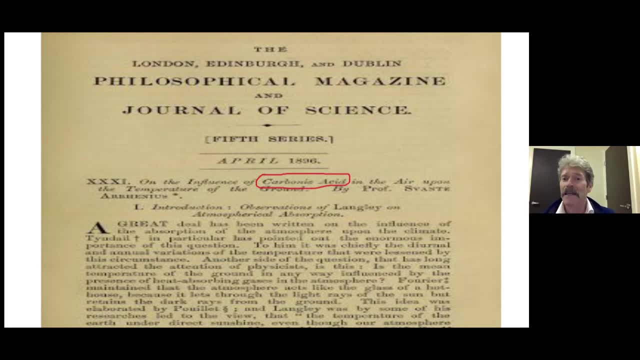 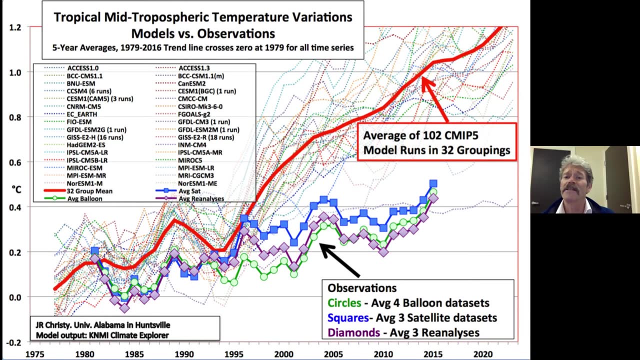 look at. We have generated models. They have not done very well. This illustrates the upper tropospheric results predicted versus the hard facts shown by balloons and satellites, etc. The only model of this group of 102 to even come close to reality is in this atmospheric level was 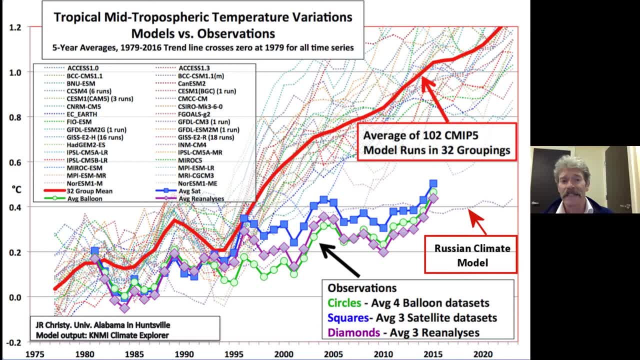 conducted by a group of Russian scientists. These are all those other ones, as an average of them, all this scatter, These are the actual results from balloon and satellite data sets. This is all in very real time. This period here- 1995, is about where we start to depart from reality with 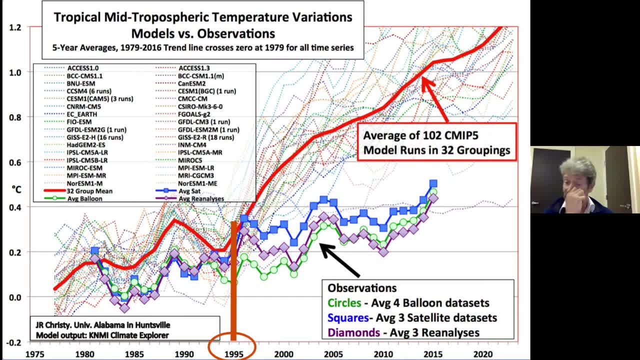 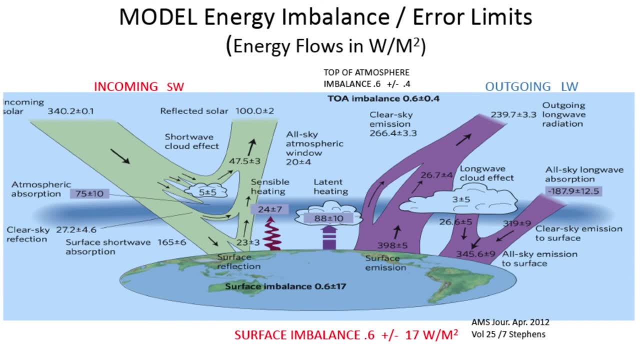 the models. Why do we still use these projections for our political planning purposes? Let's look at some major problems and techniques of computer predictive modeling. This is a complex cartoon, often forming the basis for atmospheric temperature predictions. It is so complex that the individual parts have large estimations without data underlying them. These have error limits. 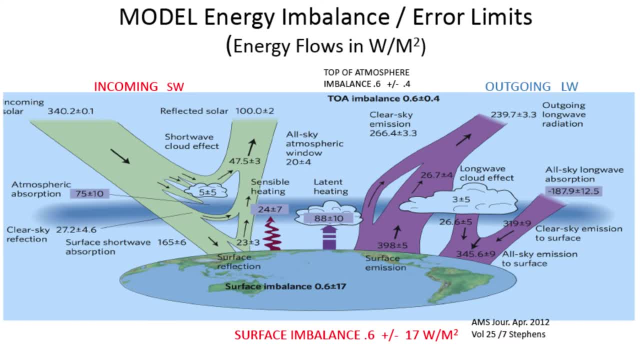 but they're not stated. Most models do not properly lay out these error limits. Any good experiment or research paper must be done. The model of this group of 102, to even come close to reality, must do so. This illustration is an honest attempt, however, to quantify the pluses or minuses error. 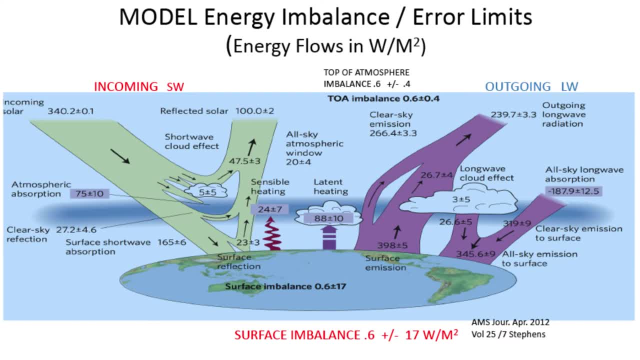 limits of various arrows and energy flows in the atmosphere only. We're forgetting about the ocean, and we're forgetting about clouds in this particular case as well. Why are the model errors so great? Why do environmental error limits vastly exceed the resolution of the predicted? 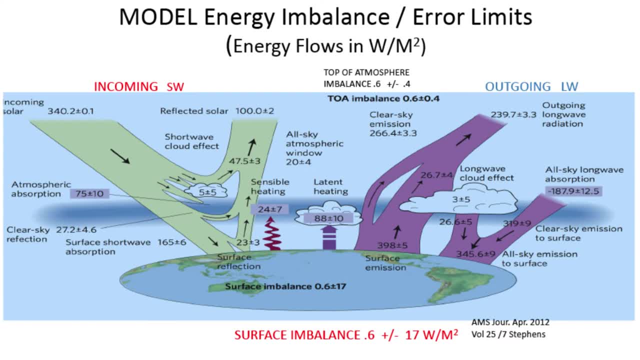 outcomes. Let's look at some of these experimental errors. The surface imbalance: here This is 0.6 watts per square meter. It is plus or minus 17.. The credibility has been lost and many variables are being used without foundation. This is the problem of using models in a very dynamic 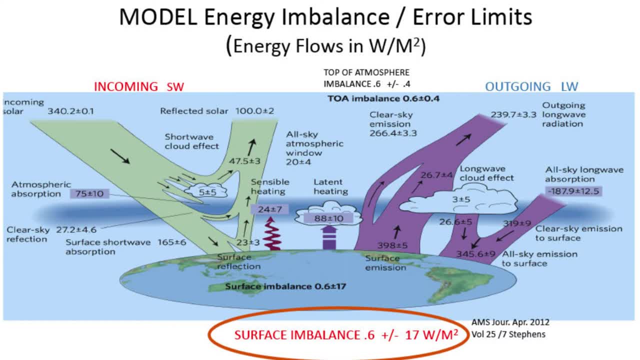 interactive natural system. The resolution of the answers are too small to fit and the regression is not consistent. This is the problem of using models. within the limits of the errors that are evident in the assumptions, No graduate thesis could ever receive a passing grade. 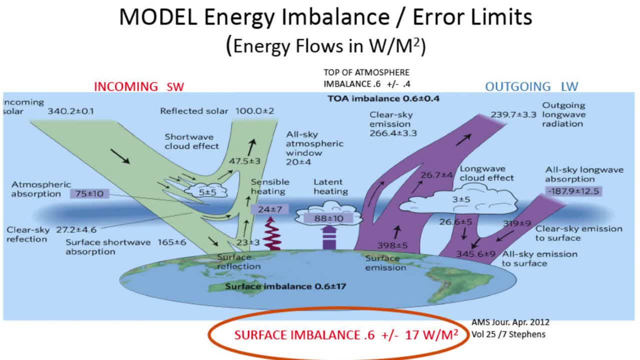 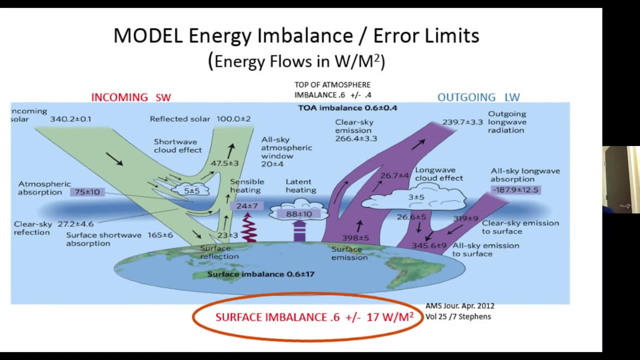 if it suffered from so many errors and did not quote its limitations in numbers. its error bars. Very large natural energy systems of the ocean and the clouds are missing and incomplete in these predictions. The size of these errors in judgment and the projection of imbalances are estimated to 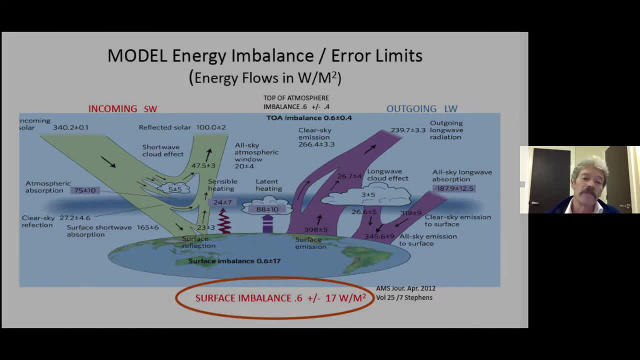 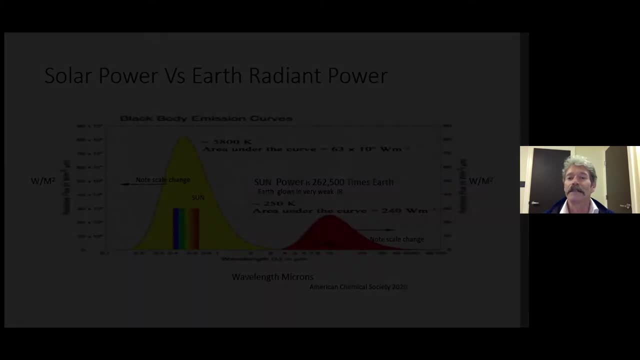 be 90% for the ocean. This is a very large number. The size of these errors and the reduction of the the ocean and up to 30% for those clouds. The physics of solar radiation in the atmosphere is what we're going to review now. These are the radiation black body curves, so-called for energy. 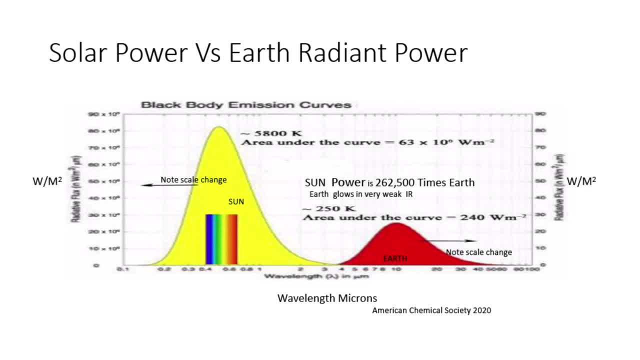 radiation absorption. These are relative to the sun and to the earth- solar and earth. They are on a common wavelength horizontal axis but are grossly exaggerated in their vertical axis to fit on the chart. The earth black body curve radiates very weakly in the infrared. 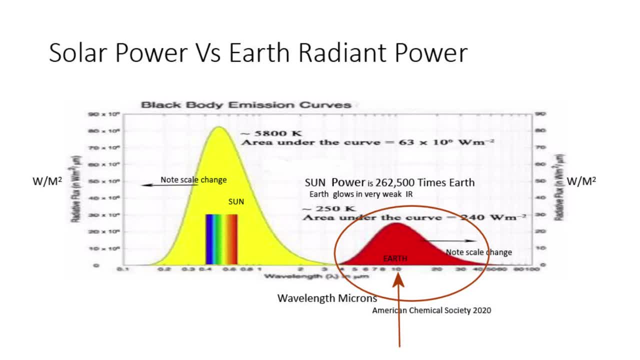 spectral area peaking at about 10 microns of wavelength. The sun black body curve is in the visible spectrum- and very high energy wavelengths at about 0.5 microns. Solar variations heat and have a significant effect on the radiation budget of the earth. The vertical power. 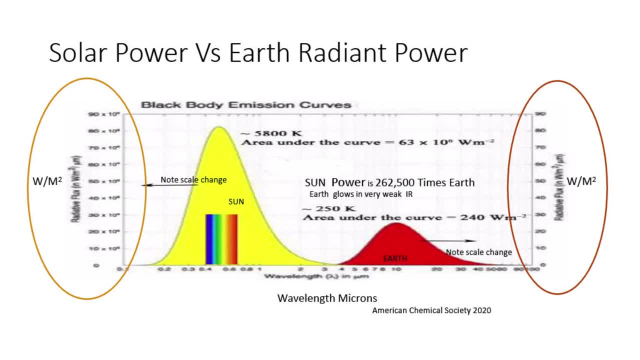 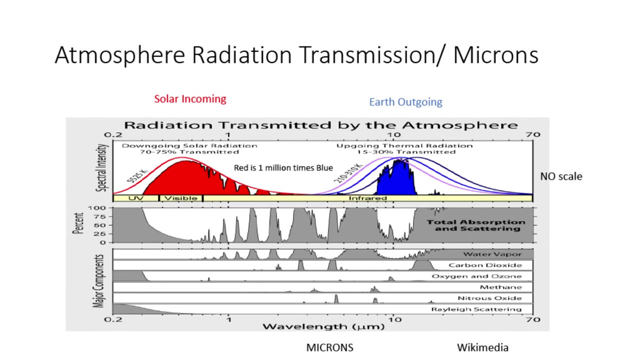 scale is totally different between the two sides: a million to one. The cumulative power, the area under the curves, can be also compared only with numbers. Here we see a difference of 262,500 times in the power under these two curves. Solar variations dominate the incoming high. 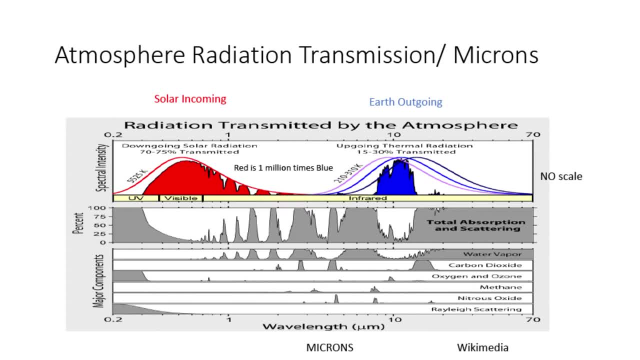 energy, shortwave radiation, as do clouds, water vapor and highly reflected snow ice, etc. The outgoing radiation window of earth is shown in blue and the incoming solar radiation curve is shown here, remembering that these are vastly different in their real scale, But this gives us a chance to look at the absorption. 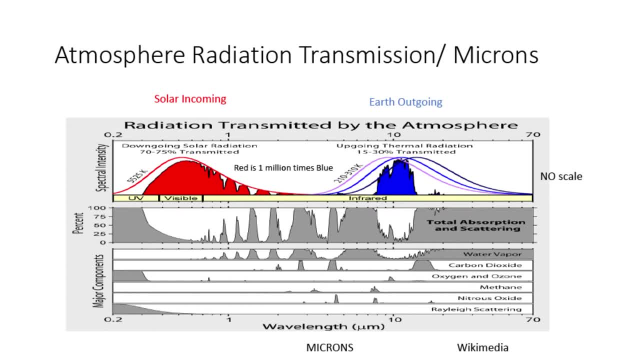 the various substances within the air that are doing that, absorbing, and the percentage of total absorption that takes place. We're dealing with the same microns across the bottom – 10 for the center of the earth and about 0.5 for the center of the sun. We'll call these fields 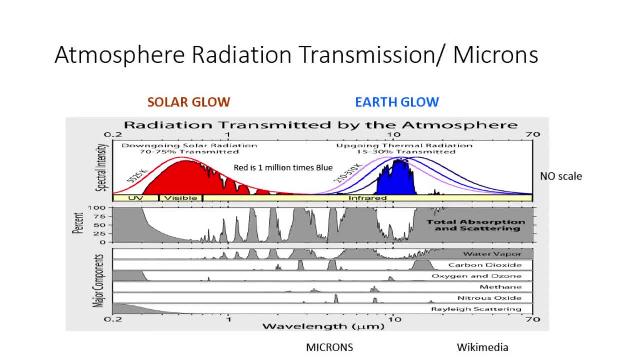 the earth glow and the solar glow over here. We have various lines here which are showing different temperatures As we rise up in the atmosphere. we have to consider different areas of temperature which the earth's能材, emrác, Earth's atmosphere has. These are in degrees Kelvin. The major active gases are going to be: 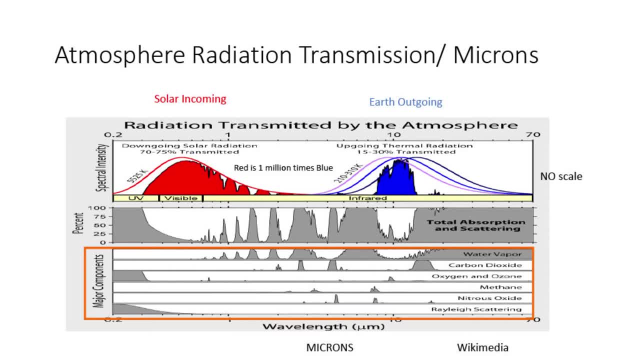 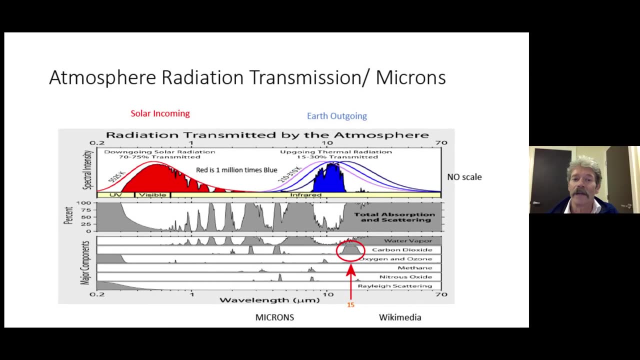 discussed. We're going to be looking at also the positions of each one of these peaks. These are the peaks in water. These are of carbon dioxide, very spiky and localized- This is one which we'll concentrate on a lot here- at 15 microns. This is what happens to the energy as we move across. 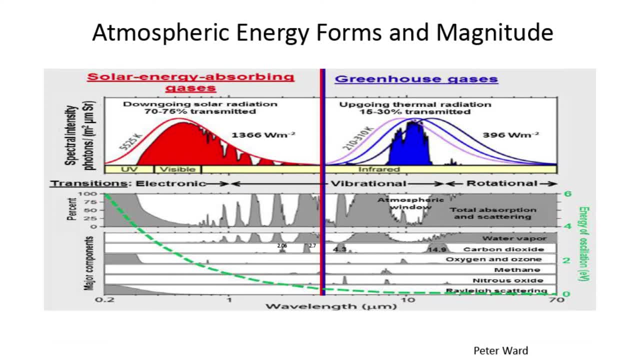 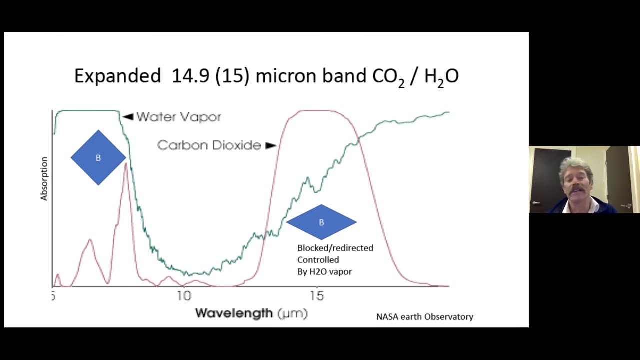 this same diagram. Energy falls drastically across the diagram here in electron volts of oscillating energy. These are the electronic components of energy absorption, vibrational and then finally rotational components of that, If we look at that one band over in the CO2 side. 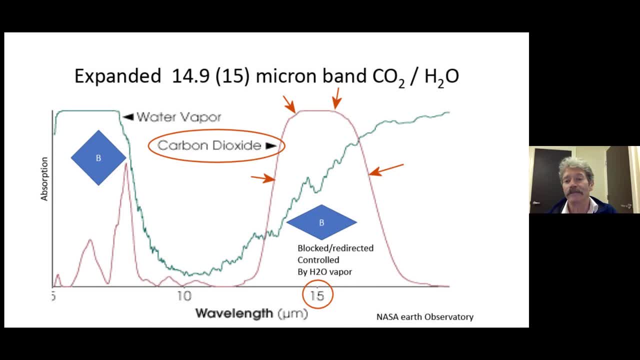 here pictured in red, it is over, It's overlapped and strongly blocked and redirected by the water vapor which drapes over it. This is the problem of using any of this information from satellites: It can't be seen, It is occluded. 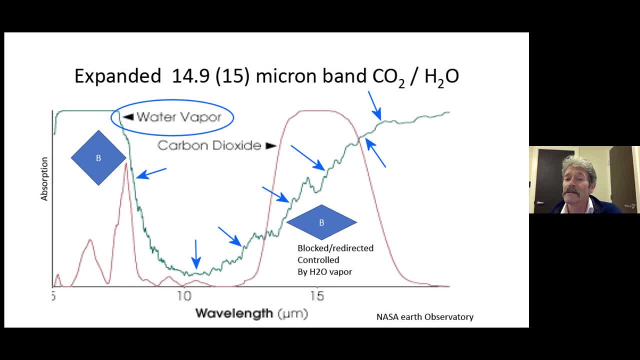 from view and can't be used as part of the analysis. In the lower atmosphere, water molecules vastly outnumber carbon dioxide molecules and dominate this blocking effect and redirection of energy into the water molecule, It's vibrations and its rotations. This is the biggest thing that happens in CO2 in the 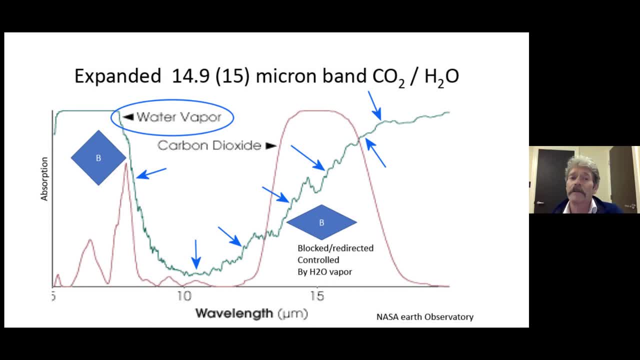 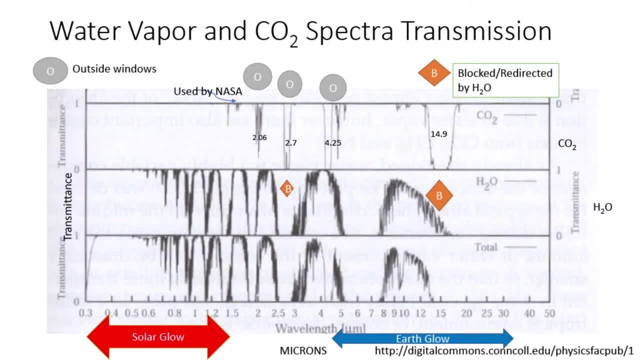 atmosphere, but we're going to show what is wrong with using that as part of the theory. This is a comparison using satellite information. What we're dealing with here is CO2.. Here is that: one large band at 14.9 to 15 microns. 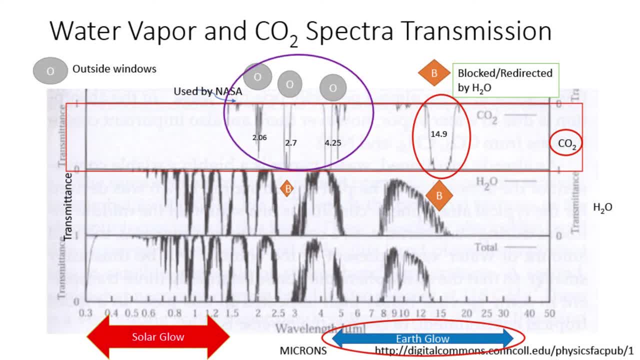 The earth glows are outside of the earth glow. They are- oh, all three of these are outside of CO2.. NASA and the European Space Agency use this small band here just barely inside the solar glow component. Why? Because water vapor blocks this or it's outside of the radiation bands. 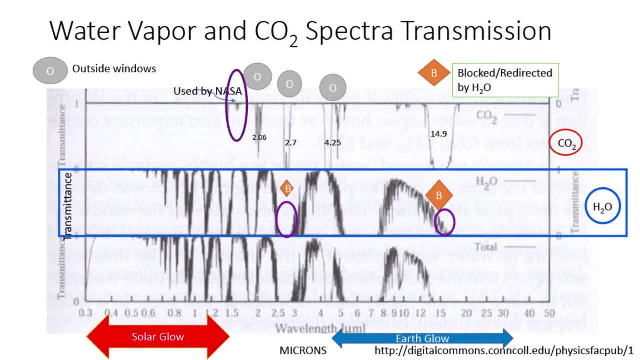 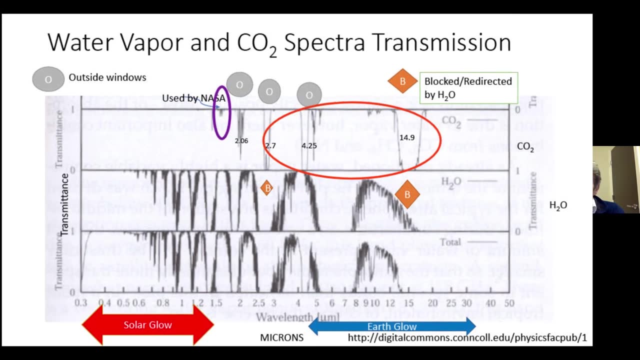 which we're trying to use to analyze greenhouse gas retention of energy. They're using this one over here to comment on all of this. The blocking and redirection is a very major issue, So to be effective, we really need to consider what is happening where CO2 seems to be dominant. 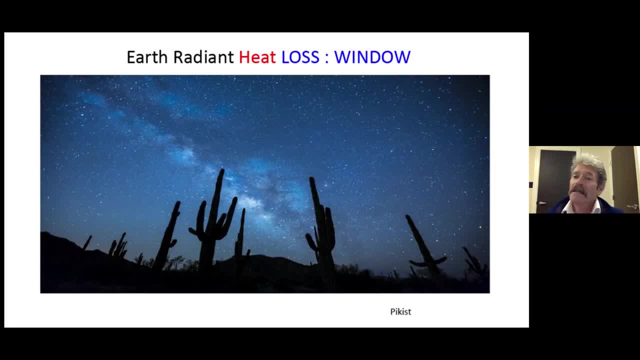 It is not. It's blocked Earth radiates best to space in the water-free, dry parts of the atmosphere. Deserts like this easily radiate and cool at night, irrespective of the quantity of CO2 that might be present. It's all dependent upon the water in that atmosphere as to whether it cools rapidly or not. 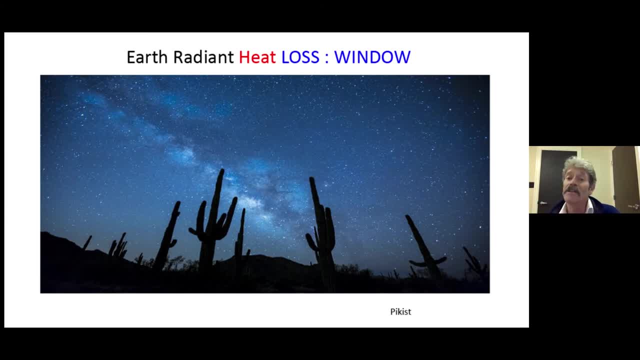 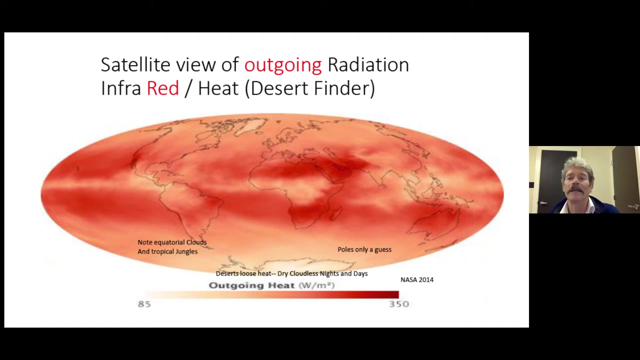 Without water vapor, the atmosphere loses its energy to the cold void of space. CO2 can do nothing to store or retain atmospheric energy. Water vapor does that job. During the day, water vapor absorbs the highest energy parts of the solar spectrum. It is showing radiation heat loss and could be termed a desert finder. 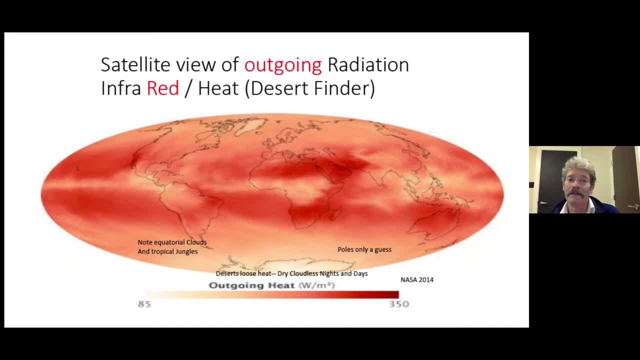 as it is intensely red in much of the desert regions of the Earth. The rest of the story is clouds, which is what's shown here, which block That radiant energy coming up from the Earth, And we also see large stretches of the ocean which are also intense radiators, re-radiators of heat where the clouds are not present. 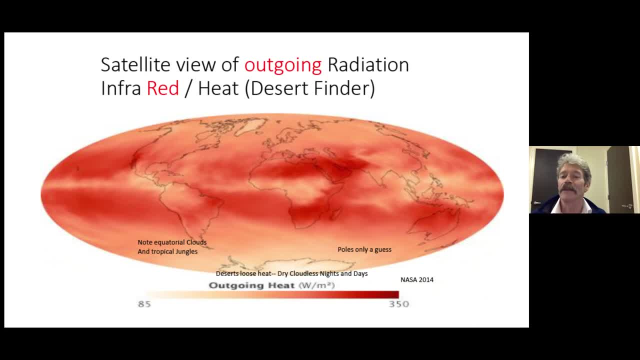 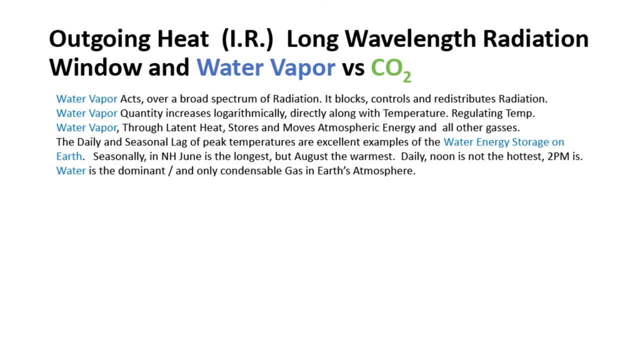 This is a clear air view, or as clear as we can in, as cloud-discised as possible. But we'll see something else from 2018 that analyzes that better: The outgoing heat, The infrared radiation, long wavelength radiation, which is the Earth's glow, and water vapor and CO2, is what we want to talk about in brief here. 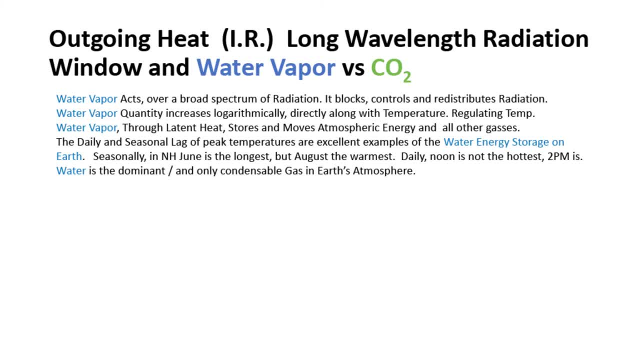 This is a contrasting kind of a slide. We're saying that water vapor acts over a very broad spectrum. It blocks and controls and redistributes the radiation. Water vapor's quantity increases logarithmically, directly along with temperature, and regulates Temperature and vice versa. 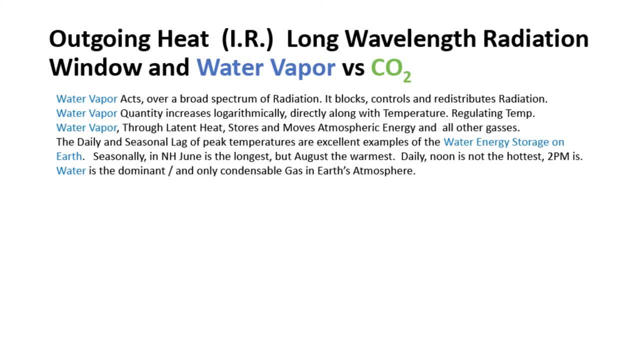 Water vapor, through its latent heat, stores and moves atmospheric energy and all other gases around. Daily and seasonal lags of peak temperature are excellent examples of water energy storage on Earth. Seasonal North America: we have June as the longest day, but August is the warmest. 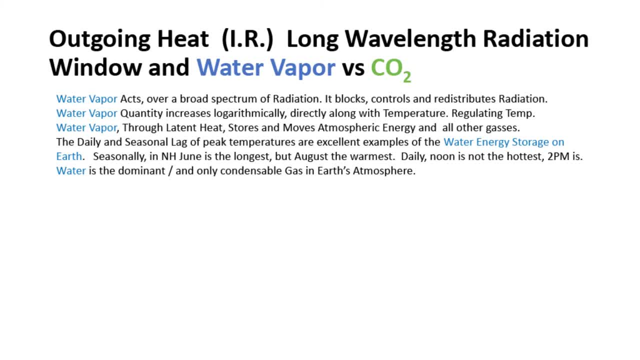 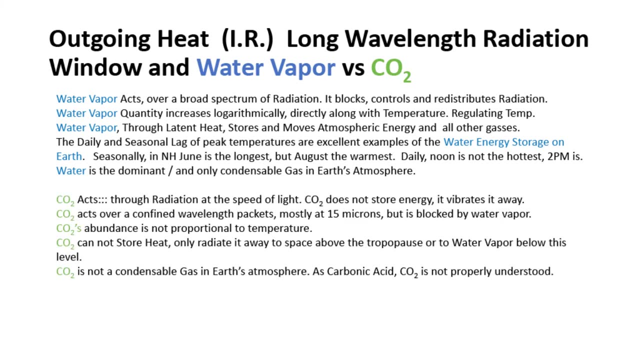 And daily. we've got noon, which should be the hottest, but it isn't. It's 2 o'clock in the afternoon. Water is the dominant and only condensable gas in the Earth's atmosphere. Now to contrast that CO2 acts through radiation at the speed of light, does not store energy and it vibrates it away. 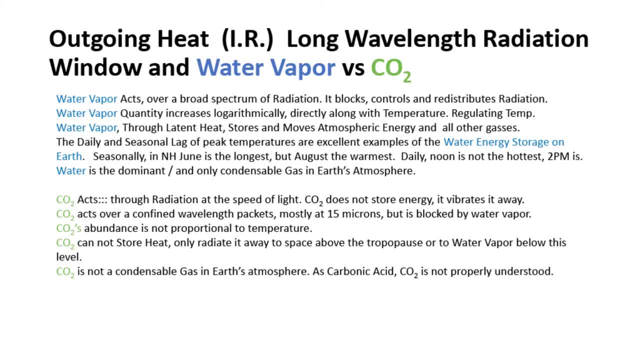 CO2 acts over a confined wavelength, in packets mostly at 15 microns, but is blocked there by water vapor. The abundance is not proportional to temperature. CO2 cannot store heat, only radiated away to space above the tropopause or to water vapor below that level. 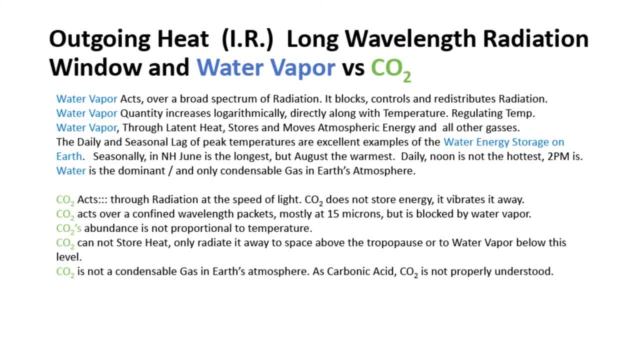 CO2 is not a condensable gas in the Earth's atmosphere And, as carbonic acid, CO2 is not properly understood. So we're going to try and elucidate on many of these points. So we've got CO2, it's a really heavy gas. 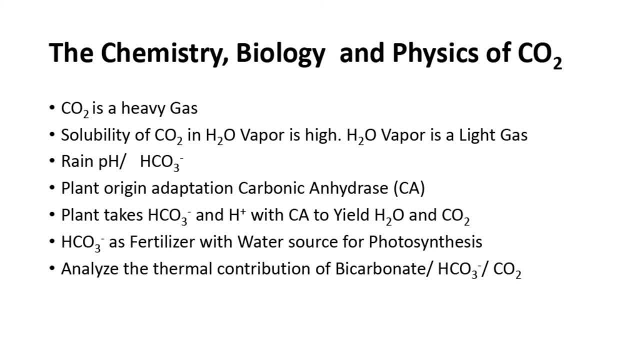 How are we going to move it into the upper atmosphere? Solubility is how we do that. The solubility of CO2 in water vapor is very high, So the water vapor is a very light gas and it lifts it as it's rising and it wants to rise. 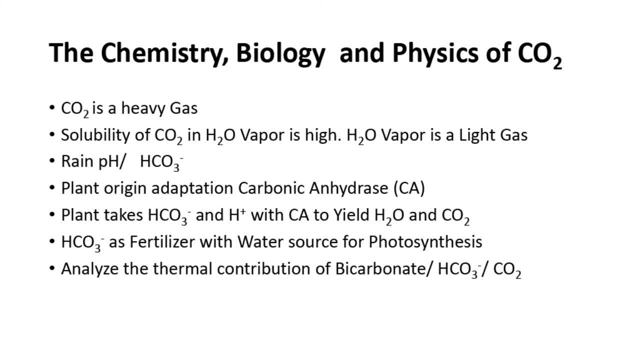 How do we know about what the CO2 is doing and where it is in the atmosphere? The rain, The pH of the rain, The CO2 of the rain has been changed- and we'll look at that- And it's made into a new substance between water and carbon dioxide. 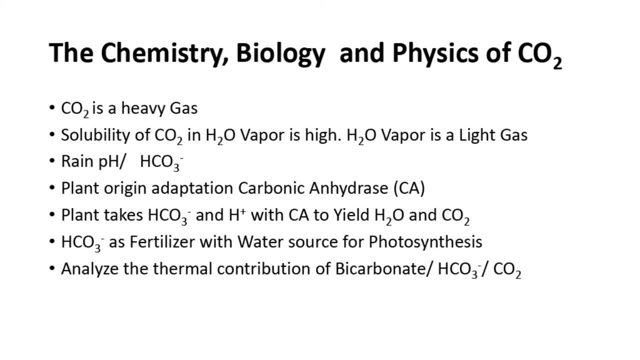 Plant origin and adaptation has involved a specific enzyme. It's called carbonic anhydrase. We'll discuss that in quite a bit of detail. The plant takes in these materials, That would be the carbonic acids- And it uses the aldehydes- sorry, the anhydrase- to break them down, to yield water and carbon dioxide to promote its own photosynthesis. 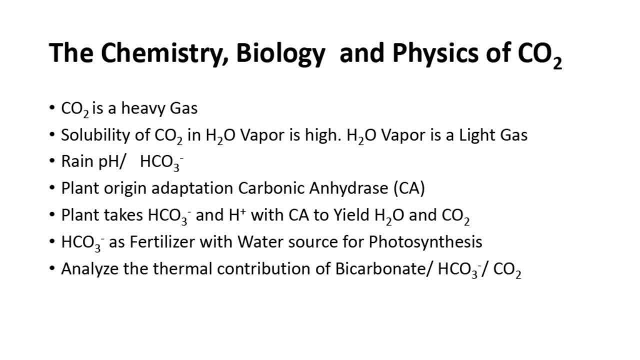 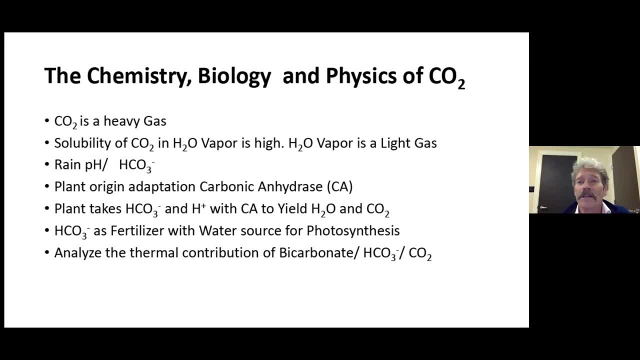 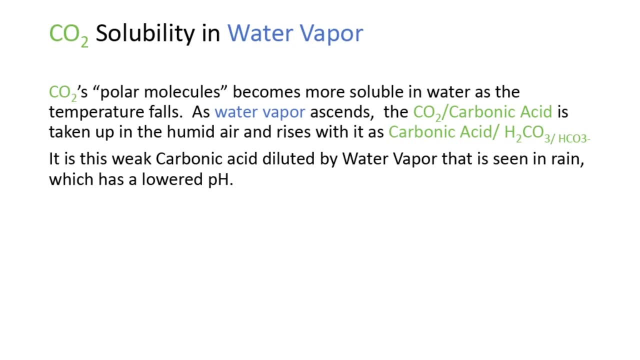 This would be the fertilizer for photosynthesis. So we've got to analyze all of these other new products now in the same way as the old ones have been. So solubility in water vapor CO2 has been changed. CO2 is a polar molecule. 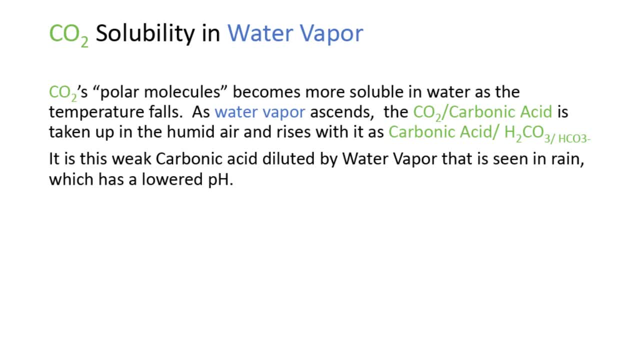 It becomes very soluble in water as temperature falls. As water vapor ascends, therefore, and temperature drops, the CO2 in the carbonic acid is taken up in the humid air and it rises with it. It's the weak carbonic acid diluted by the water vapor that we see as rain, which has a lowered pH. 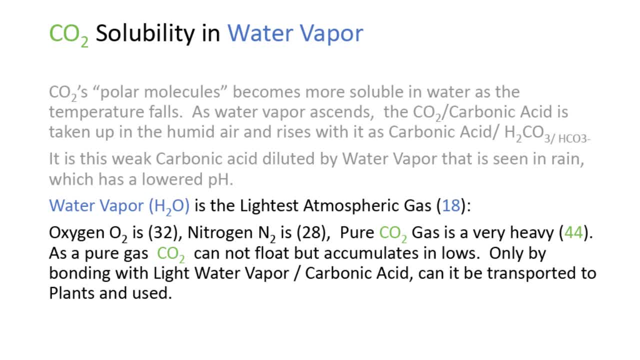 The water vapor is lightest, at 18.. Oxygen: Oxygen is 32.. Nitrogen is 28.. CO2 is the heaviest, at 44. As a pure gas, CO2 cannot float but accumulate in lows. only We don't see that. 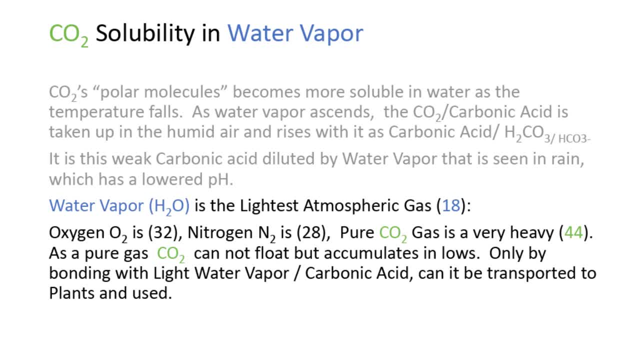 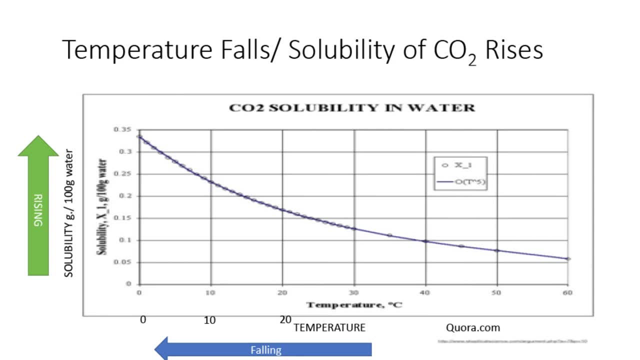 Only a bonding with light water vapor as carbonic acid can transport it to the plants to be used. This is the solubility curve. It's rising the solubility of CO2 in water as the temperature of that water is falling. 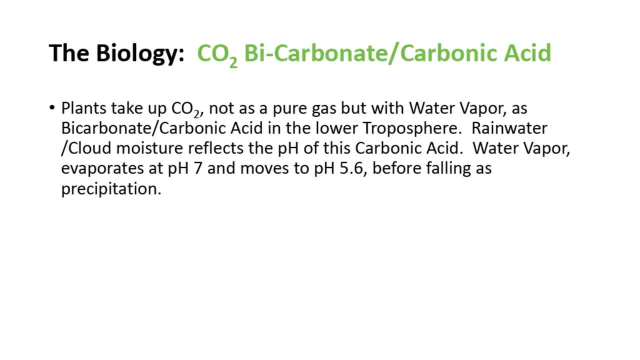 The biology of the system. The CO2 bicarbonate carbonic acid is what we want to discuss here. The plants take up the CO2, not as a pure gas, but with water vapor, as bicarbonate carbonic acid in the lower troposphere. 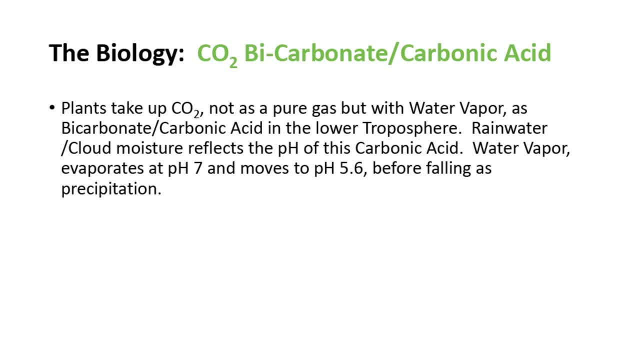 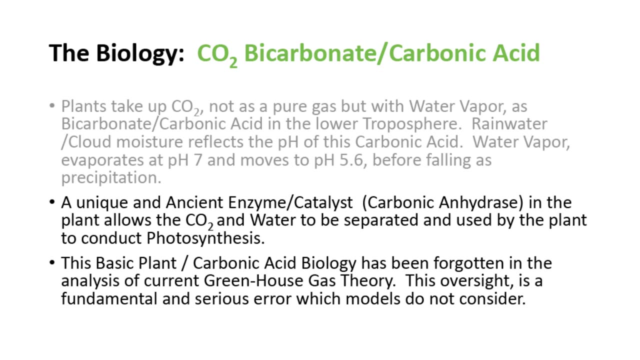 Rainwater, cloud, moisture and its pH reflects this. It moves from evaporation point at 7 pH. It moves to a slightly more acidic 5.6.. Before falling as precipitation, A unique and ancient enzyme, carbonic anhydrase, in the plant allows the CO2 in the water to be separated and used in the plant to conduct photosynthesis. 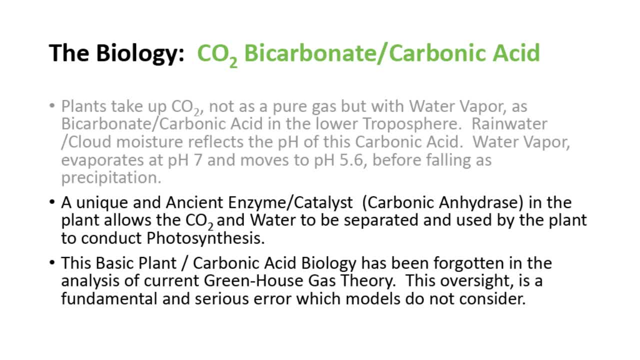 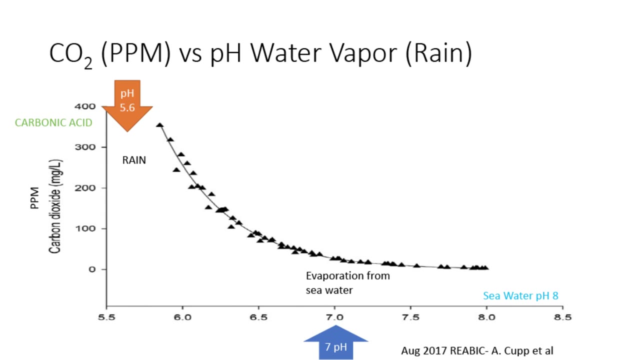 This basic plant, carbonic acid biology, has been forgotten in all of the analysis of the current greenhouse theory. This oversight is a fundamental and serious error Which models Do not consider. This is that rainwater CO2 in evaporated water makes it slightly from seawater at 8, slightly acidic to pH 7.. And then all the way up to 5.6 or so, where it rains out as carbonic acid, Carbonic anhydrase. It's a rapid acting and high volume catalyst Converting H2CO3 to water And carbon dioxide. 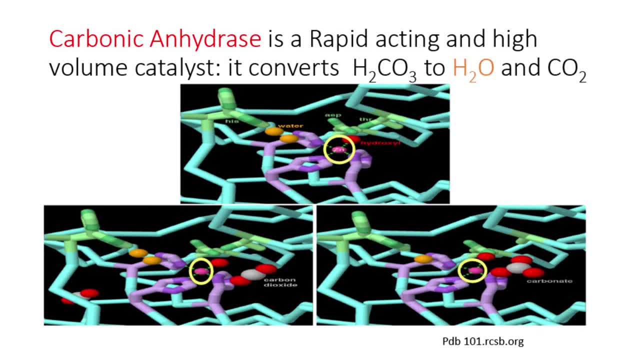 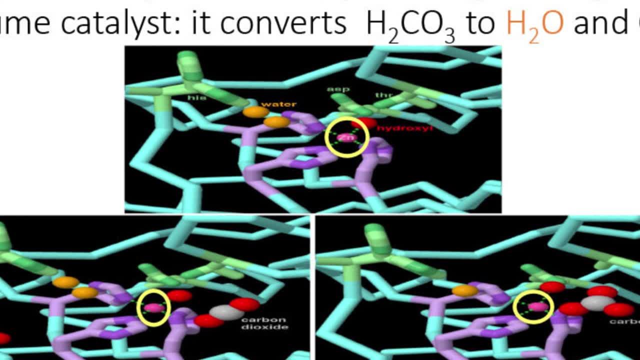 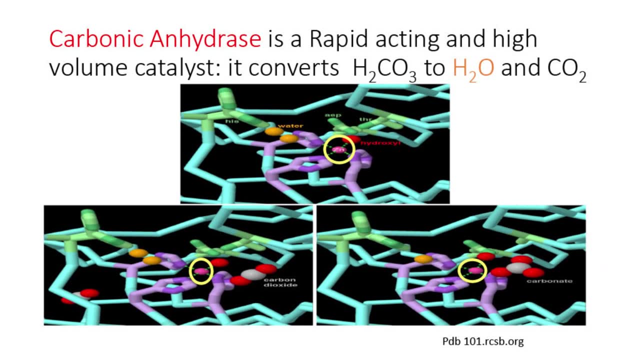 Which go on to become part of the photosynthetic system. This little guy here, the zinc in the middle, is the central element within this structure. These are proteins. These are enzymes. Now there are other areas in animals and in bacteria that use a slightly different version of this. 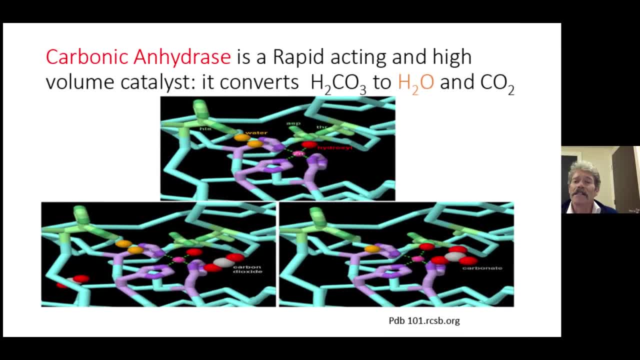 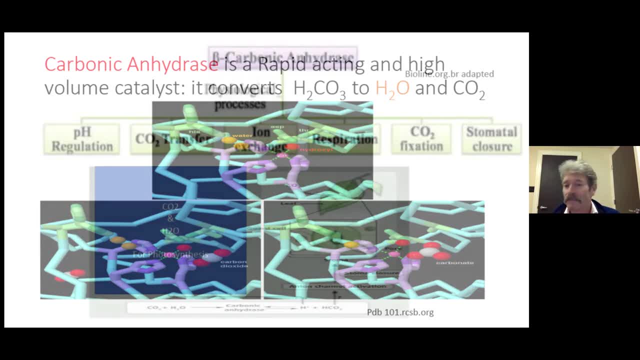 But all require it for life. In our human lungs it's responsible for life. It's responsible for rebalancing the carbonic acid in our blood And the removal of the CO2 from our bloodstream. This is the beta version of it, which is used in plants. 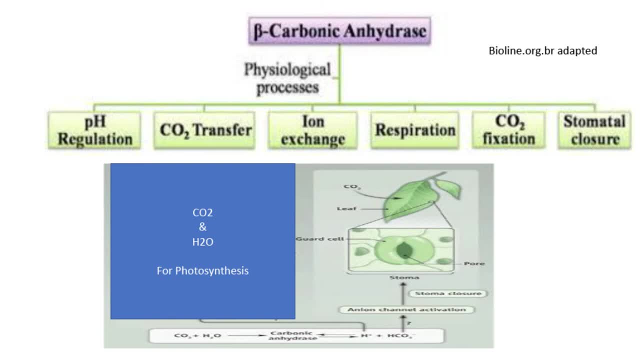 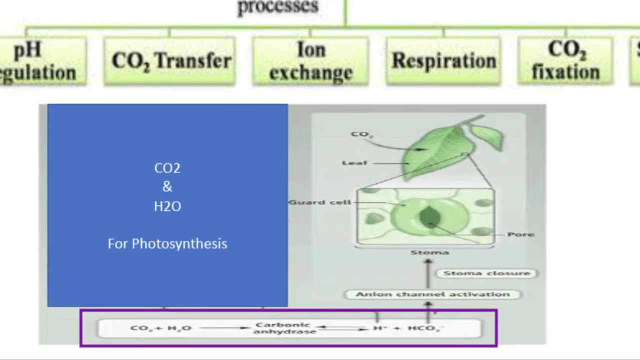 The plants do all of these things, of course, through their stoma, The closures or openings on their leaves. This formula down here is illustrating how this beta version sits in between carbon dioxide and water And hydrogen, Hydrogen ions and bicarbonate ions over here. 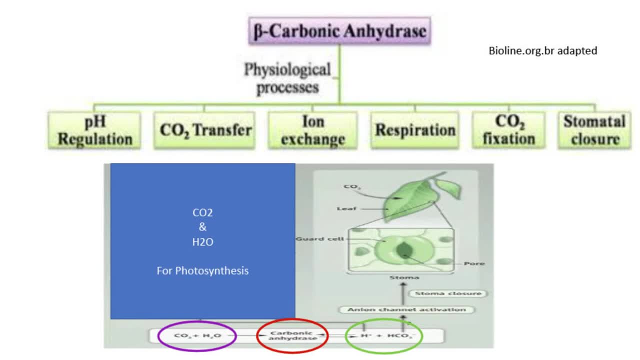 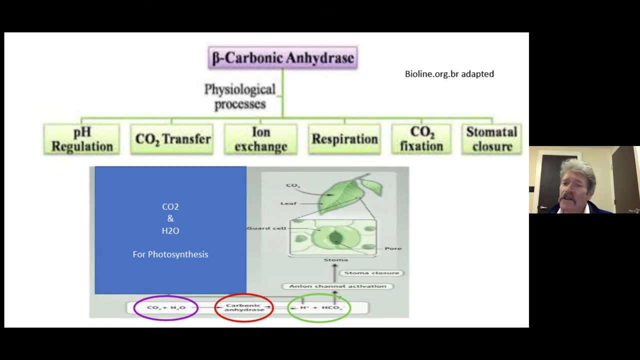 This is a part of the natural respiration cycle and transpiration cycle as well. in plants Under high altitude and colder conditions, carbonic acid cannot be easily delivered to the plant. This defines tree lines of latitude and on elevation of mountains on the earth. 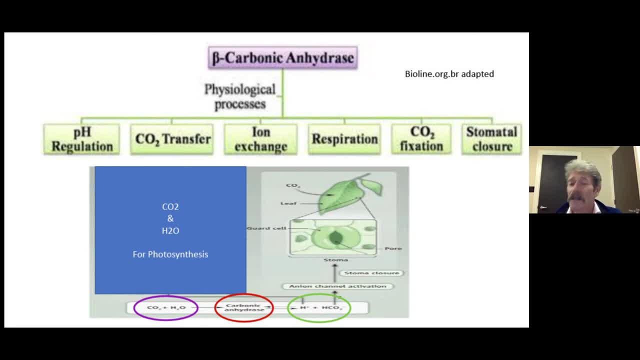 Tree growth rings show this moderation in the winter: Reduced growth based on lack of the delivery of CO2 and water in the winter. Nature would not have developed this catalyst if CO2 could be delivered directly as a pure gas. The whole process of pure CO2 induced global warming theory needs to be rethought. 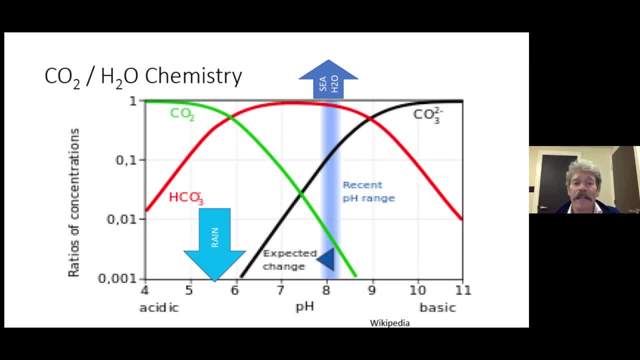 This is a complex diagram. It's got pH on the bottom here And the ratios of the various concentrations of CO2.. HCO3- And CO3-2.. We're going to deal with this portion here. This is where seawater would begin. 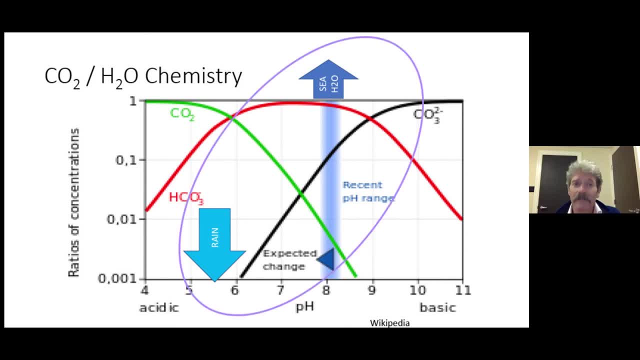 This is where rainwater would end. It's all under, really, the umbrella of, not CO2., But within the mid-range here, Where carbonic acids and bicarbonates dominate, 100% CO2. And CO3-2. And CO3-2.. 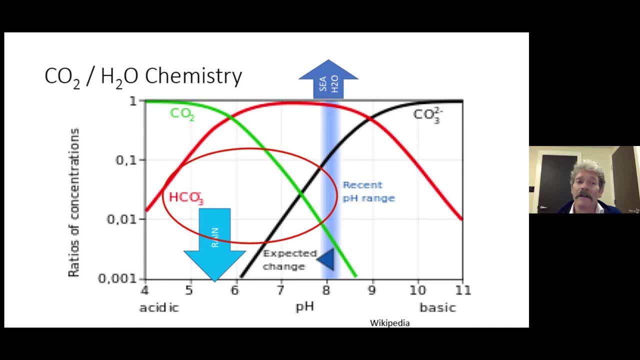 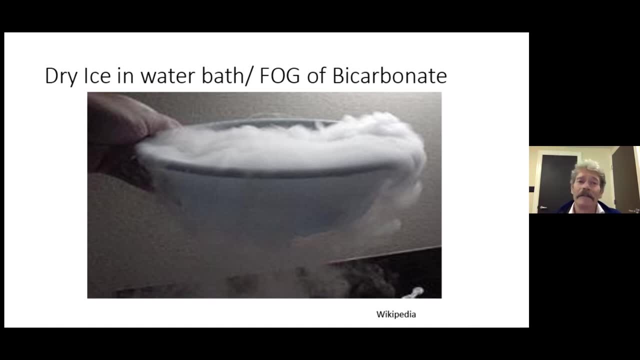 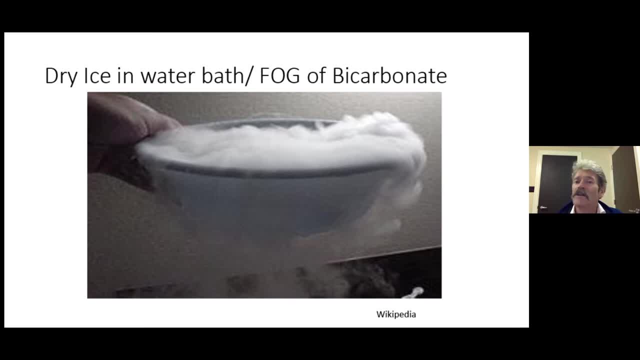 Warm water And we get a FOG, A bicarbonate FOG, Which comes off of this. So this is 100% CO2.. And it dissipates as carbonic acid bicarbonate In water vapor And rises with it from the bowl as a FOG cloud. 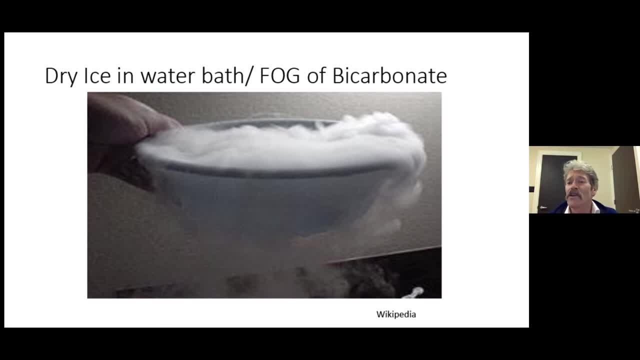 The cloud is trapped really by the worm err above it. Like an inversion being, The CO2 does not stay as a pure gas. When it is heated, the initial cold fog inversion of the bicarbonate holds together, But once it starts warming it dissipates into the atmosphere to rise. 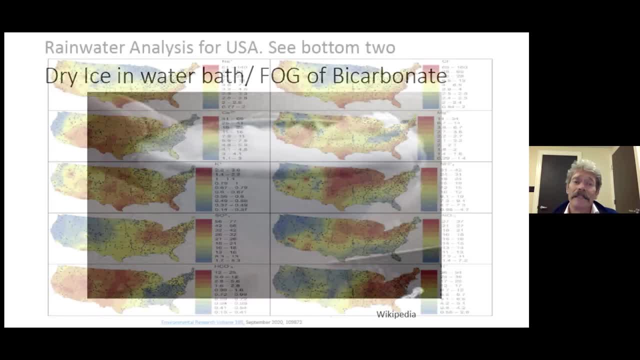 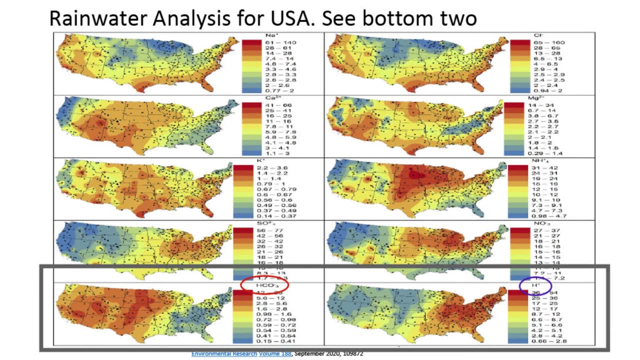 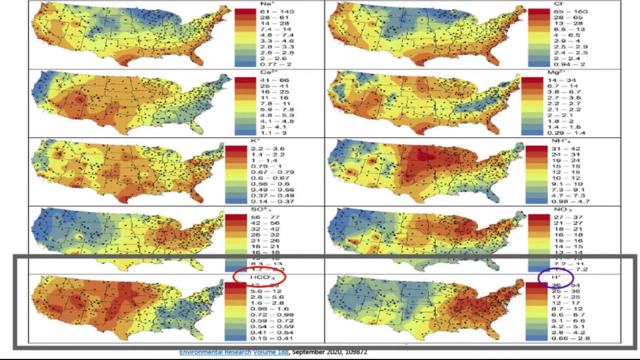 and to be carried as bicarbonate to plants. This is a rainfall analysis of the United States. These two lower portions. here are what they focused their attention on. This was HCO3 negative and hydrogen ion concentration pH of the rainwater, And that's what they showed here. 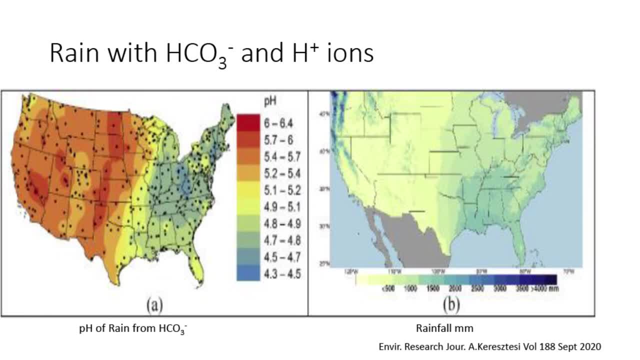 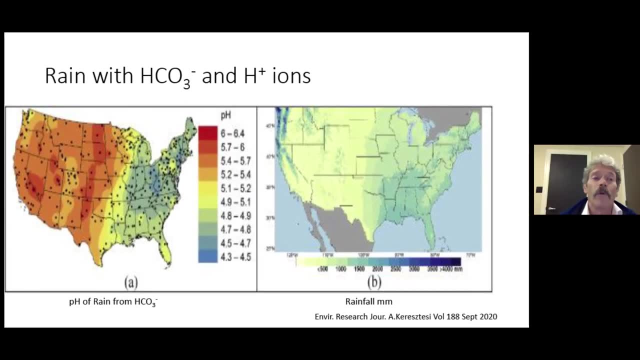 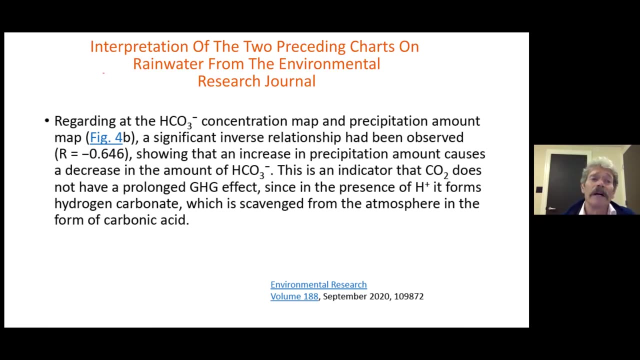 with hydrogen ion concentrations and rainwater in millimeters. Their concluding statement is rather important to us. Regarding the carbonic acid, or bicarbonate, concentration map and precipitation amount- figure 4b- a significant inverse relationship has been observed, showing that an increase in precipitation amount decreases. 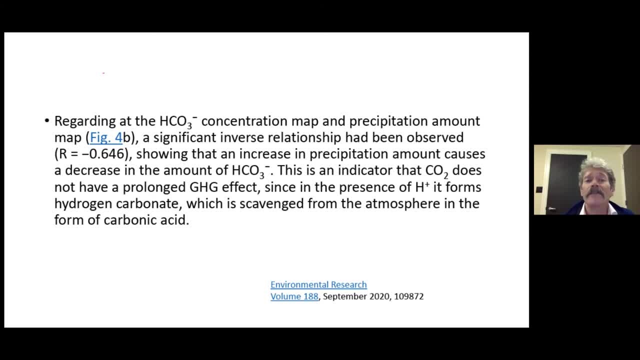 the amount of bicarbonate, And this is an indicator that CO2 does not have a prolonged greenhouse gas effect, since in the presence of hydrogen ions, it forms hydrogen carbonate, which is scavenged from the atmosphere into the atmosphere, And this is an indicator that CO2 does not have a 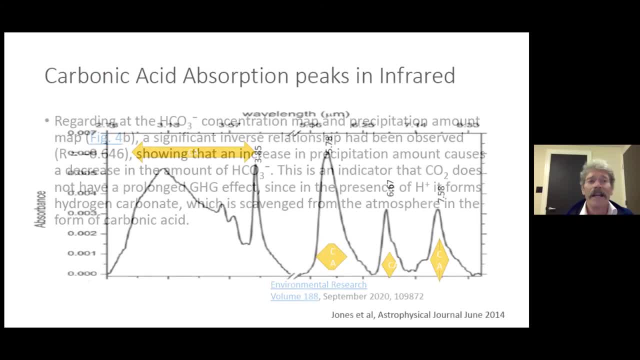 before. We can look at the PDF in a few minutes to see what it'll look like when we fá recipe is selected. So if CO2 enters the atmosphere, the perspective can be affected following dry와. So this is just aộtgybrush overview. 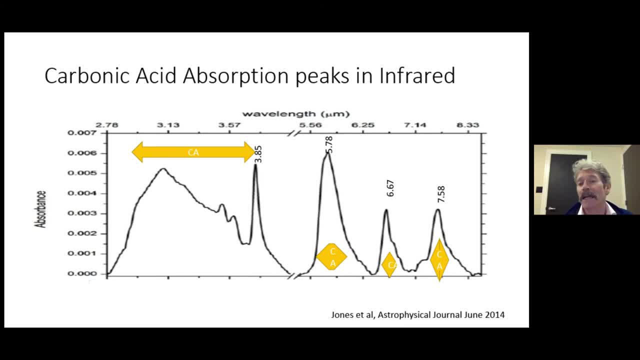 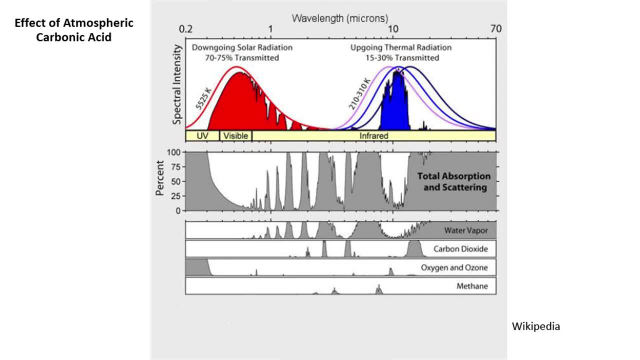 carbon, baked carbon seating we're going to transfer them into. if you remember, we had the co2 and the water and the methane and oxygen. here we have the earth glow and the solar glow. here there's where carbonic acid fits. the blue ones at the bottom, the three peaks, and then followed by the broadband here. 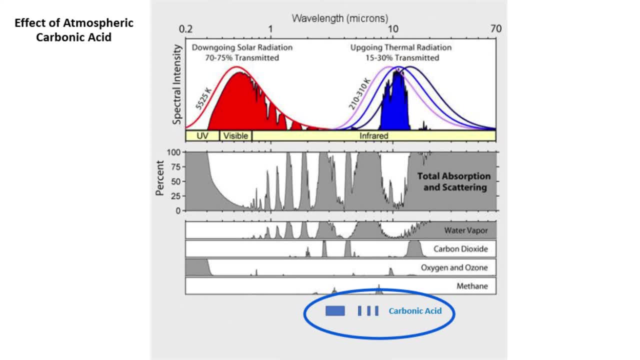 what's going on with them? what did they contribute, what are they doing to this radiation cycle in the atmosphere? here they're blocked, blocked firmly by water beyond the thermal radiation windows. these areas where earth glow and solar glow intersect, is where this sits, that broadband of carbonic acid. so carbonic acid does not attenuate the upgoing infrared radiation. 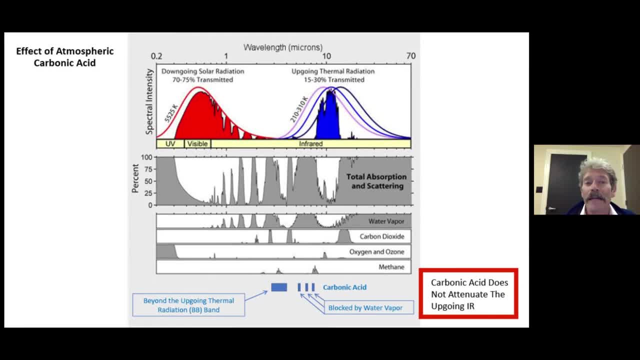 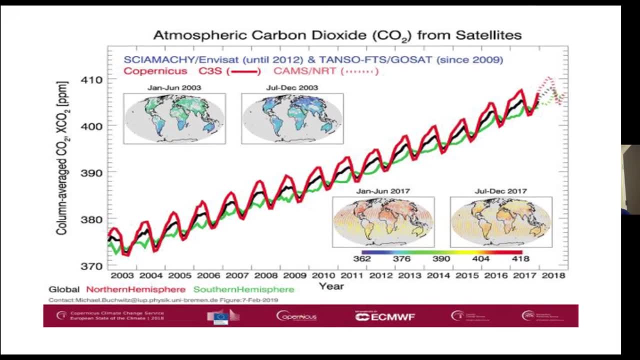 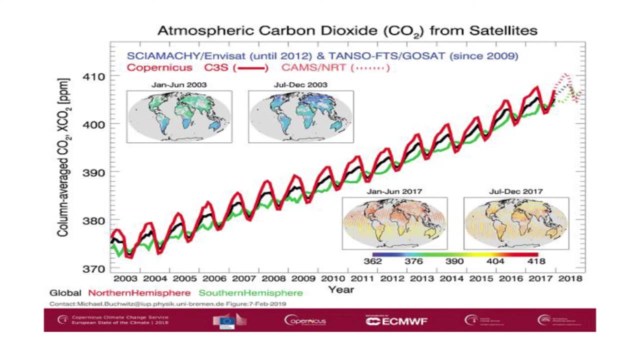 in any way. it doesn't contribute to a global warming. this is the graph of the climbing co2 as measured in the north and south hemispheres. north is red, south is green over the years. this was done by the european space group and this is the column of co2, or parts per million that would have been climbing steadily. 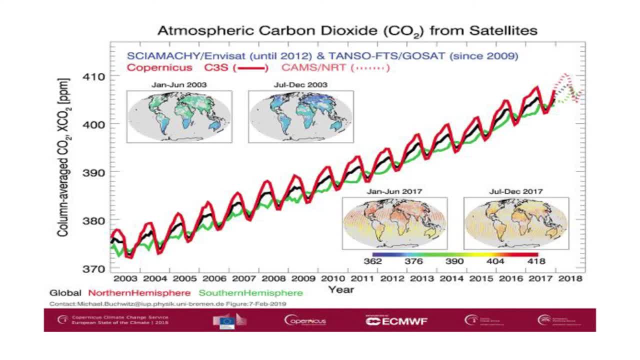 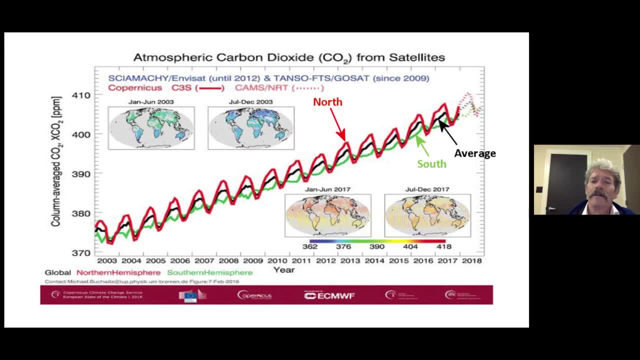 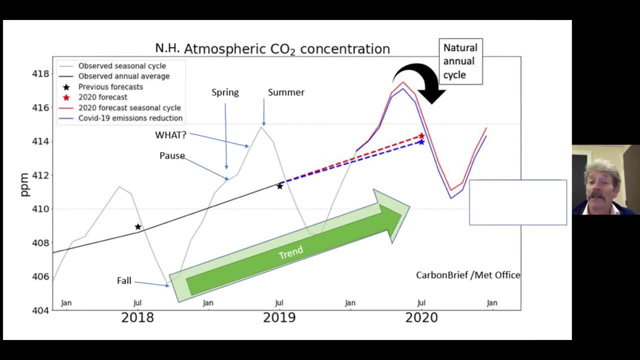 through that time. look at the difference between the southern hemisphere and the northern hemisphere. this is an average line, the black one in between. quite a remarkable change between those on a co2 basis. this is what it happens to look like when you blow it up a bit. 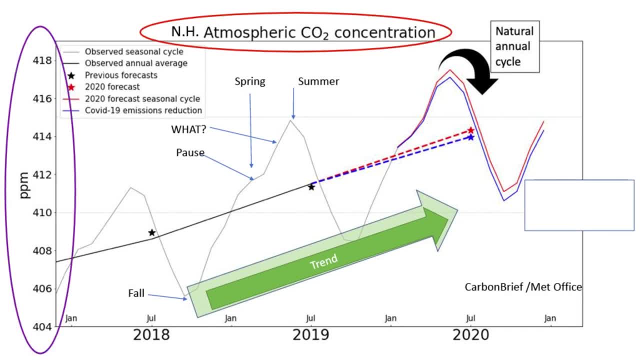 this is the northern hemisphere co2 concentration. over here and these are the years involved, we go through a fall rise, when all the leaves have died off, to a rising co2 concentration, which has CO2 to a pause, a very strange pause in the spring, But that is the beginning of the cycle of 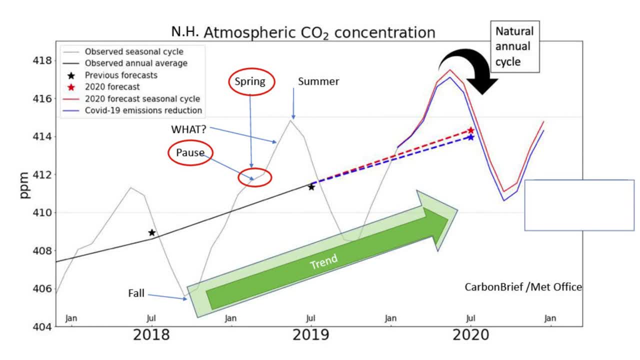 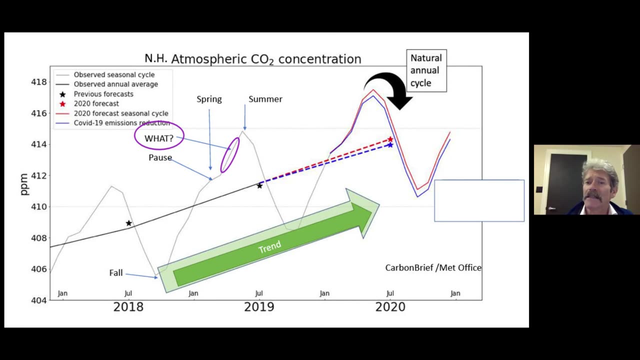 absorbing of CO2,, in this particular case, carbonic acid, from the atmosphere. But there's another rise, a second one which happens up into the summer period. What is happening in there? This is important to resolve. It's what's happening near the poles, This process of CO2 blooming. 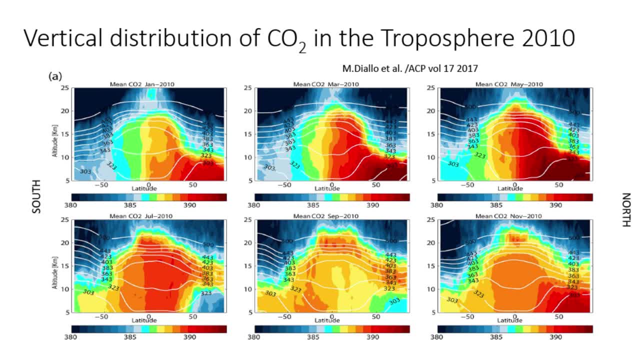 begins in the northern hemisphere winter. Back down here we're dealing with November, And it pushes to the top of the troposphere as we go to January. So we have to go across here from November to January. It then rises as a wall up the edge of the tropopause. 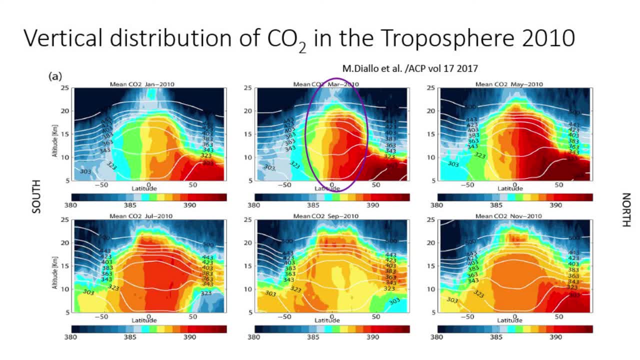 If you remember the shape, and that was the sudden step in the tropopause, And that was the sudden step in the tropopause, And that was the sudden step in the tropopause. right here, This is using CO2 as a tracer of where energy is moving and air masses. 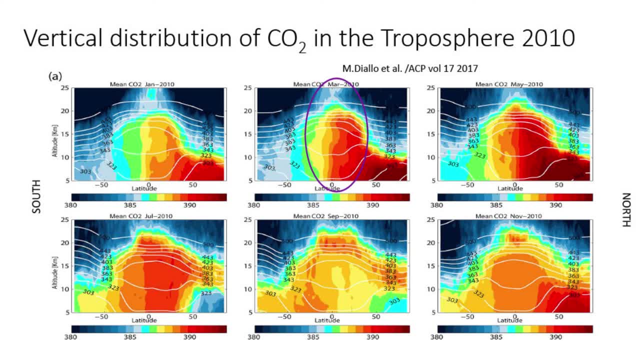 are moving. It's going from the polar areas up through there. But what's happening here? We have something else going on. In July, the northern hemispheric vegetation eats away at and diminishes the amount of CO2 that's in the atmosphere, And that's what's happening here. 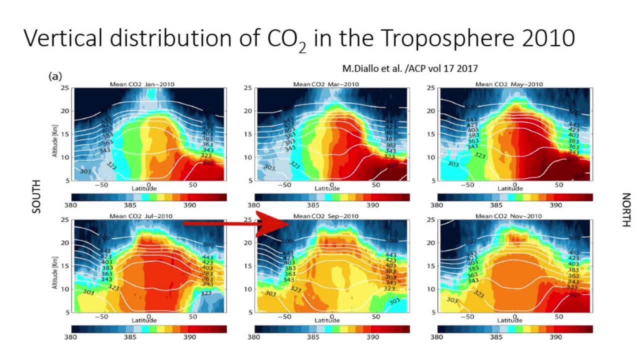 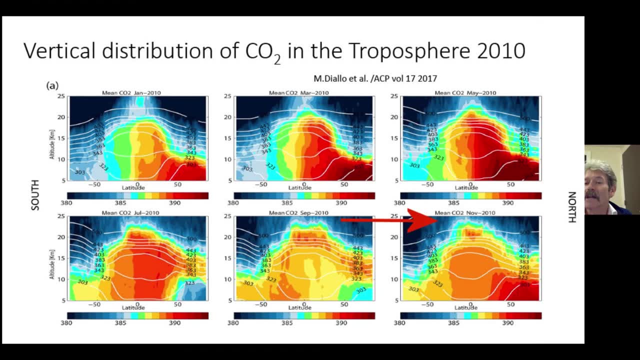 We have something else going on. In July, the northern hemispheric vegetation eats away at of CO2 in the atmosphere. That continues right through September, at which point we then revert again to the same seasonal up and down cycles. That's a CO2 tracer. These are the stations. 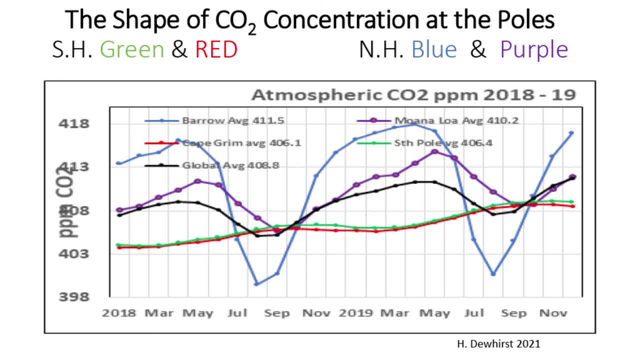 on the earth that fellow of Howard Dewhurst is showing in this graphic. The discrepancy between the poles is what he's most interested in, But using CO2 as that tracer, he shows Barrow Alaska here in the blue, with this huge up and down cycle versus what's happening here in the south. 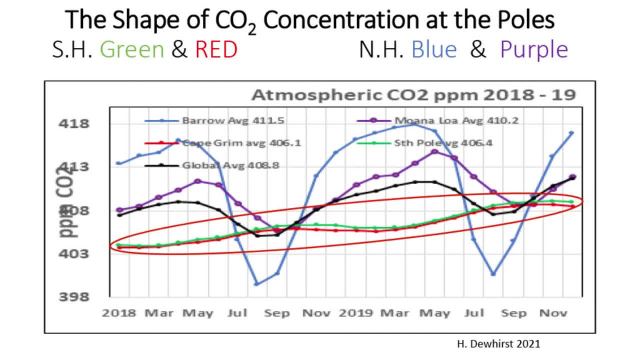 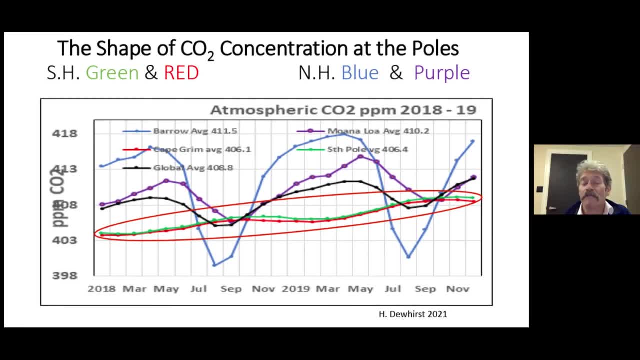 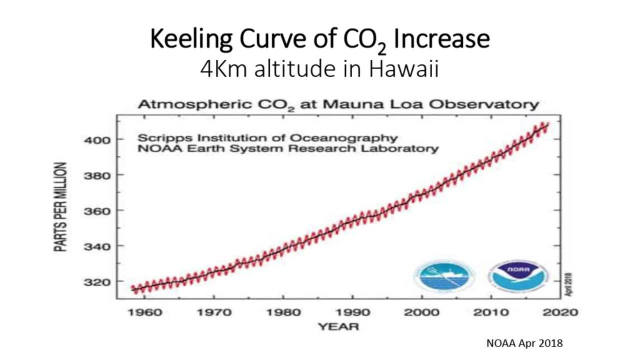 of the equator areas. This would be in Tasmania and in Antarctica. The southern hemisphere doesn't show extreme spikes at all. This is the normal curve, This one from high up on the island of Hawaii at four kilometers. The northern hemisphere is showing extreme spikes at Monoloa, the observatory looking at CO2,. 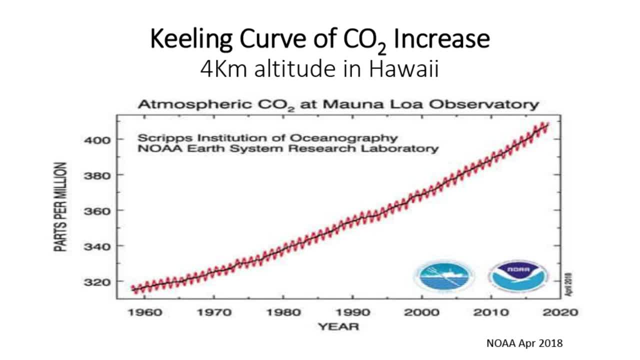 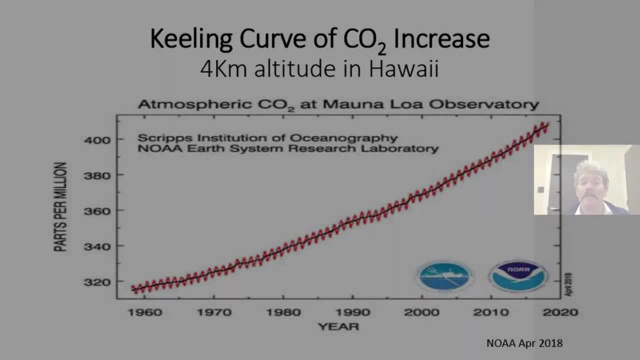 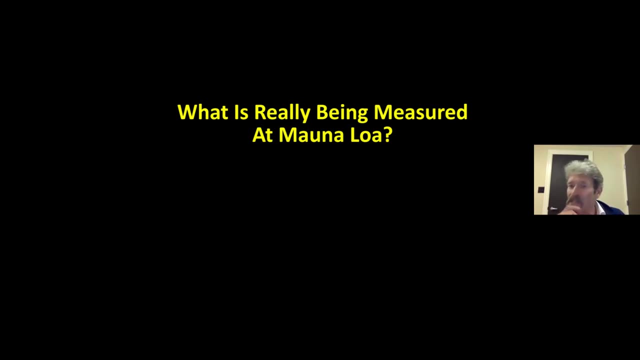 atmospheric CO2.. It's being studied there by Scripps and a fellow by the name of Keeley over many years, from the 1960s through till now. But what are we really looking at? What are we really measuring here at high altitude, in light of what we just discussed in terms of 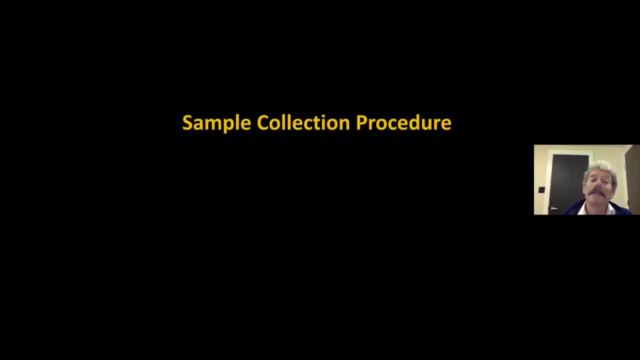 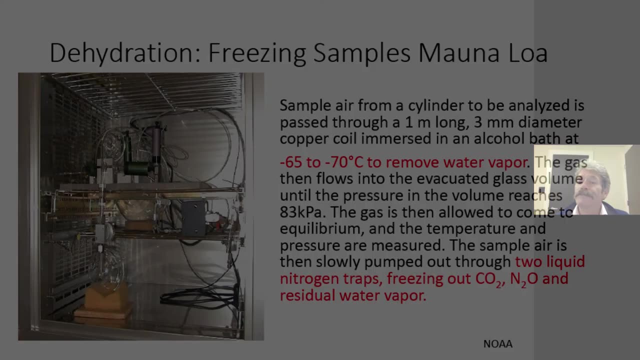 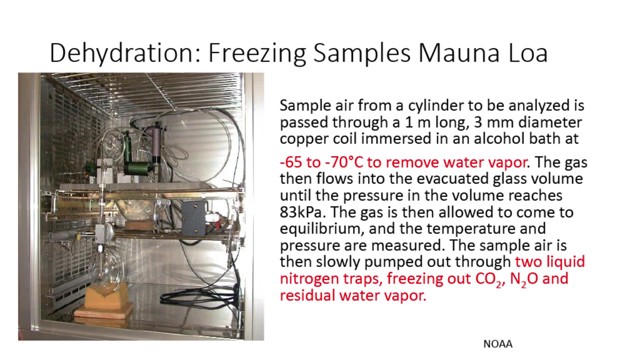 carbonic acid. How do they get their pure carbon dioxide to analyze? It has to be pure. So what do they do To accurately estimate the CO2 in the air samples? the process is described: It is separated and frozen to break it apart from water vapor. that 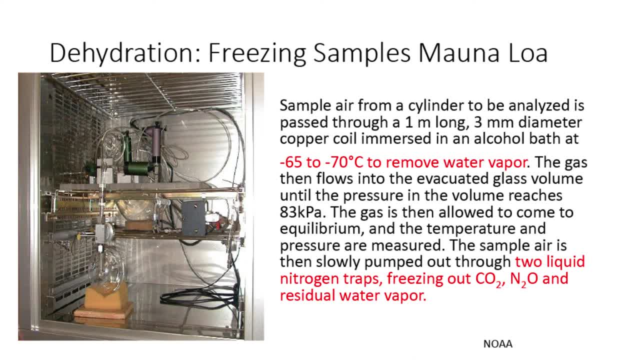 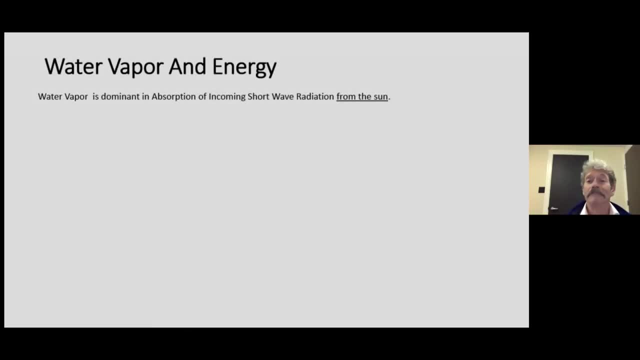 holds it and brought it there. Was it really carbonic acid? It seems that what we are measuring is likely carbonic acid and bicarbonate, not pure CO2.. The greenhouse implications of this are very meaningful. So how do they get their pure carbon dioxide to be that water vapor and energy? 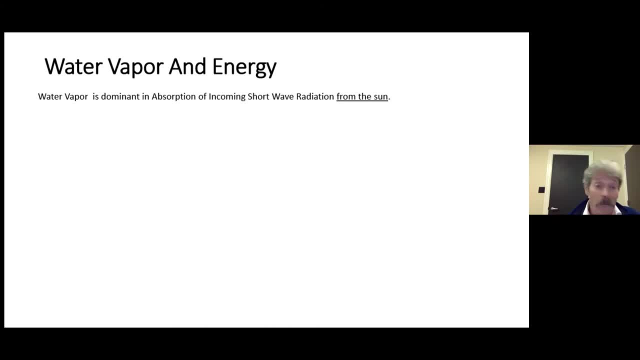 So if it isn't the CO2, is it the water vapor? Is that the thing that is managing to warm us more than what we had anticipated by some of these models that we have been talking about earlier? So under short-wave radiation from the sun? 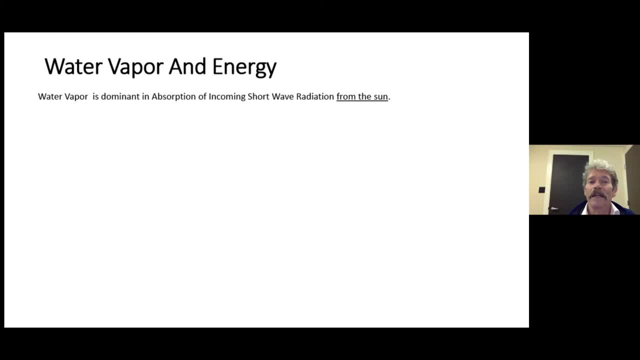 the solar glow of that incoming radiation. This has been underplayed in many of the models Under long-wave radiation from the Earth. water vapor is also the most important greenhouse gas in the atmosphere. Outgoing heat radiated from the Earth's surface is absorbed by water vapor molecules in the 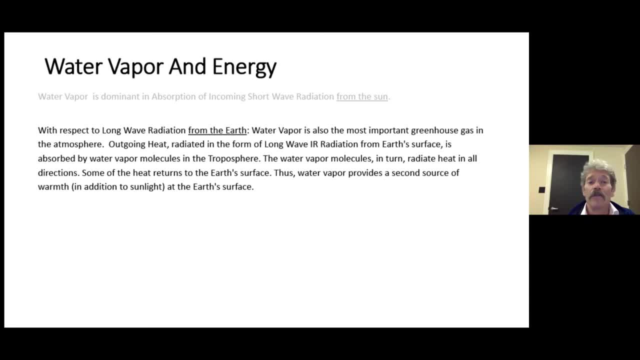 troposphere. The water vapor molecules in turn radiate, re-radiate this heat in all directions. Some of it returns to the Earth's surface, and this is what we see as heat retention, to allow us to not be in the cold of space, the cold equivalent of no atmosphere, Planets with condensable gases. 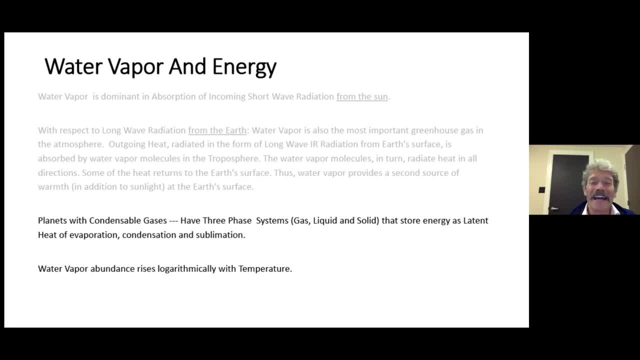 all planets of this nature that we know about have three phases: gas, liquid and solid. That's what we have here on Earth. CO2 does not have those characteristics here in any way. These stores of CO2 are in the atmosphere. They're in the atmosphere. They're in the atmosphere. 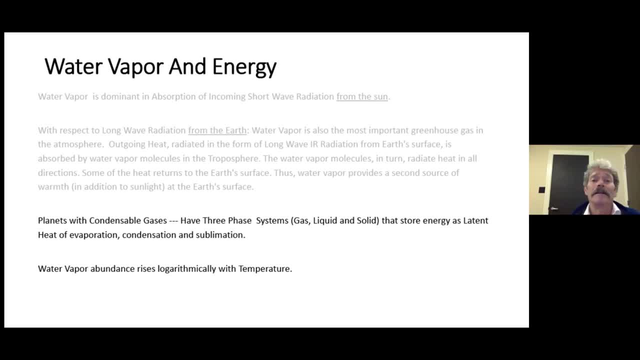 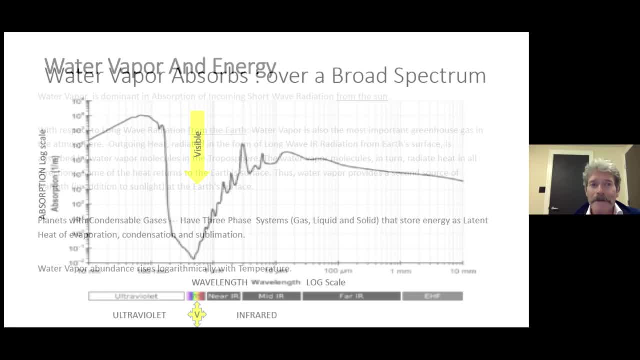 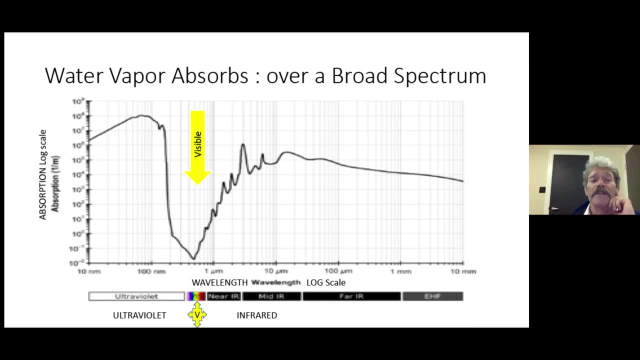 rises logarithmically with temperature. This is the spectrum of absorption of water vapor, what it absorbs over the broad spectrum here of microns. This is a log scale, little different than the last one, compressing a lot into it. We looked at 15 here before We also 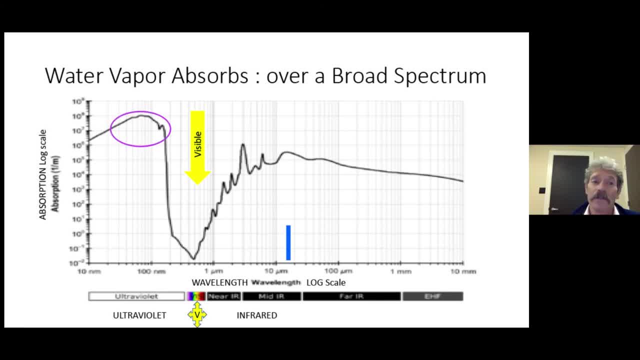 see a large bulge here related to absorption in the ultraviolet. This is the vert, this area. here the V is the visible spectrum. This is why water vapor is invisible to us. It's the most energetic. It doesn't absorb as much within the visible wavelengths Water. 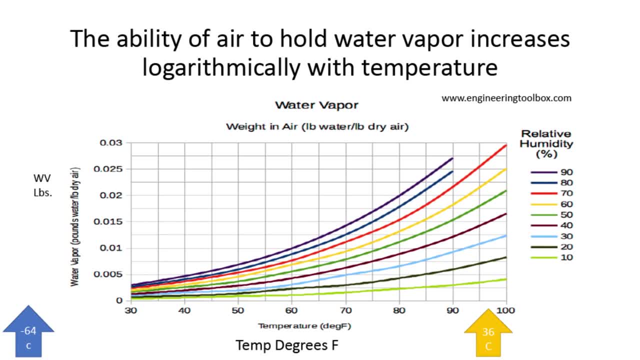 content in the air. pounds of water vapor rise dramatically with temperature, depending upon the relative humidity. Relative humidity is something we won't really dwell on too much, but what we're dealing with is a logarithmic rise of water within the air, The amount of water being 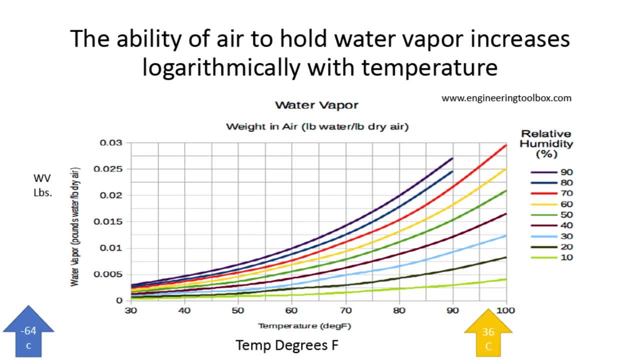 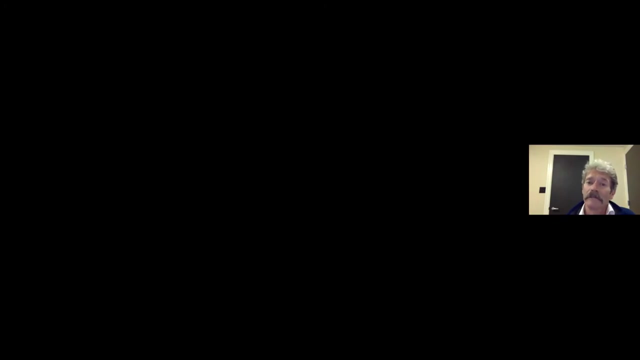 held in the air is dramatically rising. Therefore, that changes everything about the equation of how water vapor acts to preserve and to hold energy in the atmosphere and rain it back down to the earth. Abundance of water vapor thus determines the absorption rate of that energy. This is a 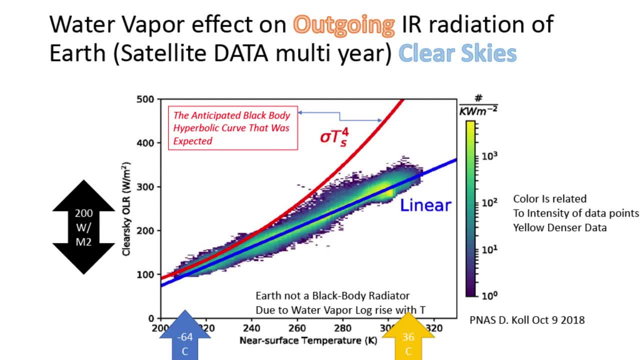 satellite study. It was done in 2018 or compiled then, but done over many years before that. from data that was accumulated, It looked at the outgoing radiation and it's all satellite data. It's multi-year and it was done in clear skies, So that was meaning. 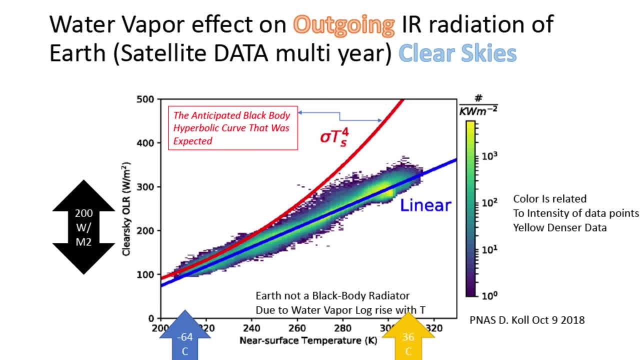 there were no clouds to actually inhibit what was being looked at in any way. The color intensity here within this band, is how many data points there were to look at. What the conclusion is from this of outgoing radiation in watts per meter squared over temperature in degrees? 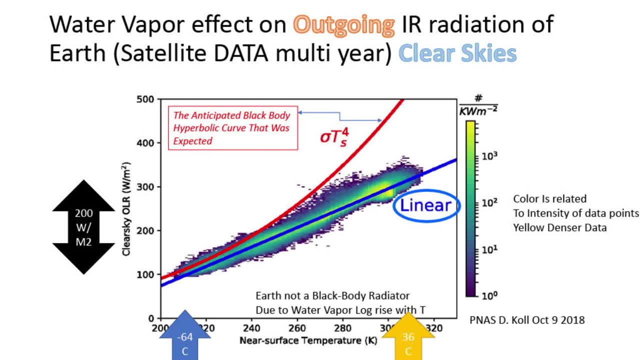 we're looking at a linear relationship. This was unanticipated. This was not expected. It was supposed to be a hyperbolic curve here. that was anticipated. What was going on here? According to the authors, the log curve of humidity minus the log curve of black body. 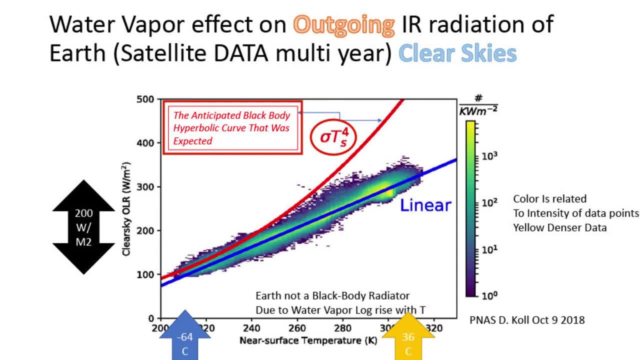 radiation results in a linear trend. The outgoing long wave radiation responds directly, linearly, to temperature. Thus, thermal radiation from the earth is controlled by water. That's why we're talking about a linear relationship here. So this is a linear relationship. This is a linear relationship. This is a linear relationship. 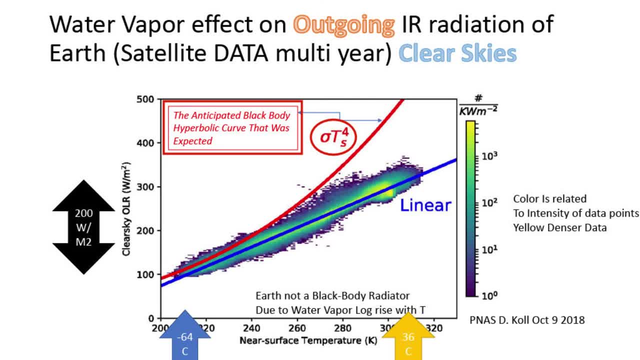 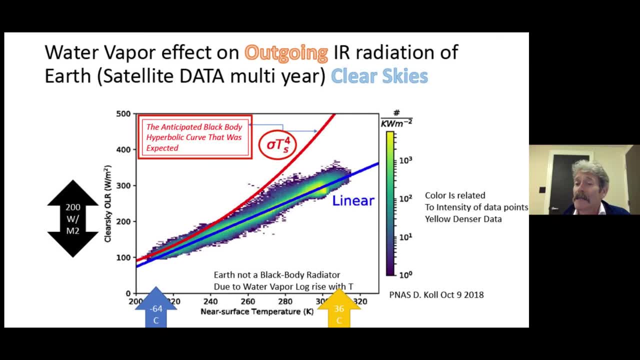 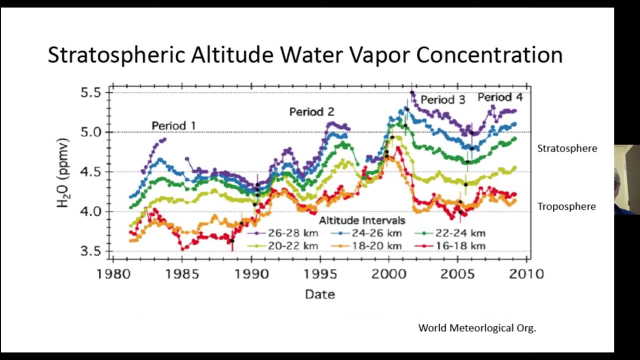 water vapor, not CO2.. There is no radiation energy fingerprint being detected directly from CO2 molecules in this satellite data, only water vapor, radiant energy. Weather balloons and work of that sort have corroborated this from 1980 to 2010,, and this one at various parts of the upper 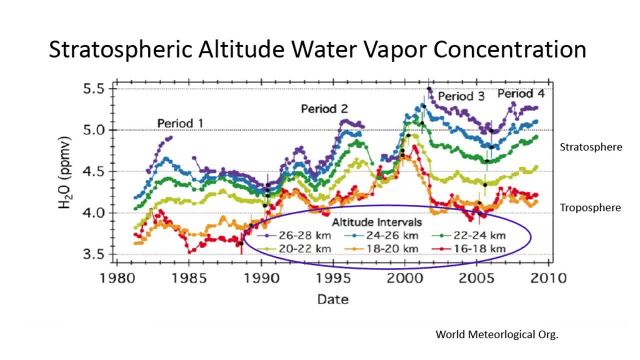 troposphere. We're dealing with these heights in kilometers, in different colors. The troposphere is about here in elevation generally and the stratosphere higher slightly. These show the parts per million of water. It's climbing. It's climbing in steps. It's jagged, It's not uniform. 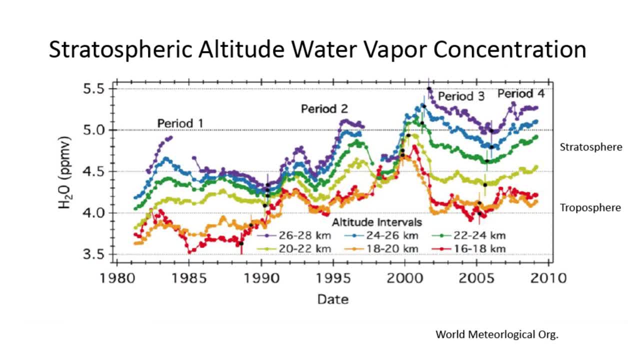 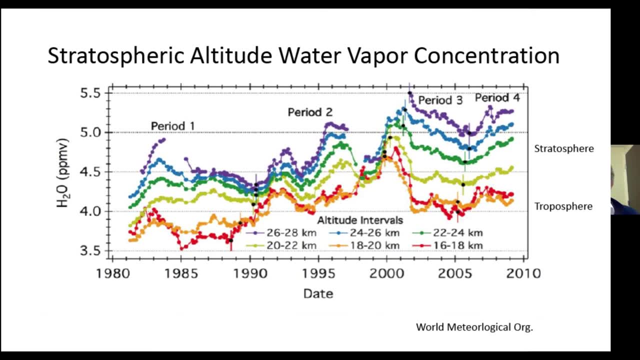 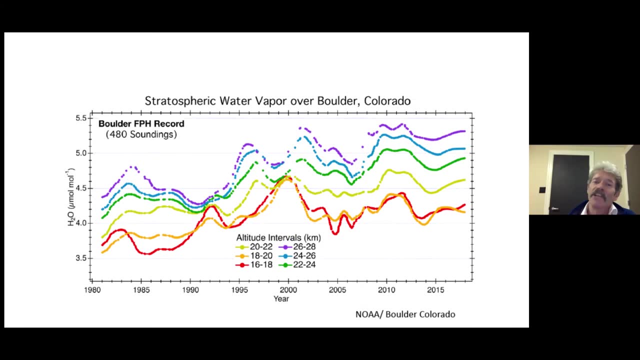 It's stacked and all of the elevation is in the stratosphere- Are responding together. It's pulsating in stages, rising and falling, and not reacting as we might have expected if it were due to an evenly distributed gas. Here's a continuation. 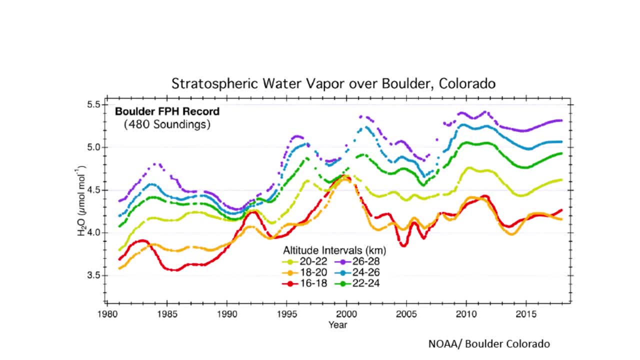 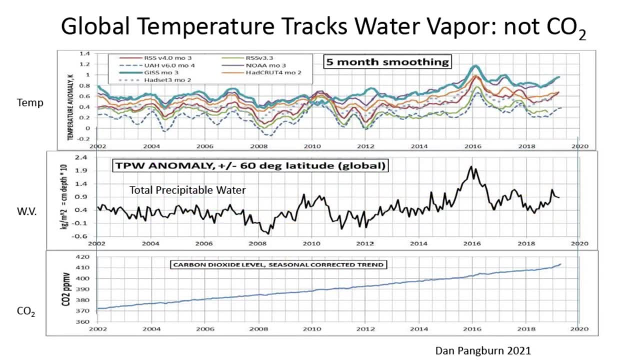 of that to add some more years from 2010 through to 18, showing the same kind of progression at all levels. Here's a conclusion by Dan in 2021.. He's looked at the water vapor readings that we just looked at, shown them here as a black line. 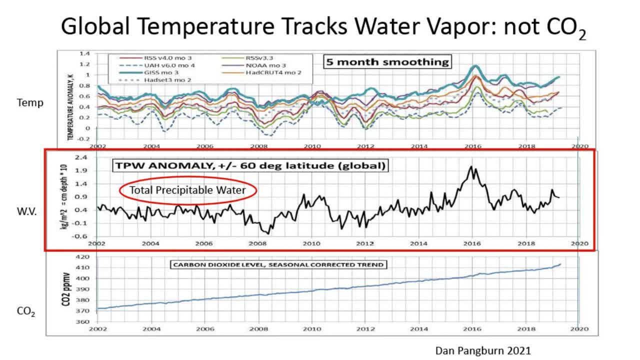 calling it total precipitable water, In that he has actually gone ahead and then compared that to, at the top, the temperature, as many different groups have estimated it around the world. These are the groups that did it: NOAA and headset and et cetera, et cetera. All of these are showing. 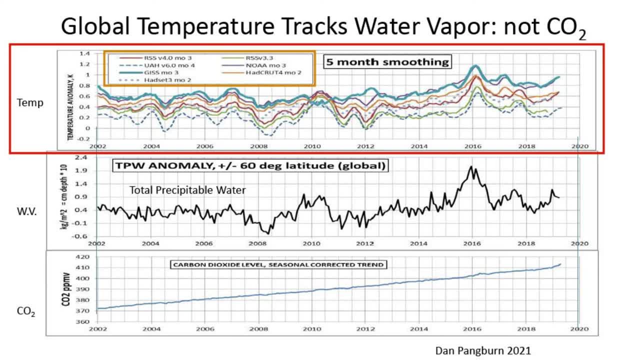 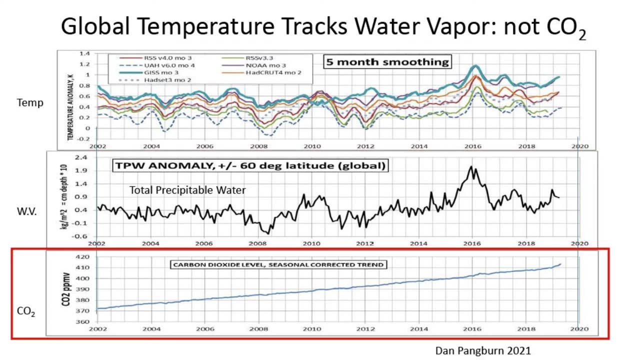 variations, some of them more extreme than others, All of them in the extreme areas, are showing a coincidence- a remarkable coincidence- with the total precipitable water. as we've been looking at, This is the carbon dioxide rising trend that we looked at from the Keeling work. 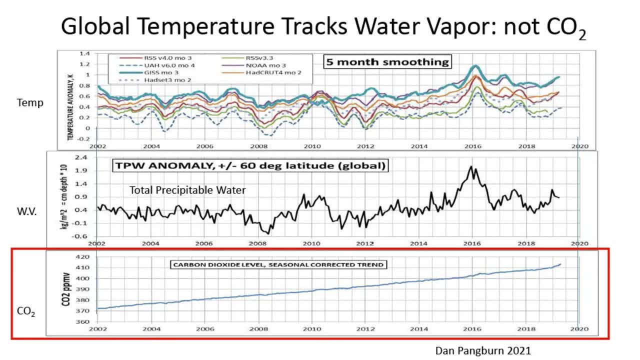 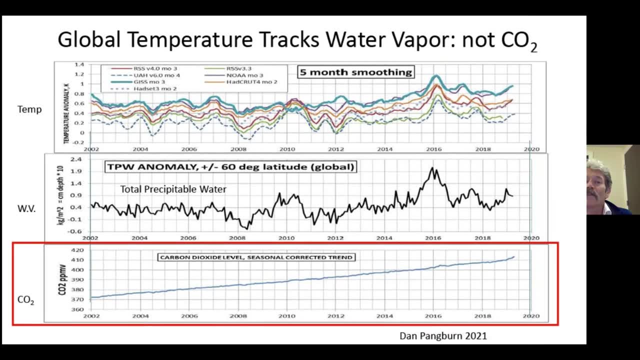 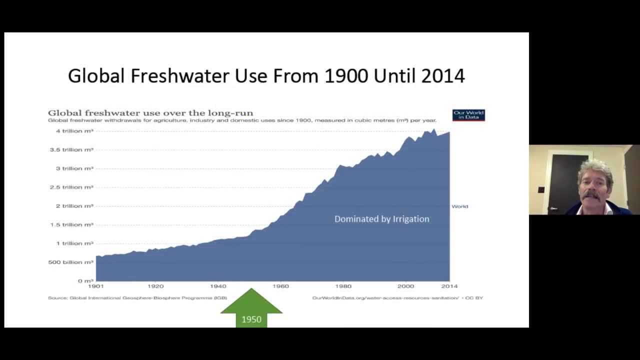 carried right through to 2019.. It is not varying in that same sense. It is not correlative in the same sense as what we're getting here between water vapor. Why? What's going on? What's special about that? Well, Dan has a feeling that we're also being dominated by excess water. that's being 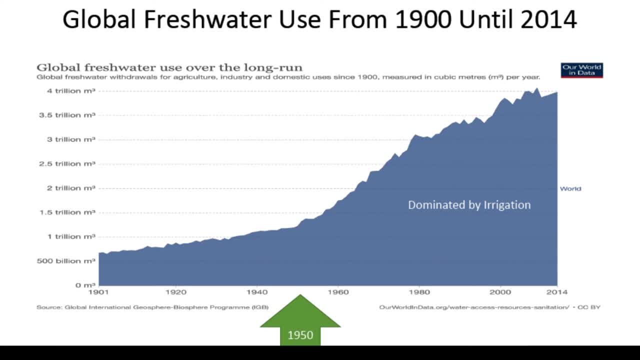 put into the upper atmosphere. That water can be sourced, he feels, from this irrigation water. Taking water and putting it into irrigation worldwide from 1950 or so has created a a tremendous bloom in the amount of water vapor available to the atmosphere. the total 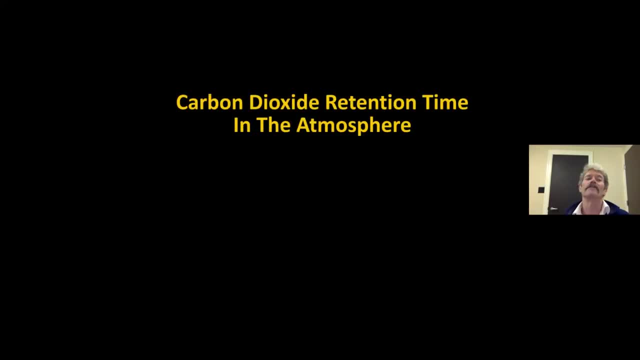 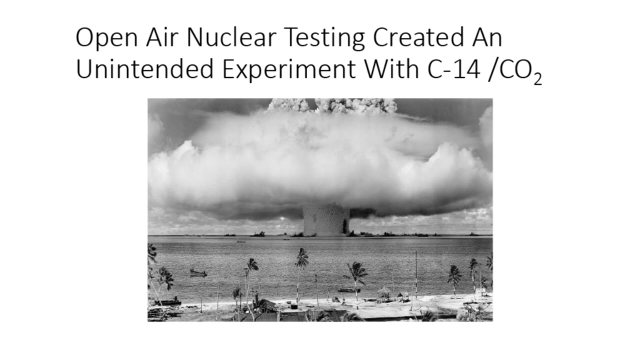 precipitable water. I want to talk about CO2 now for a little bit again. What is the real retention time of CO2 in the atmosphere? This is a strange diagram to put up, but what it is showing is a big open air experiment that was unintended. 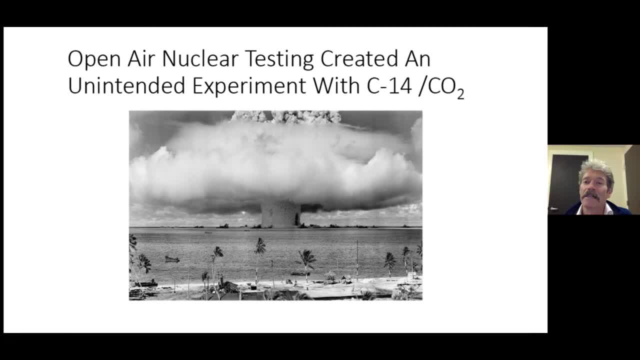 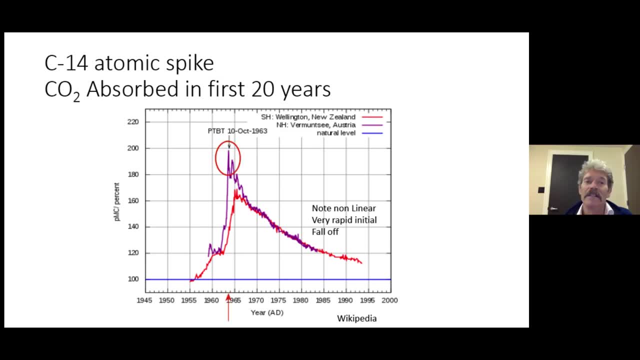 using carbon and carbon 14 in this particular case. What did it tell us about carbon? This is the atomic spike that resulted from all of those explosions. this is when the test band treaty kicked into place and stopped all further open air testing. rapidly, the curve plunged as a normal. 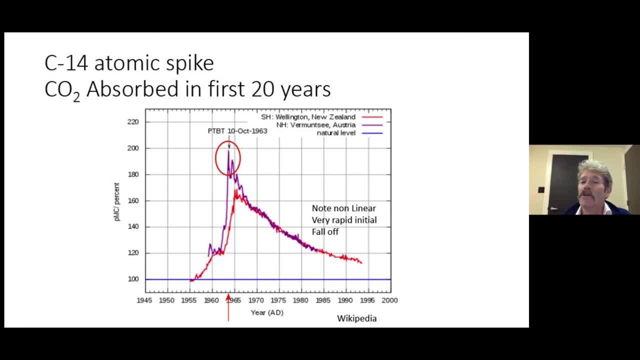 decay curve will within a natural system. we learned several things from these lessons about co2. the abundance of co2 determines the absorption rate and falls in a logarithmic decline curve toward a natural base level. the residence time of co2 in the atmosphere is far shorter than any. 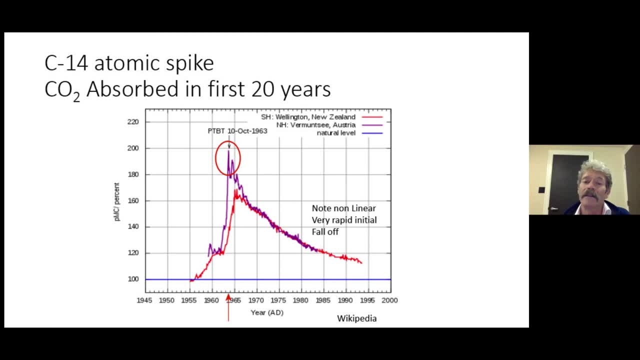 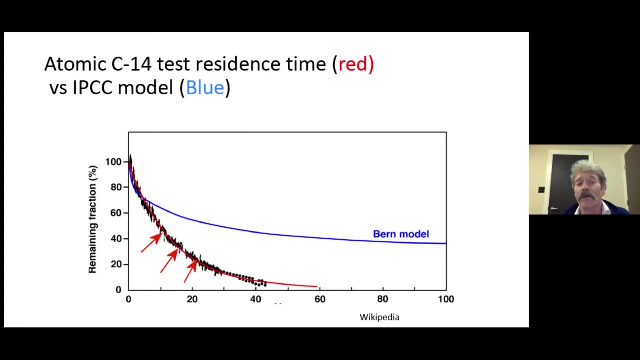 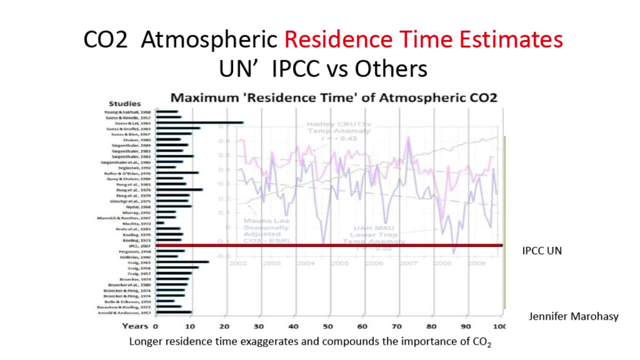 model builders and ipcc have tried to convince the public of. these are the two models. this would be what the ipcc uses, the burn model in blue. these are what those atomic results show, the carbon 14 results. the ipcc residence time as a result in the atmosphere is shown as a red bar. 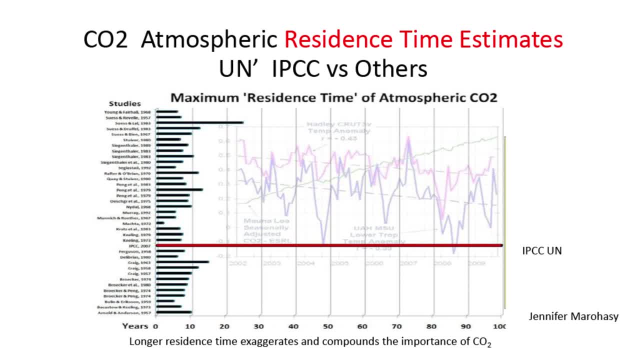 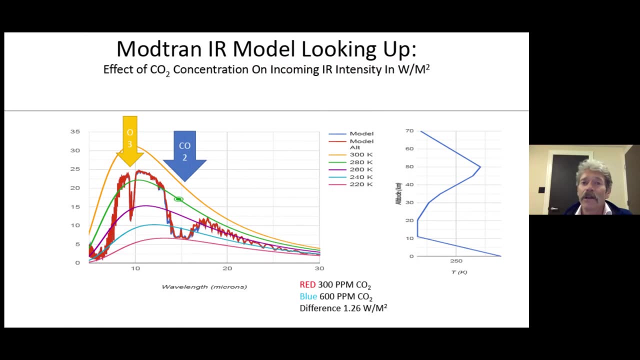 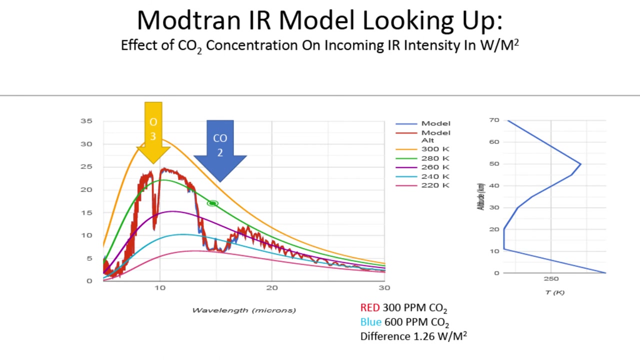 and grossly exaggerates what is shown by many other researchers and many other studies here in the black bars. why would the ipcc make this assumption in face of all the the rest of this data? i don't have the answer. we're going to look now at a model which is called mudtran um. it's a way of looking at the co2 and in this particular 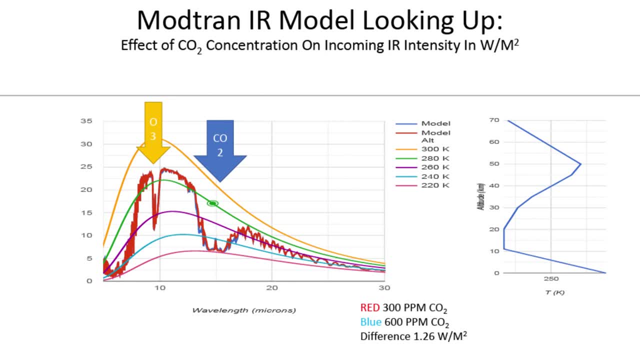 case also the o3 and the water vapor and how they influence the radiation that's coming back up from the earth and also the shock wave effect, that is, the co2 nitrogen emission of the carbon elements surface, the stuff that's supposed to be trapped. Here's a way of calculating that which is model. 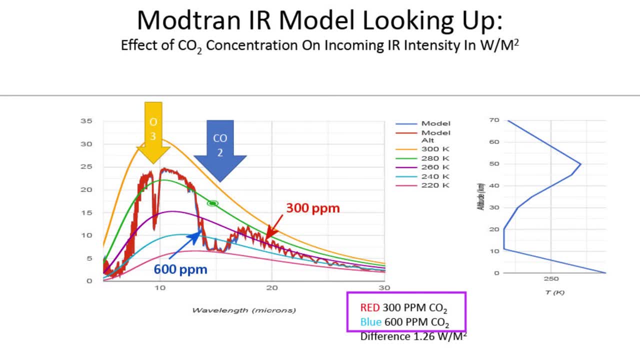 based. If we look at the difference here that's shown on the bottom, we may or may not be able to see the difference between the lines. The red line is 300 ppm CO2.. The blue line is 600 ppm. The difference between those in watts per square meter is very small, Very small, especially in 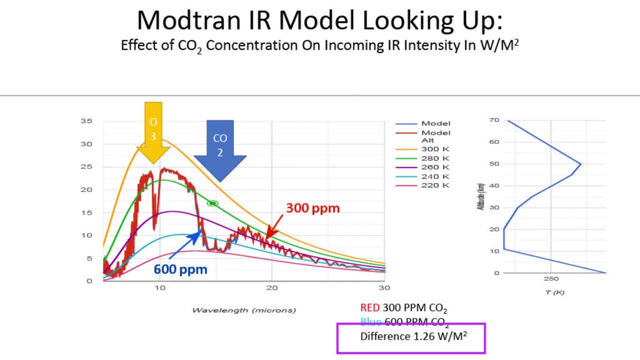 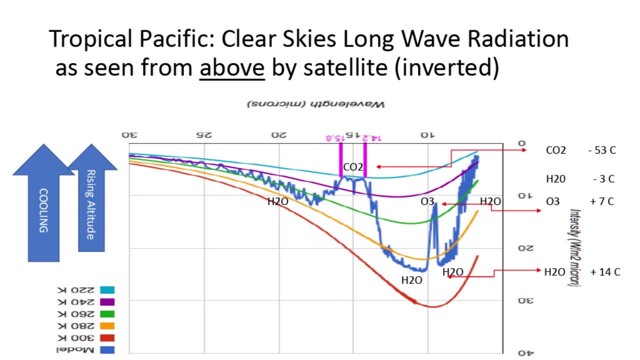 terms of the error limits, which we had discussed earlier, which exist in any model, And all of these models have very large error limits within them and assumptions. Let's take a look at the inverted image, or an equivalent image. This is a real one from the mid-Pacific area. You want to? 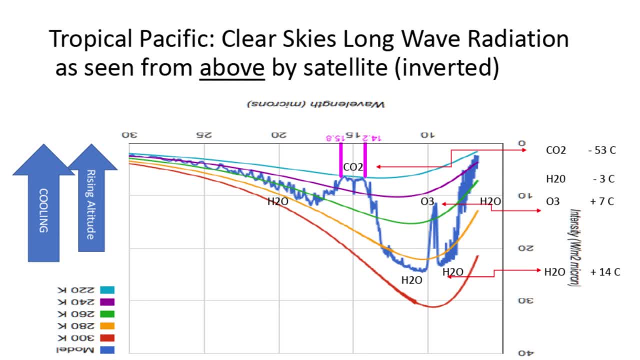 see how O3 and CO2 are and where they come from. These lines, the ones that were on the previous one, are now inverted here. These are the temperatures of the altitude or of the atmosphere as we rise in altitude and cool. So this is near the Earth's surface here at this temperature. This slide is actually of. 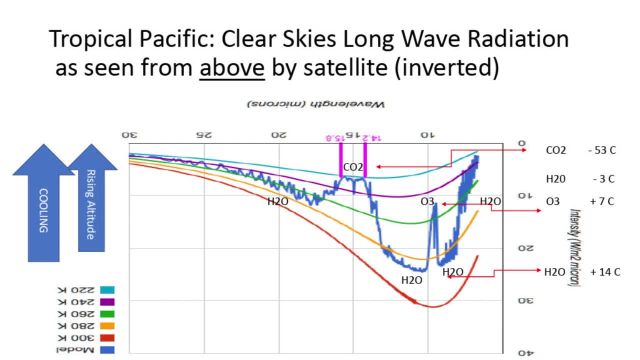 course, a spectrographic view, and so it's not a model, And what we're going to do is look at where we are. So CO2 at 15 microns is what we'll focus on first. That's in this area, right here. Now. what's happening is that it also is 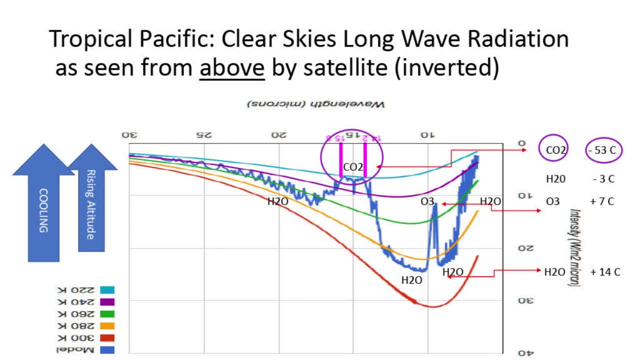 part of and equivalent to this particular area here, which is low temperature. We're at negative 53 degrees Celsius at the top of the troposphere. This is 18 kilometers above the tropical Pacific equator in this view, And the CO2 is a radiator of energy very high up in the atmosphere, but it's 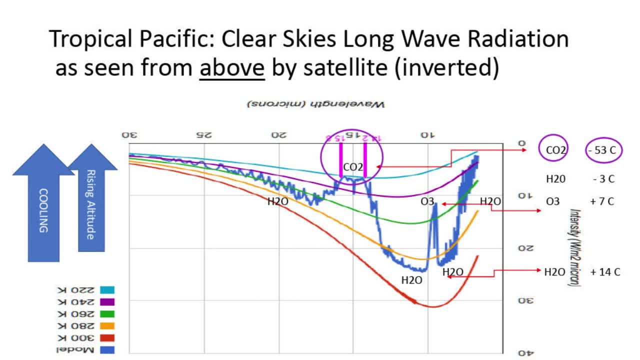 much less significant at all in the lower parts of the troposphere. We have no measurable effect below four to five kilometers. We've discussed that in terms of other reasons for that being in a different wave band, completely related to carbonic acid, But in this particular case we 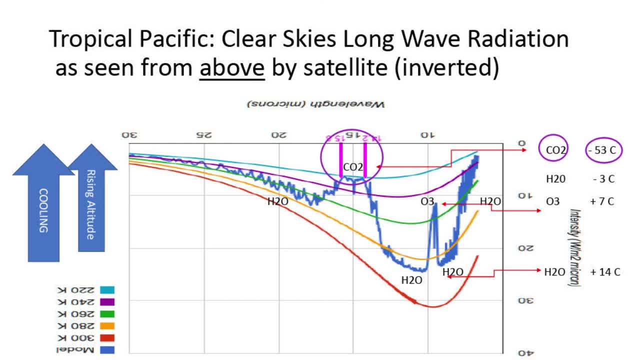 are getting CO2 and its effects showing up higher up The water and it's across the whole spectrum, at a negative three and negative three here, and also closer to ground at about plus 14.. So it dominates the whole spectrum, except for those other little peaks which are showing up. So it's 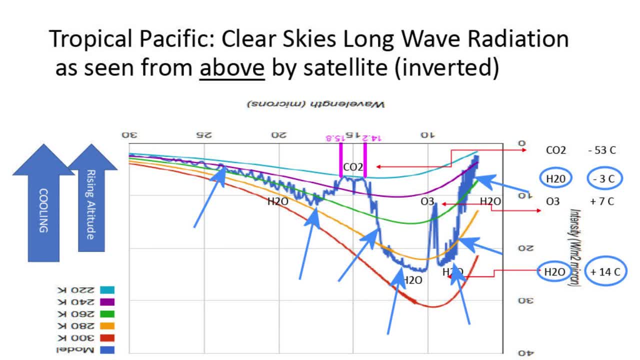 at a freezing level, at negative three, as you'd expect, And so that's where a lot of it is dropping out and not as very effective. The O3 is acting in the warm inversion zone of the stratosphere, which is at about plus seven higher up, where the warming from the creation of ozone in the upper 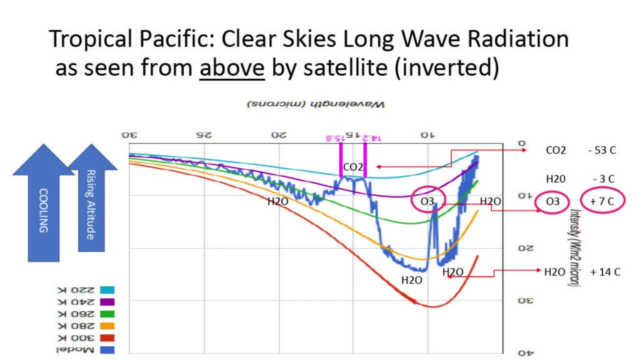 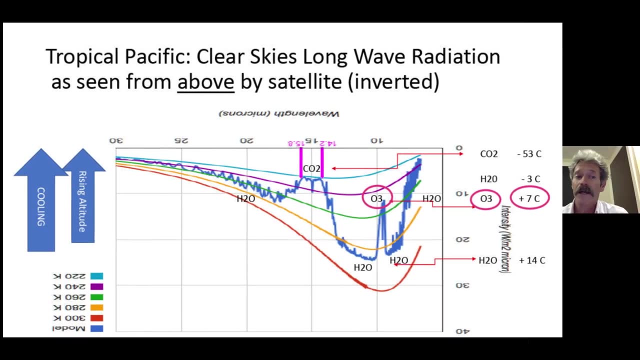 atmosphere takes place because of bombardment by ultraviolet light. So those are the reasons, but are we really clear on why and how CO2 or O3 really influence the ground level temperatures and our ground level conditions? This is a continuous column, but it isn't something that's clear. 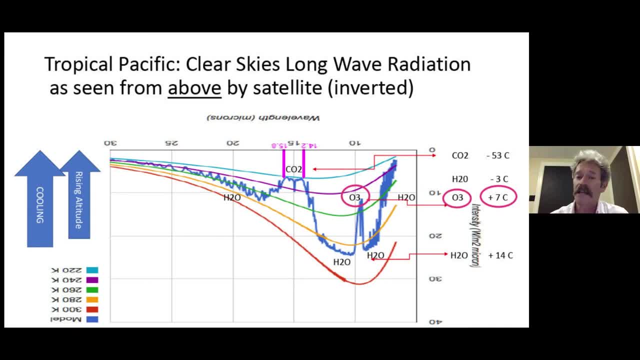 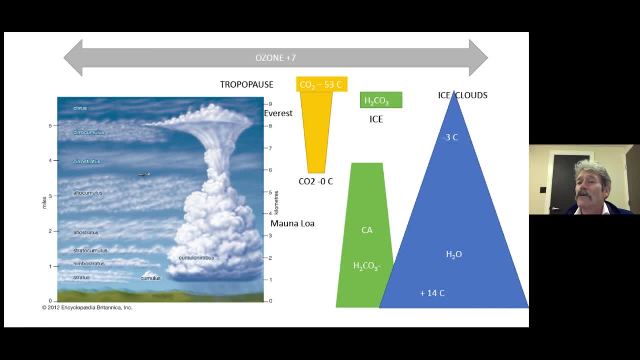 within a lot of the reasoning or people's understanding of how CO2 especially influences climate. So a profile view. you know CO2 does not act below six kilometers, So here's kind of a profile view of that. Here's Mauna Loa and here's Everest. Here's the CO2, maybe beginning its. 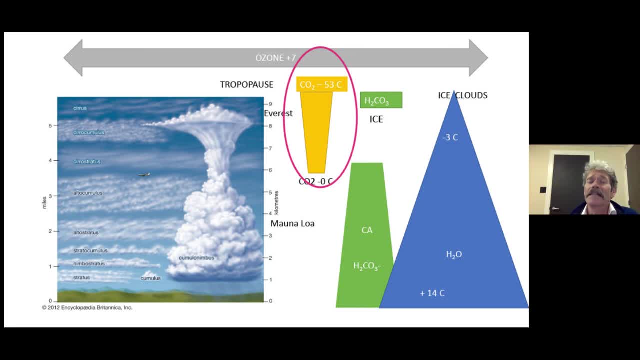 ability to act as a greenhouse gas in the upper atmosphere here, but dominantly looking at its biggest area way up high Negative 53 degrees C. These are the carbonic acid components. The ice of this nature is a speculation as to whether we also have carbonic acid ice. These are ice clouds, of course. 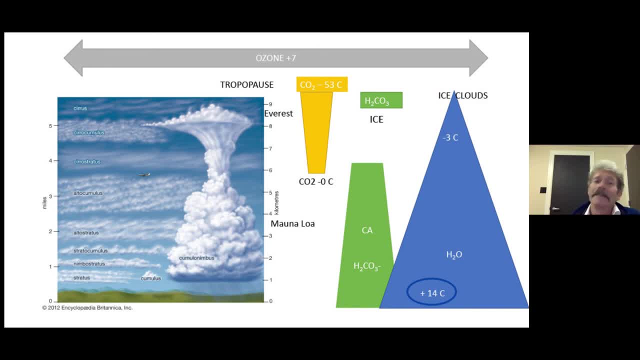 related to the water cycle, which goes from 14, we said- to negative three. The ozone. here it is sitting up anomalously at plus seven, Reheating, as you remember, because we have that thermal inversion: we cool down and then we heat up again. The only significant. 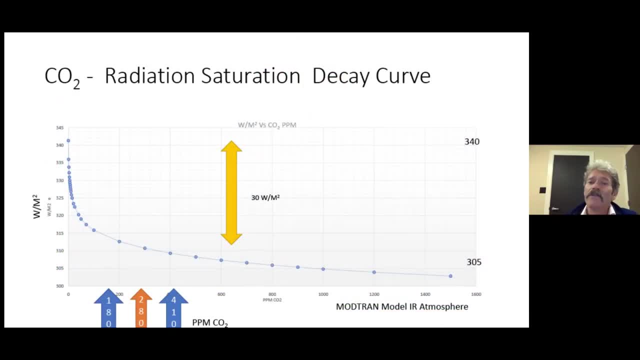 radiant power in theory attribute to CO2 comes in the first zero to 280 parts per million. over in here, moving from this point down to this point, Of the total theoretical power curve shown, 86% occurs in the first 280 parts per million. 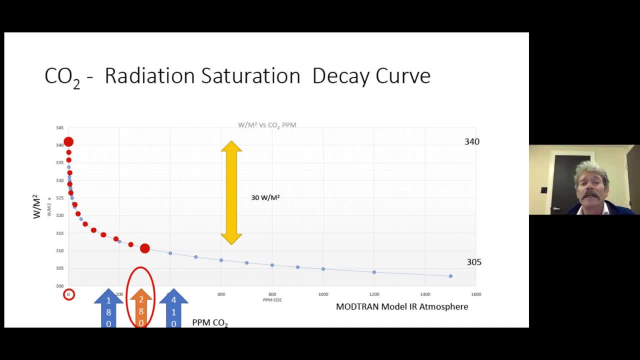 At times of glaciation. the CO2 in the ice core, if you remember, is sitting in about this area here at 180.. The real form of CO2 as carbonic acid in the lower atmosphere is not being shown in this model. The CO2 is involved as a pure gas. only here, Higher up in the atmosphere, is the place. 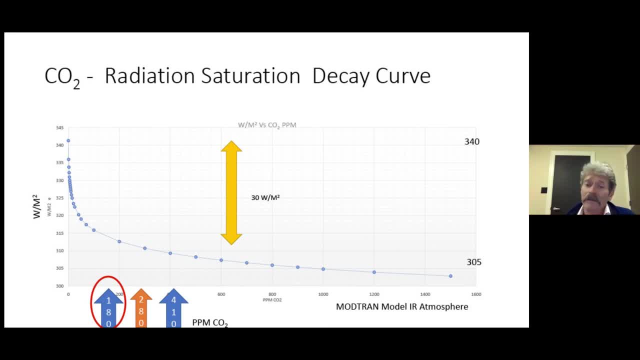 it can act. The PPM at that level should be thinner. This is a model built on PPM sliding across the top here: 800, 600, 400, 200.. Where is the CO2 going to be on a PPM basis in that upper? 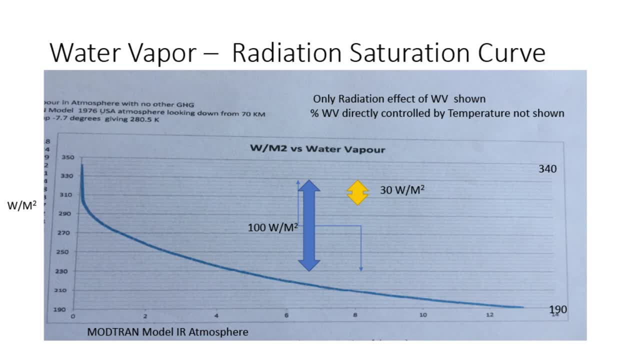 atmosphere And how will it influence? As with CO2 saturation in the previous slide, we see that water vapor also saturation, as shown in this Motran model as well, Comparing the two of them with CO2, theoretically, And this one is where water vapor is theoretically in this model. 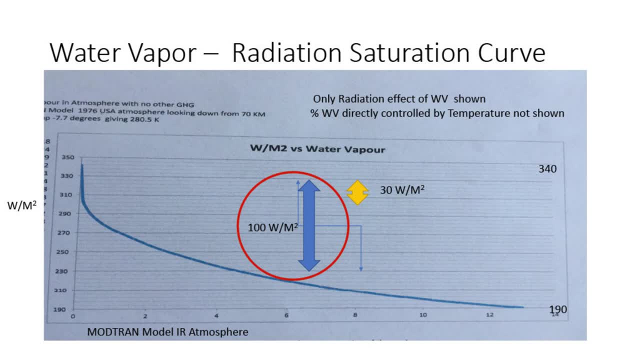 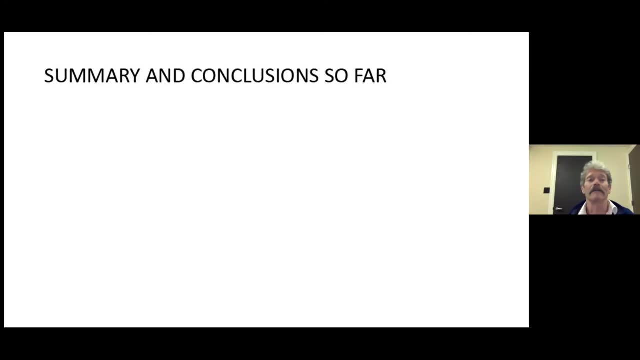 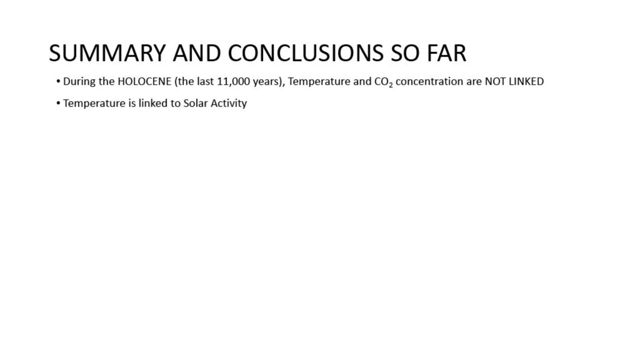 This is a factor of three to four times and certainly shows that water dominates. So I'd like to summarize: We've covered the Holocene the last 11,000 years. The temperature and the CO2 are not linked there. CO2 is not driving heating in the Holocene in any regard. 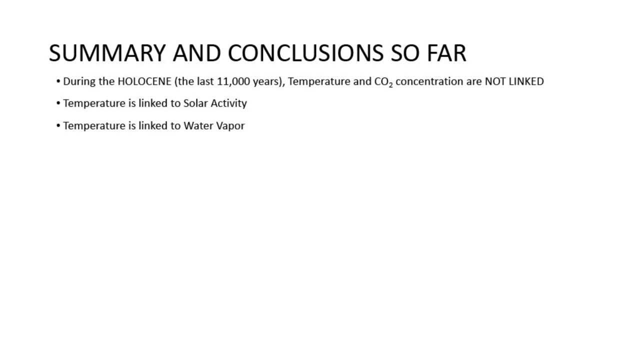 Solar activity is linked to temperature. Temperature is linked to ocean currents and water vapor. The ITCZ moves north or south seasonally and climatically with tilt of the earth. Models have large air limits. They poorly define the small energy imbalances. as a result, 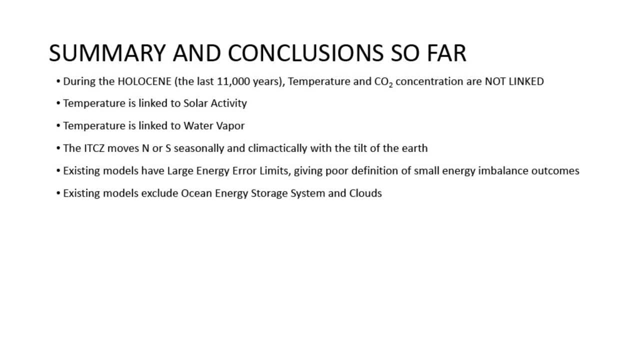 They exclude major areas of significant interest in climate analysis: The ocean energy storage system and clouds. Recent work in solar activity drives water vapor absorption. The solar activity is what seems to be driving our current water vapor, as we saw, and energy within the system.